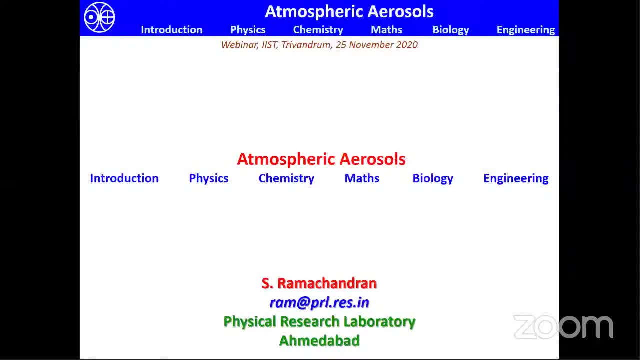 Modeling their impacts and radiation budget, atmospheric temperature and climate using radiative transfer and general circulation, and global climate models. He was a lead author of 2000 lead author of the 2007 climate science assessment of the intergovernmental panel on climate change, IPCC, which shared 2007 nobel peace prize. He is a reviewer and an author on the world. 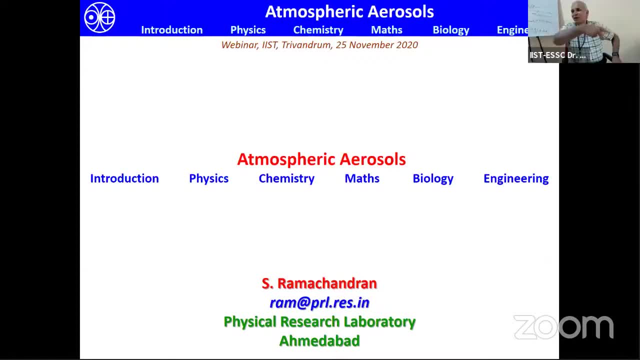 metallurgical organization WMO scientific assessment of ozone depletion. He was a senior fellow at the institute of advanced sustainability and studies, posdam, germany, in 2019.. He was a senior fellow at the nasa ams research center, california during 2008 and 2011-12 under the nasa postdoctoral 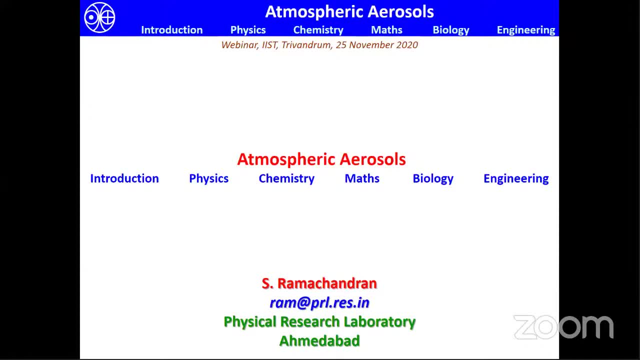 program. He is a recipient of the indian national science academy young scientist award in 1997 and also a member of the indian national science academy in 1997, and also a member of the indian national science academy in 1997, and also a member of the indian national science academy in. 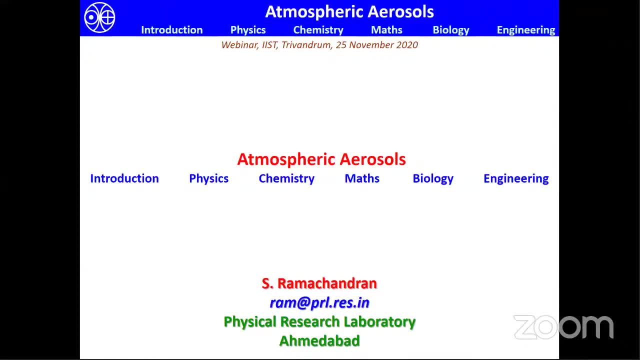 2007 and also the nasa group nasa group achievement award in 2000- 2009.. He has published about 100 research papers in peer-reviewed journals is recently he recently authored as a textbook entitled atmospheric aerosols characteristics and radiative effects and detail about professor. 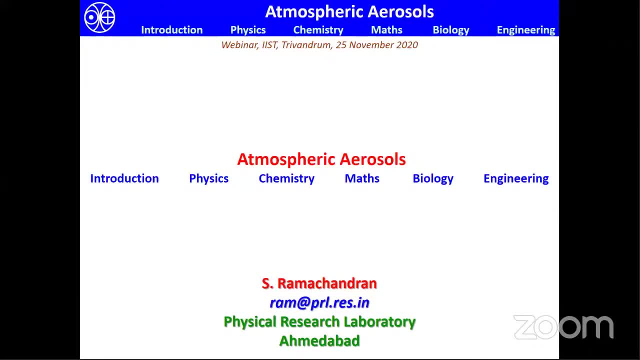 ram chandran can be obtained at his home page at pra. i request professor ram chandran to deliver his webinar. thank you, thank you, dr sinha. uh, dear friends, good afternoon. at the outset i like to thank professor chandra shaker and dr sinha for the invitation. 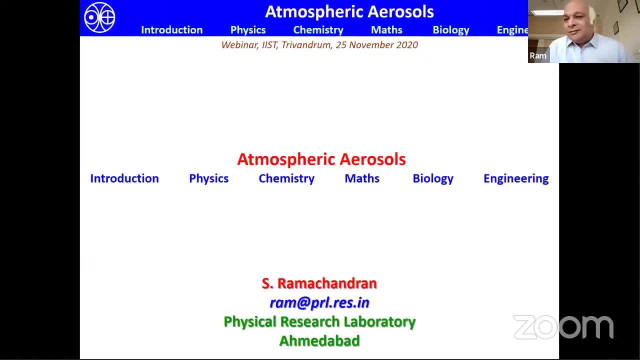 uh, while i accepted, uh the invitation with a little uh trepidation, because, uh, it was written to whom i will be addressing. so that actually posed a challenge to me, because normally you go deliver a talk based on your expertise and then try to come out of it when the job is a little easier. but 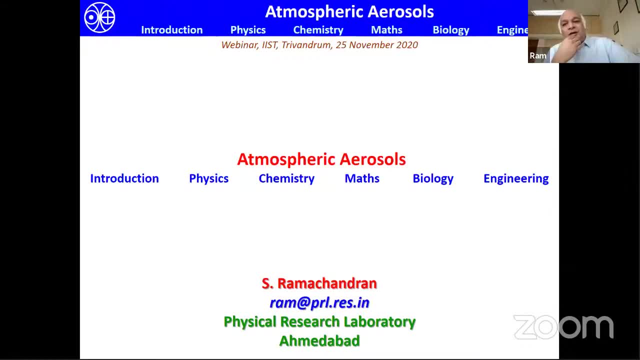 when, when the audience or the clientele is going to be of various times and some of the brightest minds in the indian engineering um force, which includes also sign science background people. so i set out a challenge for myself to kind of do the reverse engineering and then try to attract 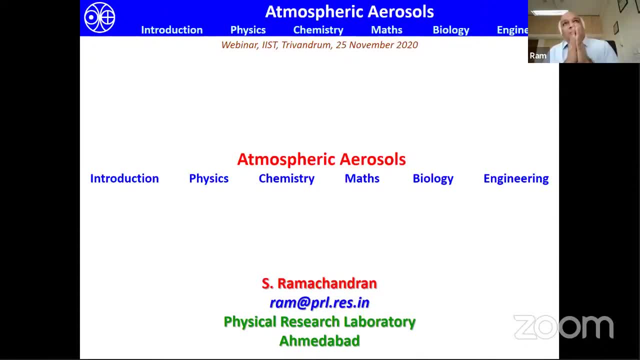 and then make you understand the various concepts of what we know on aerosols, which includes the physics, chemistry, max biology and the engineering aspects. so with these words let me begin the. so the presentation will go in in the following sequence: i will begin with an introduction and 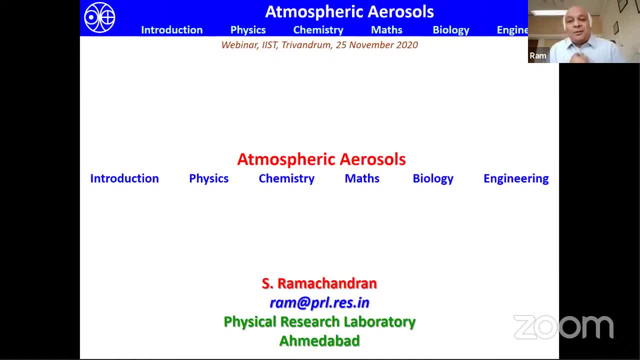 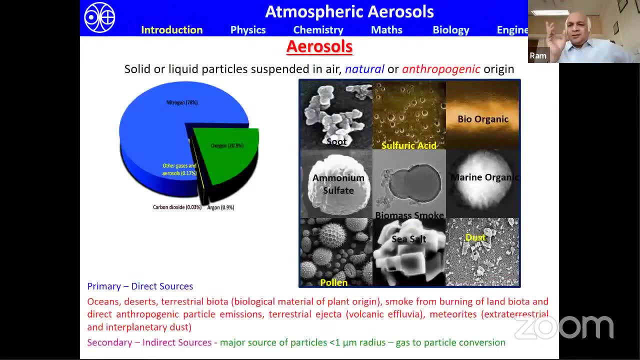 then i will discuss the various features under the pcmb and e and then, finally, we'll conclude the talk. so these aerosols, or air pollutants, as we know, are the solid or liquid particles that are suspended in the medium of air. they can be of natural and anthropogenic origin. 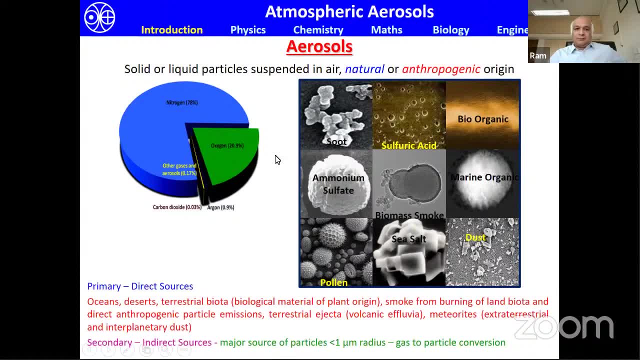 they are also very different in shape, and so i will give you a brief example of the way that these aerosols are suspended in air, so you can see that the sources are different, the shapes are different, the structures are different, etc. all the other species, all the other trace gases actually fight for each other. why? for their 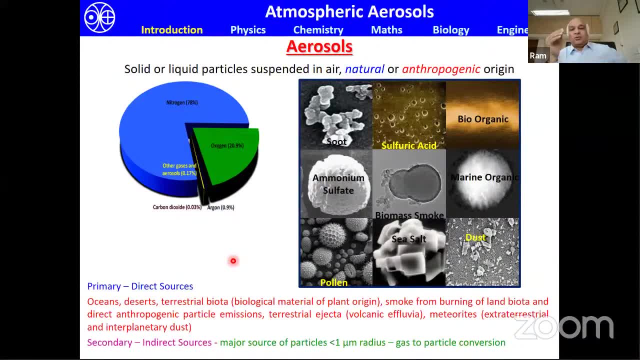 attention, starting from argon, carbon dioxide, ozone, trace gases and aerosols. you look at this. the percentage contribution to the total volume of the, the constituents in the earth's atmosphere by aerosols, is on the order of 4.1 percent or so, despite their very small contribution in the total. 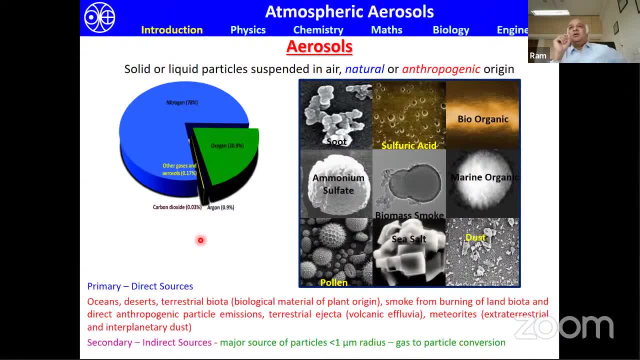 volume. they play a very important role in the physical, chemical process and the dynamical and radiative aspects of the earth's atmosphere system, as you will realize at the end of this seminar. so the sources of these particles are primary and secondary. the primary sources of the direct sources which have, which are oceans, desserts, terrestrial biota, meaning biological, 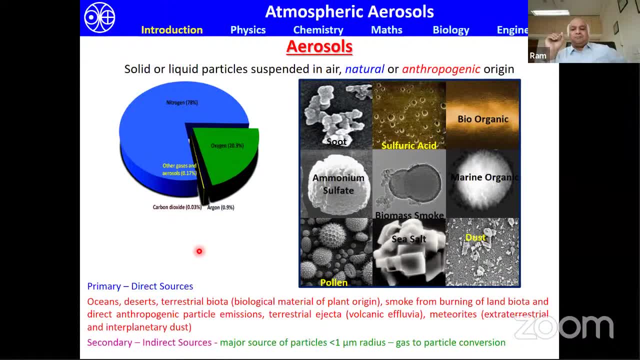 material of plant origin and the biological material of the earth's atmosphere and the smoke from burning of land, biota, direct anthropogenic particle emissions, terrestrial ejecta, which includes what the volcanic eruptions of the effluvia from volcano meteorites, the extraterrestrial and the interplanetary dust also form a part of the aerosol. 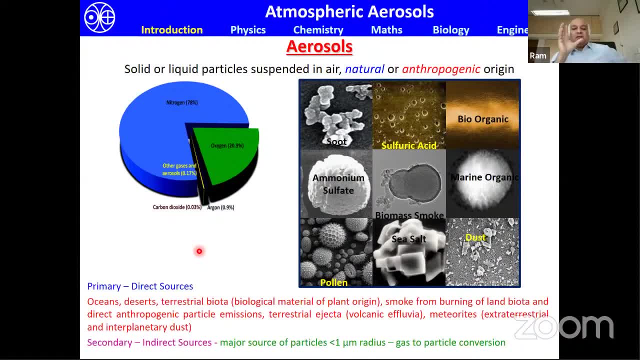 um. the secondary or the indirect sources are the the major source of particles for smaller in size, which also contribute to air pollution, which is mainly due to the gas to particle conversion mechanism. the precursor gases get converted into aerosols and then remain as aerosols in the atmosphere. 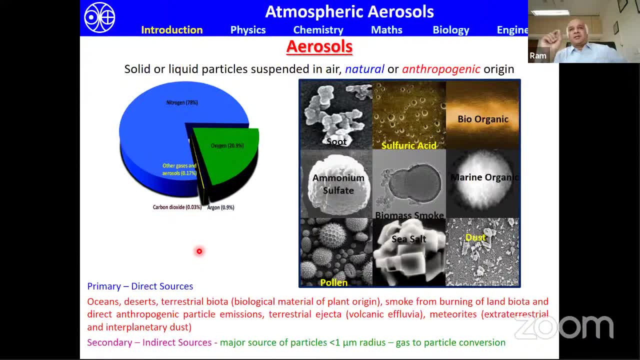 99.99 percent of aerosols or more are located in the 0 to 40 kilometer altitude of the earth's atmosphere. the, the extraterrestrial and the interplanetary dust content contribute to altitudes to aerosols above that. but as you, 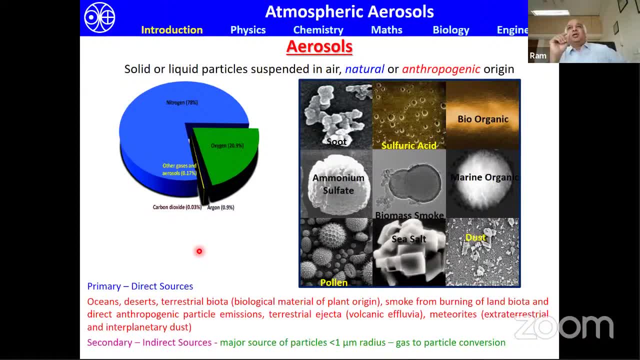 can see they form. they are a miniscule, very minuscule portion of the total aerosoles that is present in the Earth's atmosphere. and second thing, these emissions from the meteorites are extraterrestrial dust, or the interplanetary dust is kind of not systematic they are. they come in in 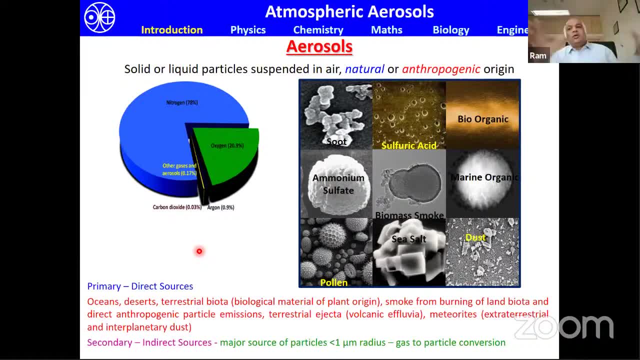 events, kind of an event, and so to the totalspec of the depletion, eated those particles than the apparently the most delicious долларов will become Escort and also, coming so far, economic zoo keen portion of the total glob remaining Day, and so that's the kit, and then water evenings that cleaned in this region하u. 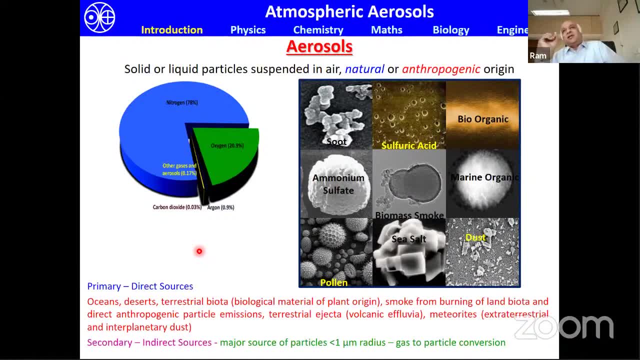 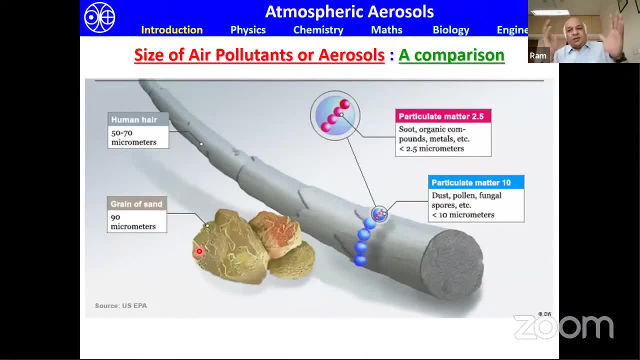 volume or the net volume of aerosols that is present always in the atmosphere. these are, like very, very, very, very small, so, um, so that you can appreciate the kind of concern, and what are we studying with respect to the aerosols and the air pollutants that we know? i have tried to compare. 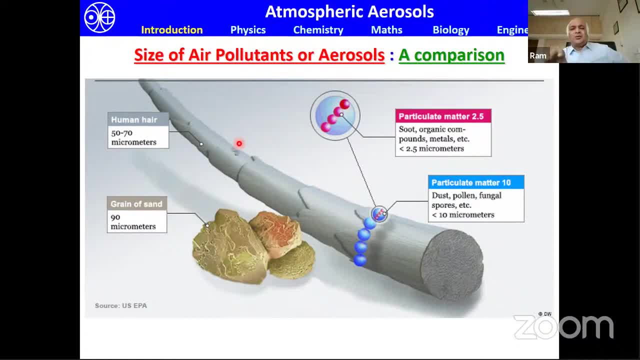 the particles that we call as aerosols, with the uh known species that we we are aware of. for example, human hair is part is shown here, typically a dimension of over 50 micrometer in diameter. when compared to that, the, even the dust and the other biological material are all. 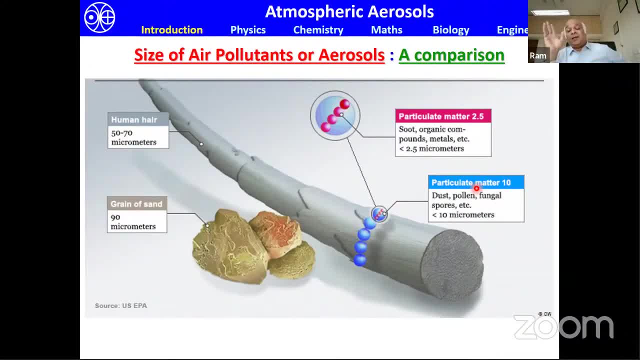 particles that are smaller than 10 micrometer and the particles such as soot, organic carbon, other metals, etc. they are even smaller than 2.5 micrometer. this is just to show the level of the, the size of the species and how they are playing an important role in the atmosphere. 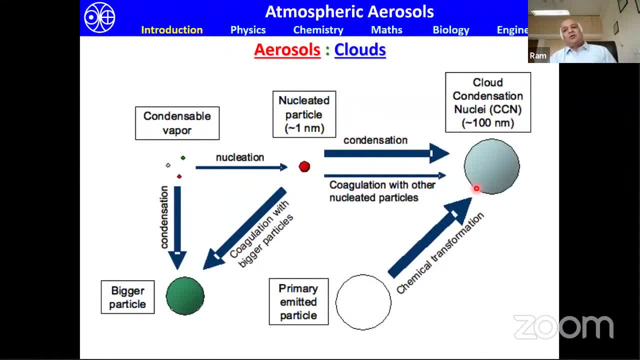 so these aerosols also serve as the cloud condensation nuclei- the smaller particles that are present, the content they can condense on the vapor, and then they form the nuclei to form bigger particles, which then finally turn into cloud condensation nuclei about 100 nanometer size. please note that 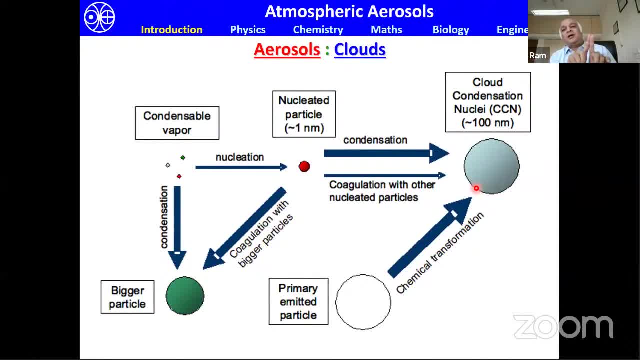 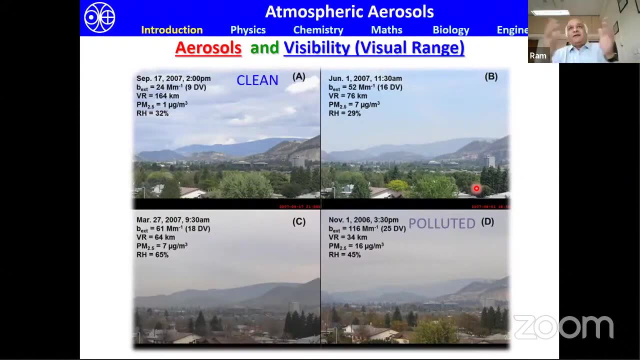 there will be no clouds if there are no aerosols in the atmosphere. so this is an important aspect of the earth's atmosphere, where aerosols serve as the cloud: condensation, nuclear, which includes sulfates, organics, etc. now, one aspect that manifests itself because of aerosols is is what is called as the visibility. 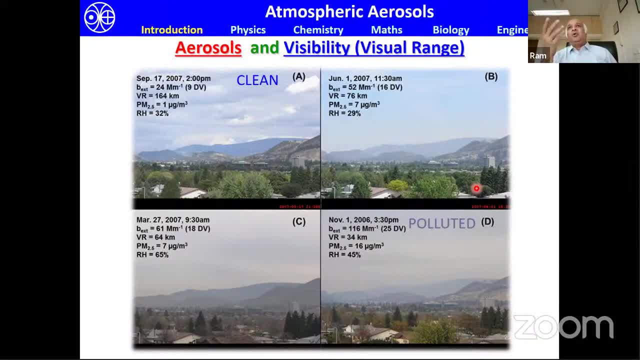 of the visual range. we know that when there is more pollution or dust in the atmosphere the visibility reduces. here i have just put it, put a figure here just to illustrate the difference between a cleaner environment and a polluted environment. so this is the kind of effect that it has on the 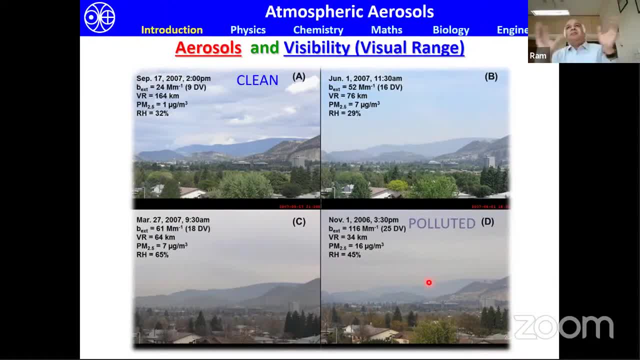 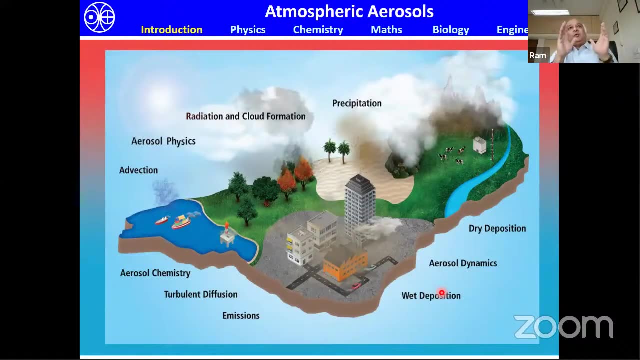 visibility. so this is a kind of a nearby manifestation of these particles when you are in a cleaner place with respect to a polluted place. so to sum up in the introduction, these aerosols are ubiquitous and omnipresent around us and is involved in almost all the processes that control the earth's climate, starting from 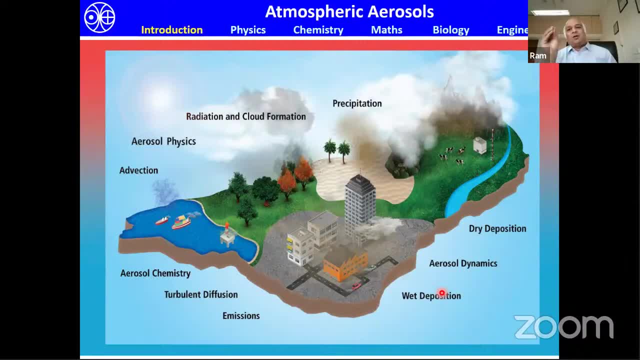 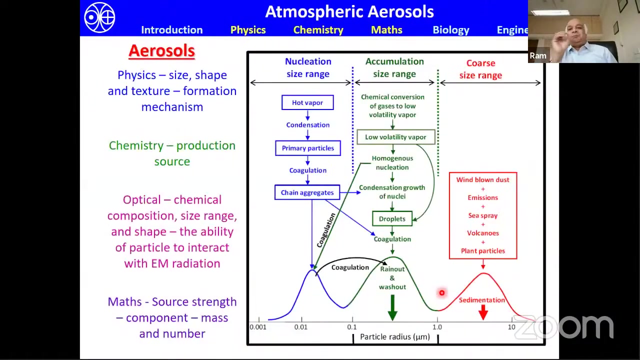 the balance, of affecting the balance of radiation, cloud formation, precipitation, emissions getting transported, the physics, chemistry and all of them. so each of this we will kind of look at it in some detail and kind of i will try to also demystify the, the myths surrounding these particles in the atmosphere, so the aerosols. we saw that they come. 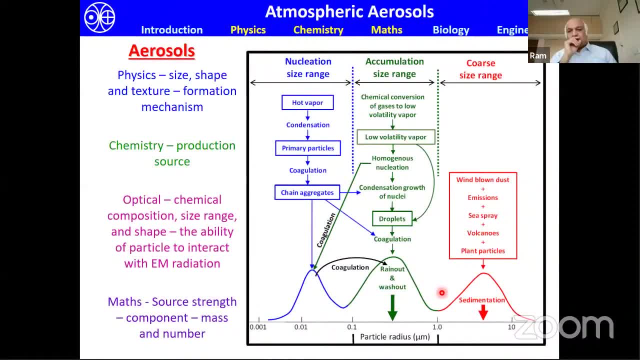 from different sources and they are of different sizes. here i have tried to plot as a function of radius, the, the type of particles that you can have in the nucleation size range, meaning particles that are less than 0.1 micrometer in diameter. so this is roughly 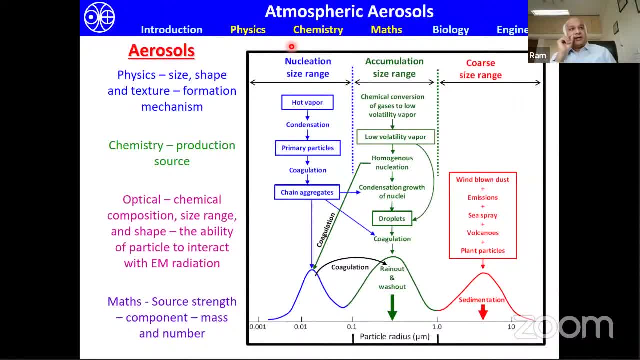 100th of 2.5 micrometer, kind of a scenario, one tenth, and then you have the accumulation size range, which is between 0.1 to 1 micrometer, and then the required size range where the particles are larger than 1 micrometer. so different processes take place in terms of the formation. 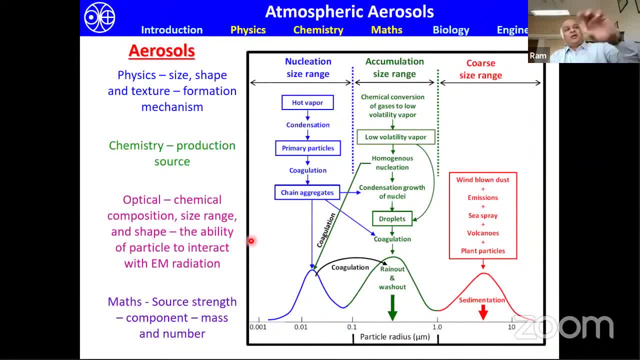 like i mentioned earlier, that when it forms the cloud condensation nuclei, it is the the vapor condensing on the smaller particles. they form a chain of aggregates and then form the aerosol particles in the nucleation size range, which then they chemically can convert into low volatility vapor or aerosols through. 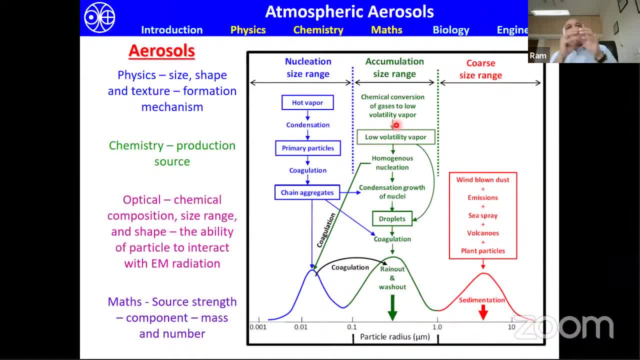 nuclear. so nucleation and also the condensation of growth. they can form a little bigger droplets than which are in the nucleation size range and then they are the main amount. they contribute, the main amount of particles in the accumulation size range. well, particles that are larger than one micrometer in the atmosphere are generated by mechanical 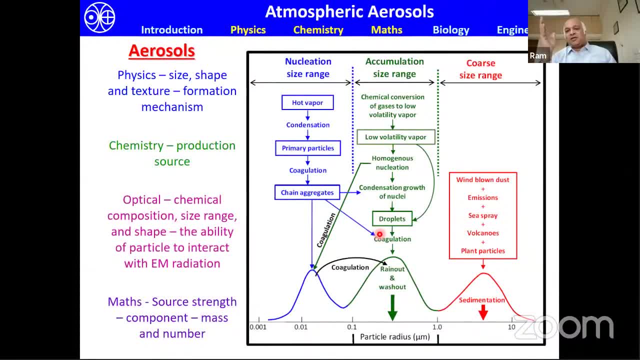 process, such as windblown dust, sea, salt sea spray emissions, volcanoes, plant particles, etc. all of them we'll see in detail as the top progresses. so when i mentioned that the, it involves all the aspects of science and also engineering, so i meant this one. so the size shape. 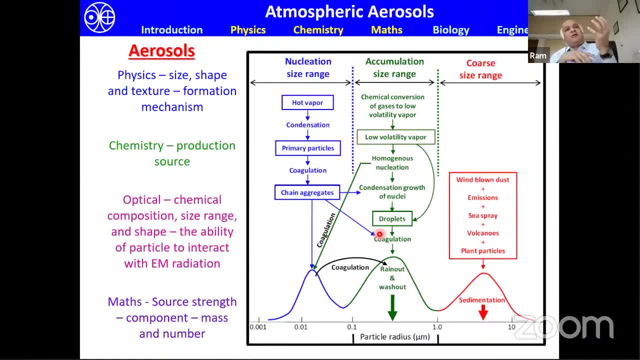 and the structure of these particles. they vary. the formation mechanism determines the physical characteristics, while the production source- whether it is coming from a vehicular emission versus a volcano, versus a windblown mineral dust- that determines the chemical composition of the species, then both of these combined. 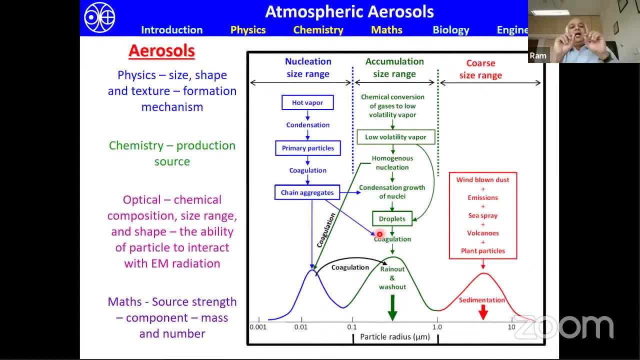 The composition, size range and the shape decide the ability of each particle to interact with the electromagnetic radiation that is coming from the sun and also going back from the Earth's atmosphere, so directly contributing to climate and the radiation. And we need mags in order to determine the source strength of each of these components in the Earth's atmosphere, which is decided by the mass of these particles and also the number of these particles as a function of size. 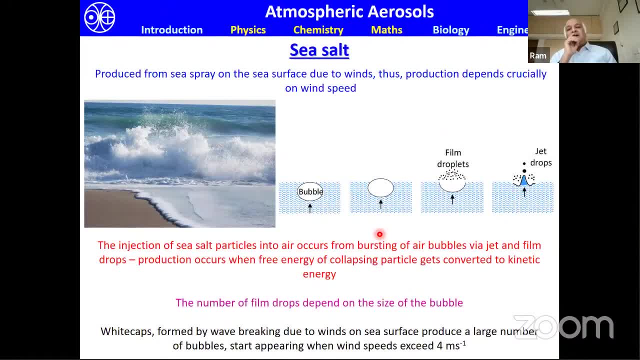 So, starting from sea salt, I'm sure I don't need to tell my friends in Shemangram that have you seen sea salt or sea spray? They will. They will kind of look at me. So the sea salt is produced from sea spray on the sea surface due to winds. 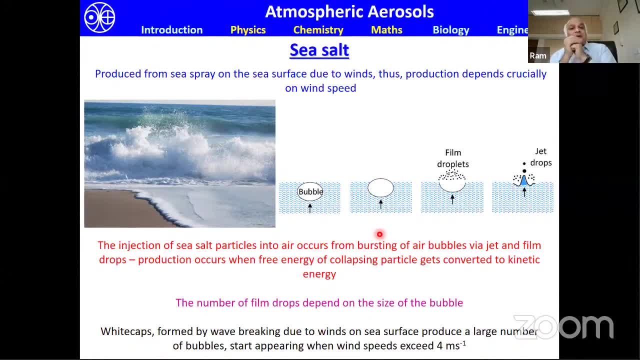 Thus, the production of these particles depends on the wind speed. Typically, the injection of sea salt particles into the atmosphere occurs from bursting of air bubbles via jet and film drops. This production of these particles occur when free energy of the collapsing particle gets converted into kinetic energy. 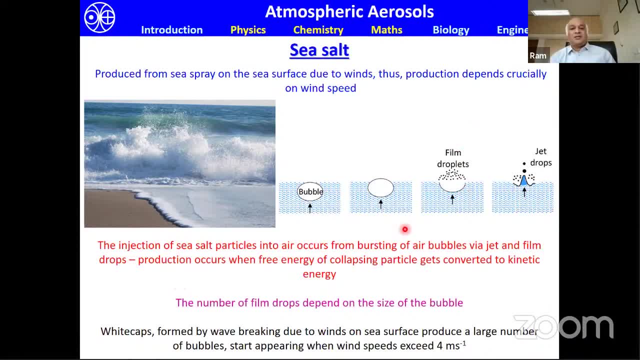 The number of film drops that come out of this depend on the size of the bubble. The bigger the bubble, the more the number of film drops. So usually, when the wind speeds exceed more than four to five meters per second, you see on the ocean surface a kind of a white layer, which we call as the white caps, which are formed by wind breaking due to winds on sea surface. 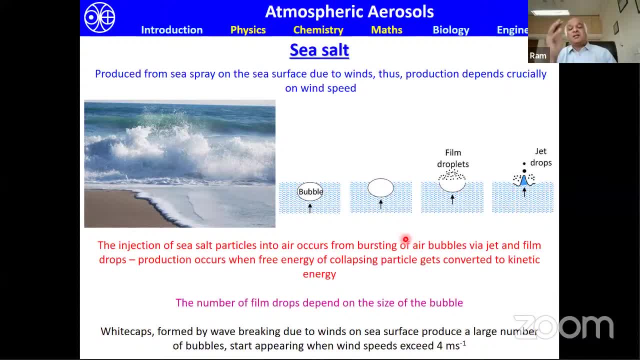 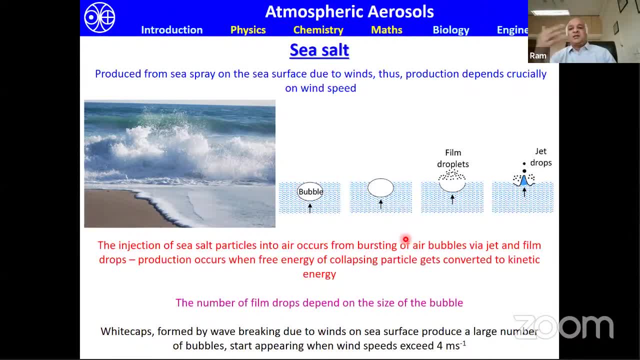 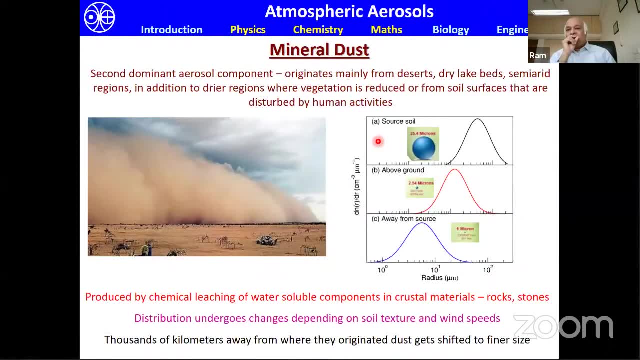 So the sea salt is released. So the sea salt is released. The wind speeds exceed about four meters per second. So this is how the sea salt particles in the atmosphere are produced. The second dominant aerosol component, namely mineral dust. they originate from deserts, dry lake beds, semi-arid regions, in addition to drier regions where the vegetation is reduced from soil surfaces that are disturbed by the human activities. 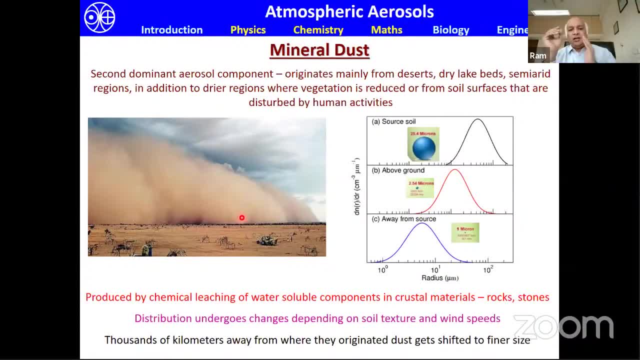 So The dust particles are essentially produced by chemical leaching of water-soluble components on crustal materials such as rocks and stones, Where they are produced, and because these get transported. like you can see from the figure on the left hand side, the distribution goes on changing depending on the soil texture and the wind speeds. 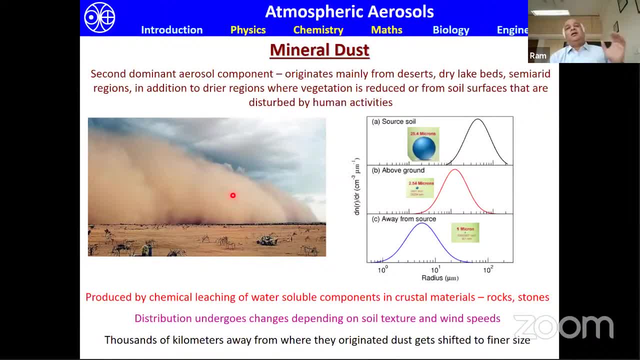 Thousands of kilometers away where they originated, the dust particles get shifted to smaller sizes. So here to give an idea of what we are talking about in terms of the size near the source of soil. where suppose, if I am allowed to measure the dust here? 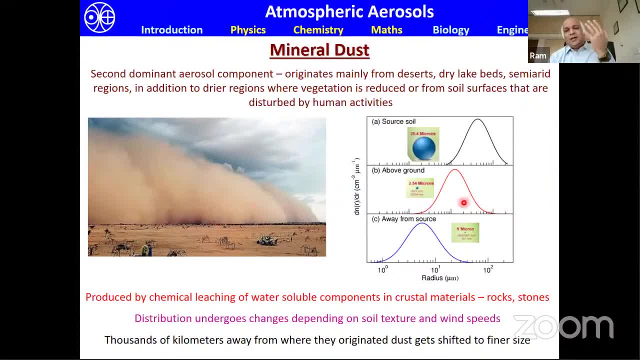 the size will be about 25 micrometer and then a little above ground, a little farther. then you can see the size that is getting reduced and regions thousands of kilometers away. they can be very, very. it depends on how high the dust particles are. 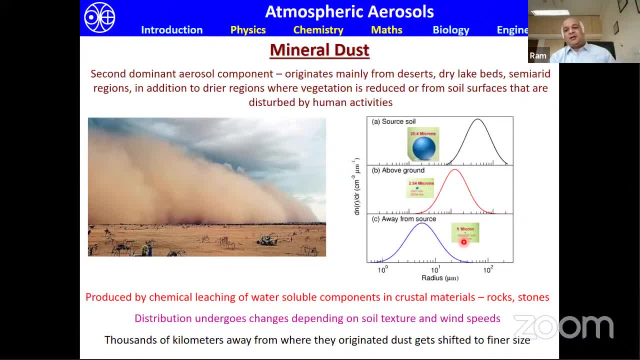 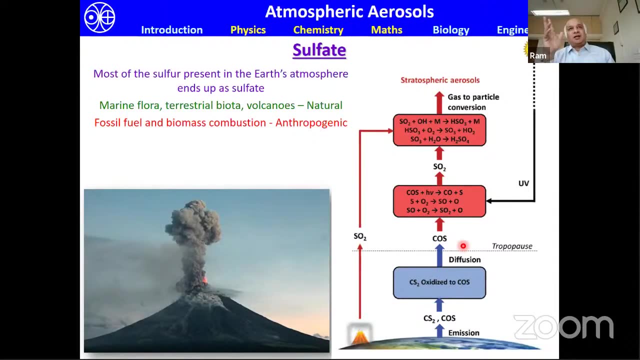 what is the wind speed, what is the texture of the dust material, etc. So you can see particles that are very small at thousands of kilometers away from the desert regions. Then the other major aerosol component in the Earth's atmosphere is the sulphate. 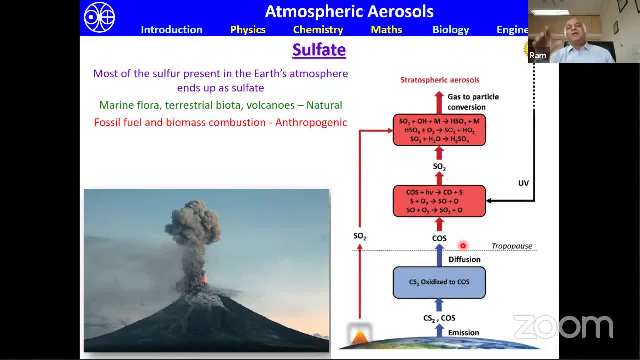 All the sulphur that is present in the Earth's atmosphere ends up as sulphate. as it is the thermodynamically stable form of sulphur, It interacts with oxygen and then forms the sulphate, Out of which the marine flora and the terrestrial biota are the major biological sources of sulphate aerosols. 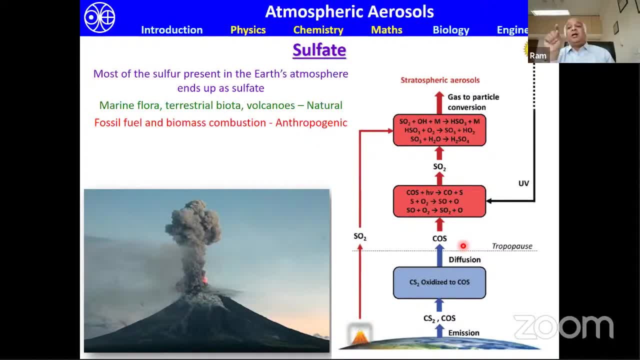 meaning dimethyl sulphide and other compounds. The only non-biological source of sulphate in the atmosphere comes from volcanoes. And these are all the natural sources, While the fossil fuel and the biomass combustion of the biofuel burning, which is anthropogenic in nature. 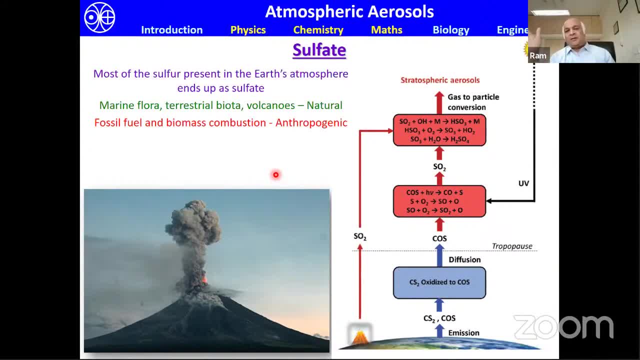 they inject a large amount of sulphur dioxide and then sulphate particles, So typically the sulphur dioxide that is emitted in other species, such as carbon, disulfide, etc. they get oxidated to carbon and sulphide SO2 can get directly converted into sulphate. 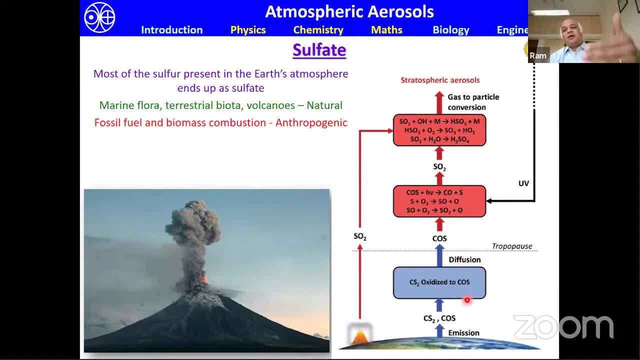 while carbon disulfide and carbon and sulphide. they get converted into sulphur dioxide first, and then they become sulphate aerosols. This is a schematic of aerosols that is found in the troposphere and in the stratosphere of sulphate. 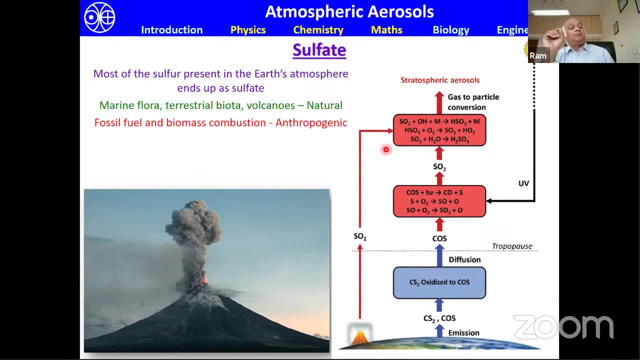 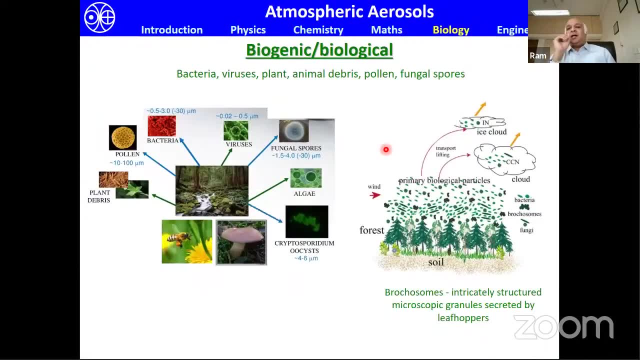 And this process occurs through gastroparticle combustion mechanism, which we saw earlier. Now the other natural component that is present of aerosols in the atmosphere is of biogenic or biological origin, where the bacteria, viruses, plant and animal debris, pollen, fungal spores, etc. 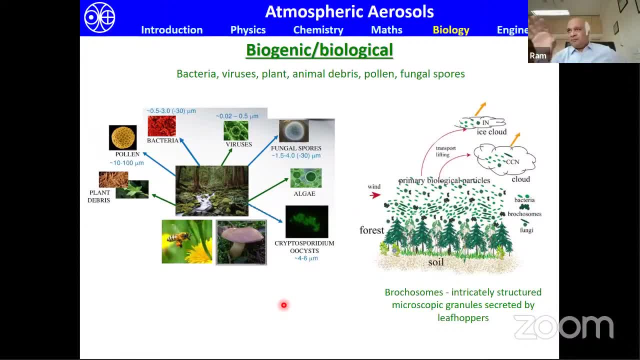 they also contribute to the aerosol that is present in the Earth's atmosphere. I have shown here an illustration of the typical sizes of pollen grains versus the other species of interest, So typically the forest regions and the soils. from there they emit a large amount of these biological particles. 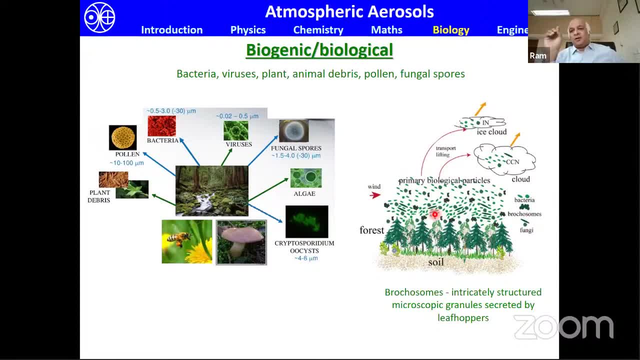 which also play a role in the cloud condensation process that we talked about earlier, And then they also get transported across, depending on the wind speed, the conditions that are favorable, etc. So you see, on the right hand side, a word called brocosomes. 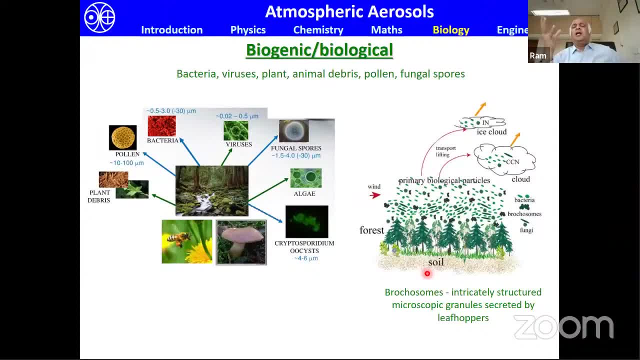 These are intricately structured, microscopic granules that are secreted by a species called leafhoppers. These are also aerosols practically suspended in air. Liquid or solid is what we call as the aerosol. However, when it comes to the radiative aspects and the climate aspects, etc. 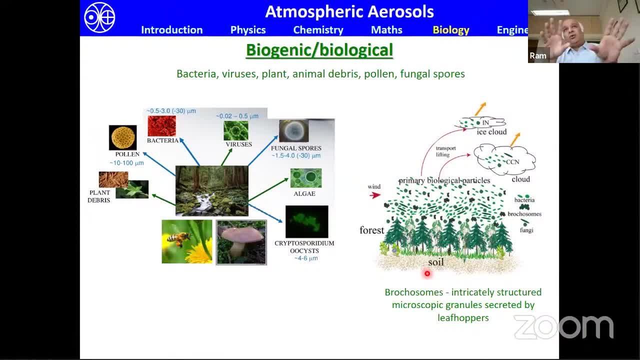 the biological aerosols have their own role in terms of the climate change, etc. which we will touch later. But when it comes directly to radiative effects on climate, the other aerosol species that we talked about earlier or the aerosols from the different sources, 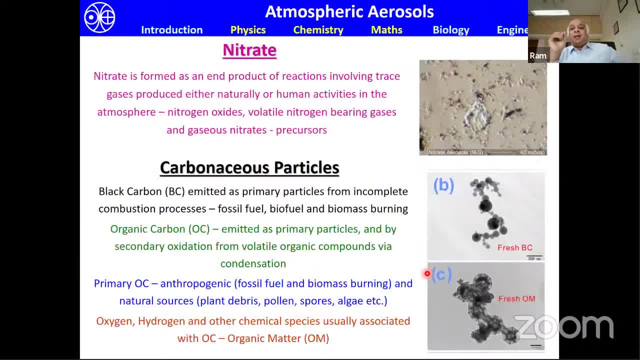 they contribute to those effects. The other major species of aerosol is the nitrate. This nitrate is formed as an end product of reactions involving trace gases produced either naturally or by human activities in the atmosphere, typically nitrogen oxides, volatile nitrogen-bearing gases. 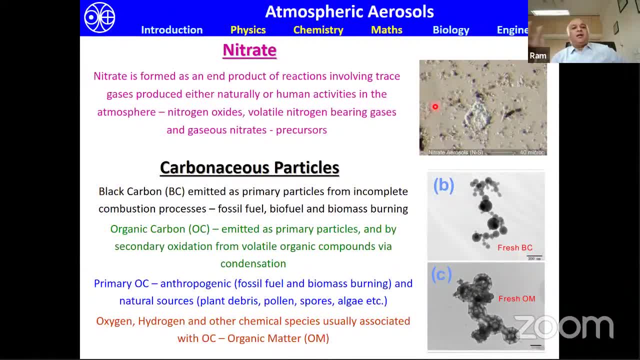 and gaseous nitrates, which are precursors for the nitrate to be formed, which are both of natural and anthropogenic origin. The vegetation and the soil and the fertilizers that are used they inject a large amount of these nitrogen oxides. 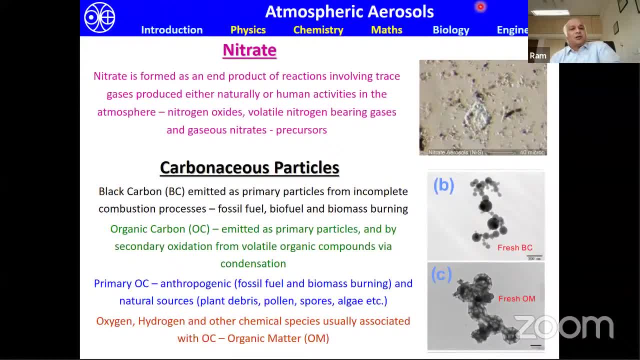 and the vehicular and industrial emissions also inject a large amount of nitrogen oxides and volatile nitrogen-bearing gases. The other species that is gaining interest in the recent decades are the carbonaceous particles, which are of two types: One is the black carbon and the other is organic carbon. 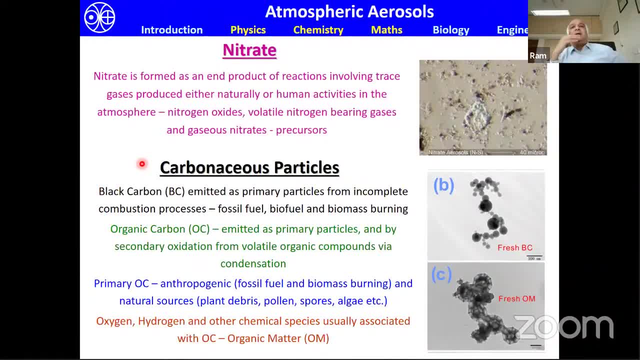 Black carbon is emitted as primary particles from incomplete combustion processes such as fossil fuel, biofuel and biomass. burning Organic carbon is emitted as both primary particle and by secondary oxidation from volatile organic compounds which may have their biological origin via condensation. 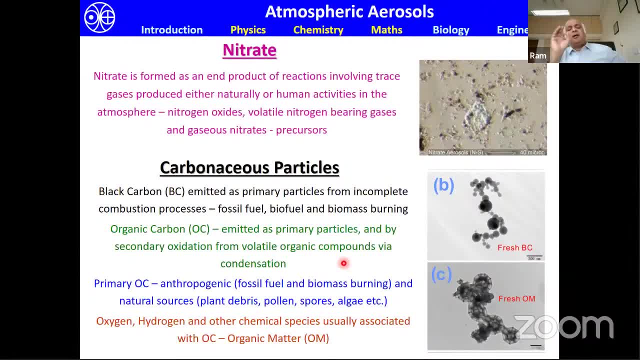 Now the primary anthropogenic, primary organic carbon comes from the anthropogenic, namely fossil fuel and biomass, and also from the natural sources, namely plant debris, pollen, spores, algae, etc. Typically oxygen and hydrogen and other chemical species. 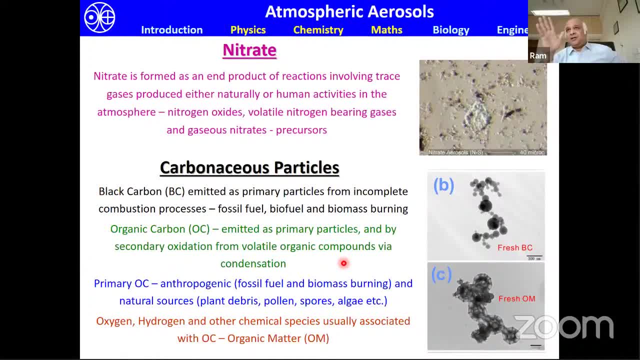 are usually associated with the organic carbon that is present in the Earth's atmosphere and we, in total, we call them as organic matter. As opposed to all the other species in the Earth's atmosphere, there are no known natural sources of black carbon. 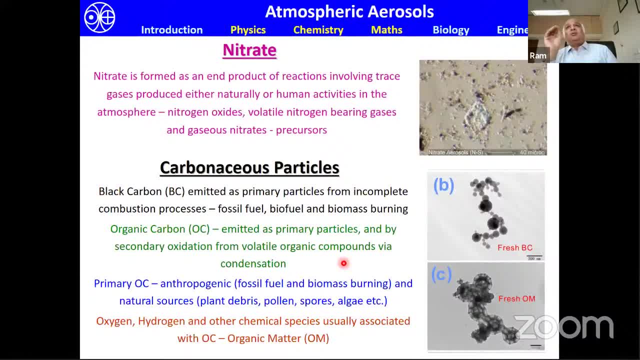 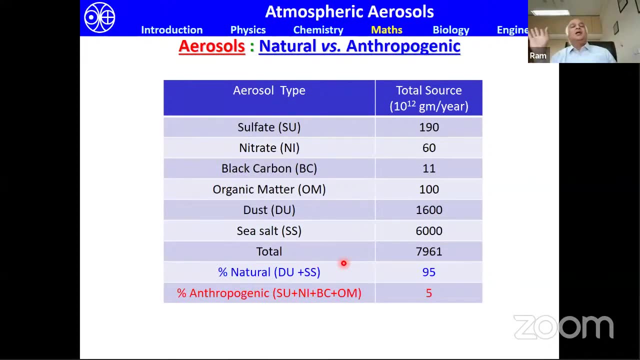 in the Earth's atmosphere. So almost all of them that is present, black carbon in the atmosphere- is actually human produced. So if I'm allowed to look at the break up the budget and see that, how much is natural, how much is manmade in terms of the aerosol loading. 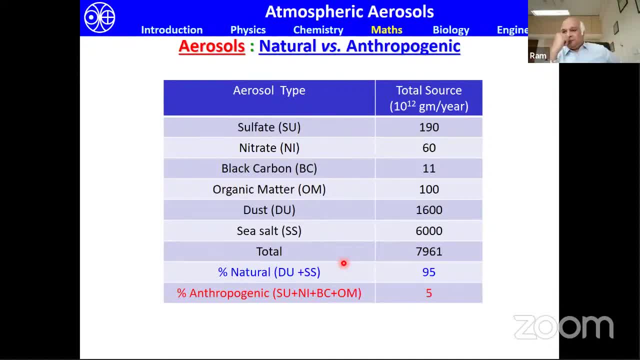 or the source that is over the Earth's atmosphere. then we put it in terms of 10 to the power of 12 grams per year. This is the source, the amount of emissions per year, and then we try to put the numbers based on various other estimates and model studies. 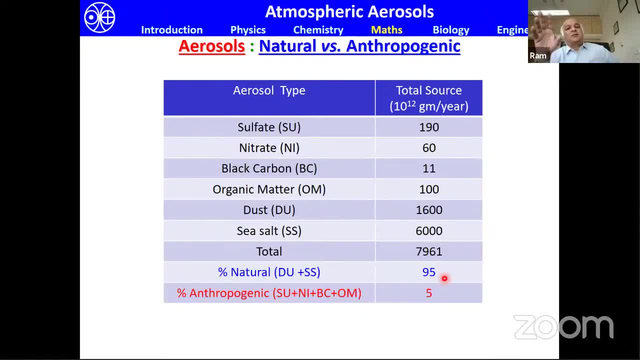 and we try to categorize them as natural- versus anthropogenic. The natural, which I have categorized as dust and sea salt. they contribute more than 90%, while the manmade contribution is only about 5% or so in the total volume of aerosol that is present in the atmosphere. 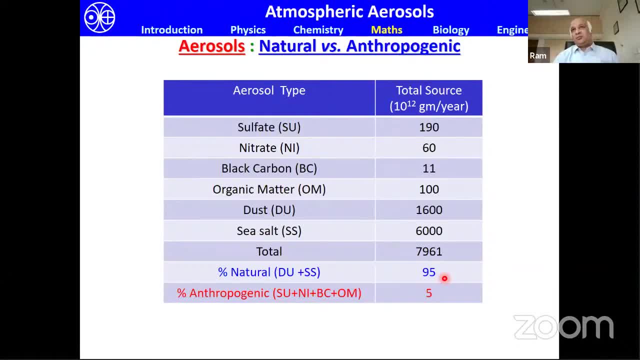 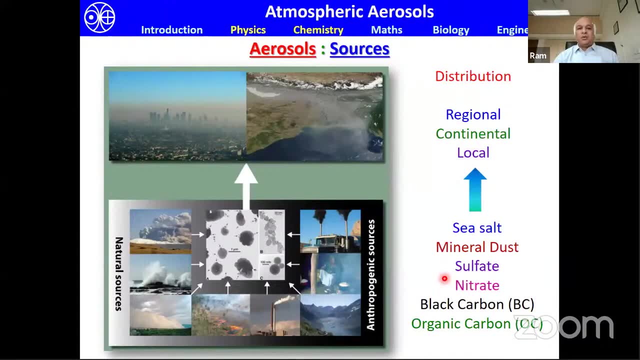 But the whole scenario, you will see, change will change when we are talking about the radiative and the climate aspects. So these aerosols, which are produced from different sources and can be categorized as sea salt, mineral dust, sulfate nitrate, black carbon and organic carbon. 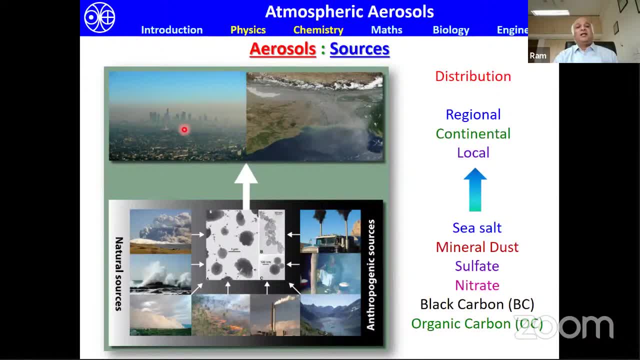 they can. they produce a kind of a hazy atmosphere which is clear, and also there's a familiar picture across the Indo-Gazette which has declined during the winter timeframe and there is a lot of these aerosols get transported across. 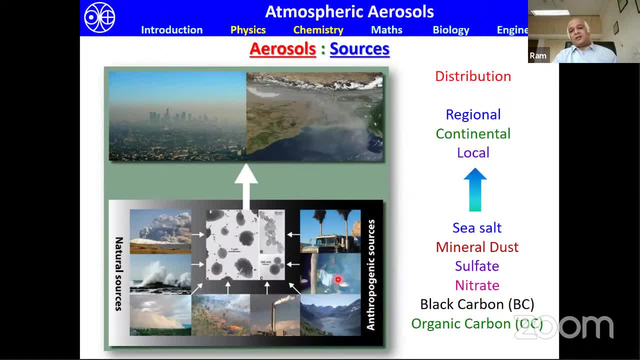 And from all these, both natural and anthropogenic sources. you also notice that when I am classifying them as natural versus anthropogenic aerosols, the natural aerosols are more whitish when compared to the anthropogenic sources, which are blacker. 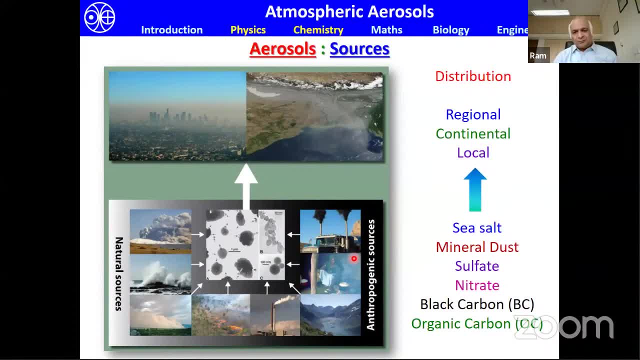 the importance of which will come in the next few slides. Keep that in. keep this in mind. So these aerosols that are produced from different sources can produce local, continental, regional and global distributions and hence can contribute to global effects. 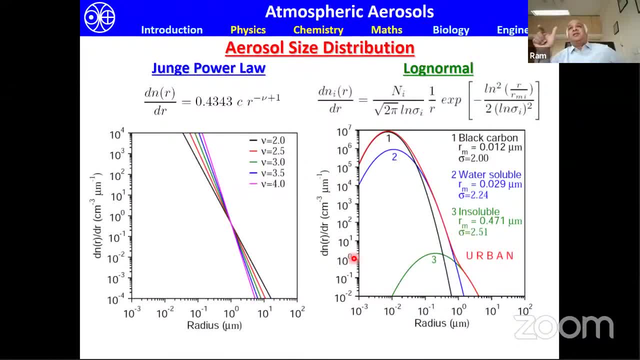 So when physics and chemistry came in, Max, how can it be far behind? So Jungge was the Christian. Jungge was the first scientist who found that, in order to represent the aerosols of different sizes, you need what you call a size distribution function. 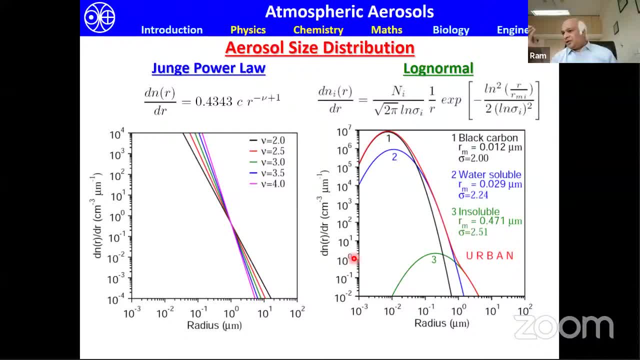 and an expression to derive or to measure the size distribution function. Because this became important? because, unlike the air molecules, which is of one size, where aerosols are of several magnitudes, they are different, sweeping from a cluster of molecules at one end to hailstones at the other end. 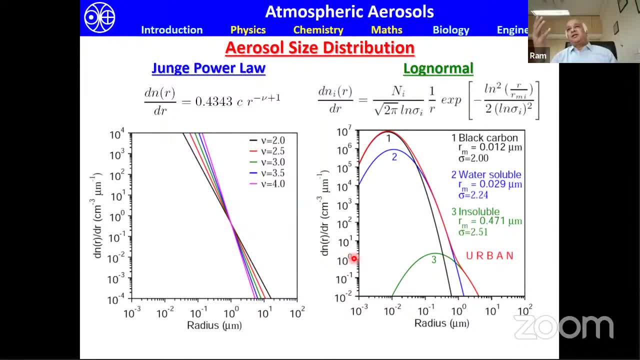 So you need to have a measure, a mathematical measure to show, illustrate how the particle numbers vary as a function of size. So Jungge thought of an easy way to come out of this. He simply said: okay, the number of particles that are present. 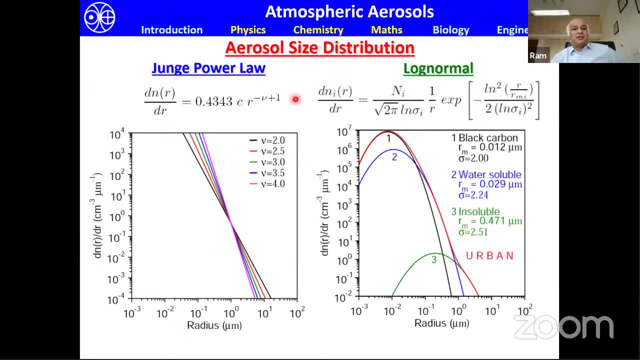 should be proportional to a parameter which is called as the size distribution function, which is given as mu here, And depending on its variation, the number of smaller or the larger particles will be different in the atmosphere. Now one of the major drawbacks in this distribution: 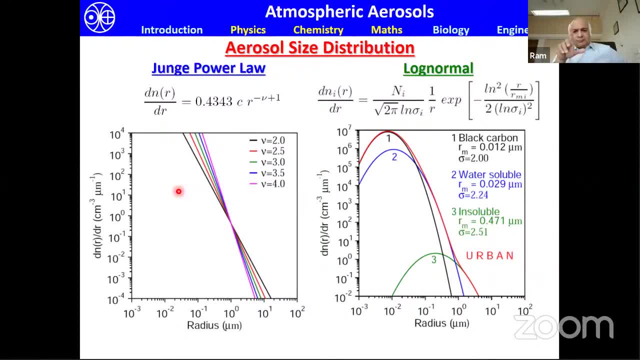 is that the this may be applicable to kind of one type of species, one type of particle, namely sulphate nitrate or black carbon or something, But when the atmosphere, which has all the components that represent together, then it becomes difficult to categorize this. 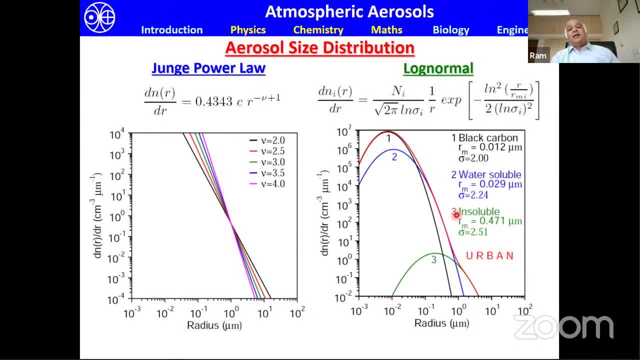 using this size distribution. So then came what is called as the log normal or the normal distribution with the log attached to it. So this one has the ability to decipher or delineate the contribution from each of the different types that contribute to the population. 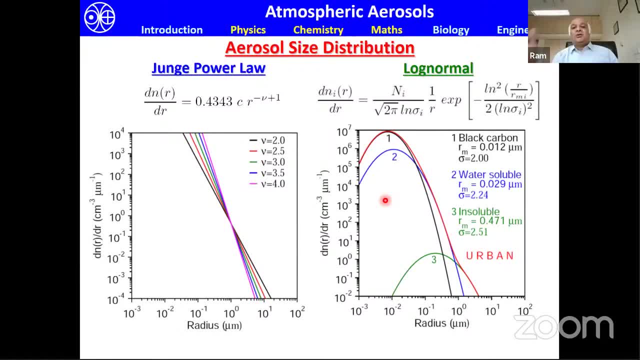 that are present in the particular region. So here what we are seeing is an aerosol distribution or an urban region which is primarily made up of three components, namely the insoluble species, certain amount of organics and dust. 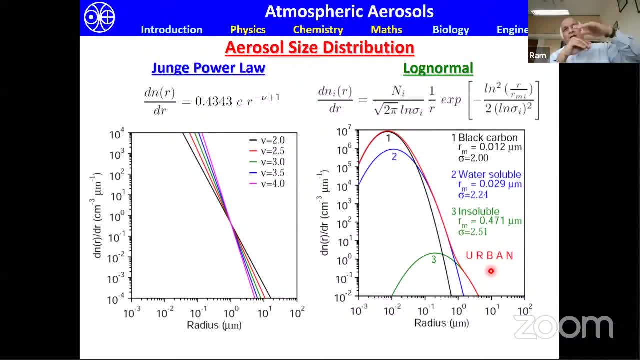 soil, dust, particles. Water soluble is sulphate nitrate, etc. organics, etc. And black carbon is the human influenced or human emissions of black carbon from industrial and vehicular emissions. So each of these components, I have named it as one, two, three. 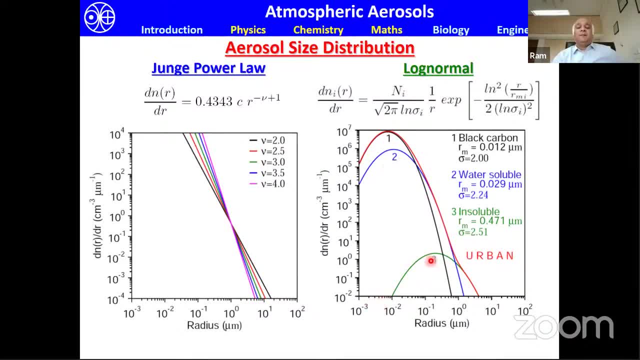 and the total is given in red. They all have a distribution with the different values wherein they actually peak and they contribute to the total. So this is a kind of a more realistic way of representing the aerosol distribution which arises due to aerosols of different sizes. 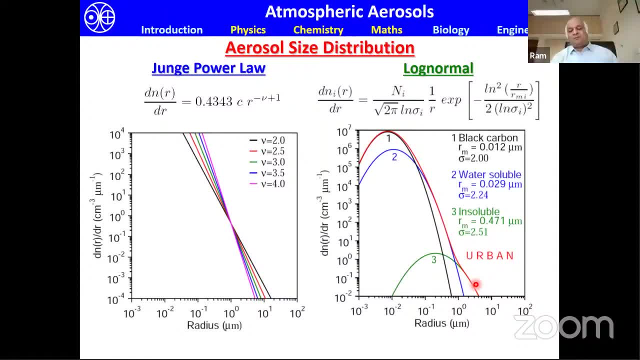 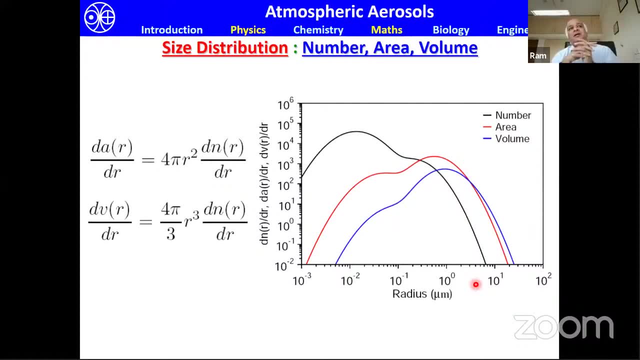 that are present in the atmosphere and in different numbers. It is not the same, but the numbers are also different. So you can equally represent the number that is measured or derived into area and volume by multiplying spherical 4 pi r square and 4 pi by 3 r cube. 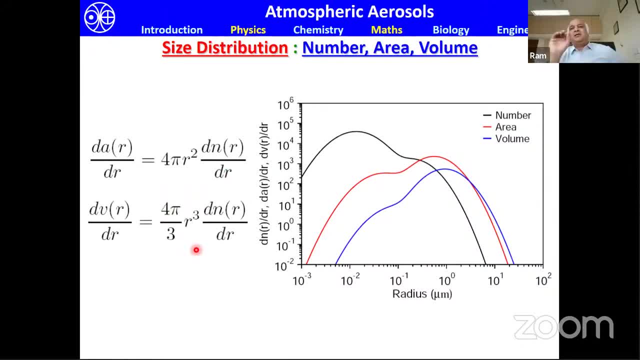 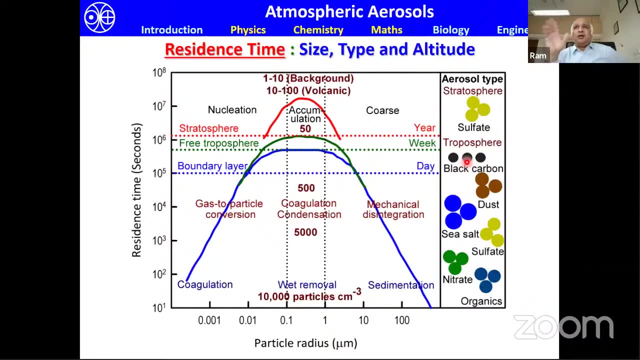 So, depending on the r square, r dependence, the peak at which the distribution peaks also will differ, because the area is r square and volume is r cube. as you are aware, The aerosols that are produced by different processes and the different sizes. 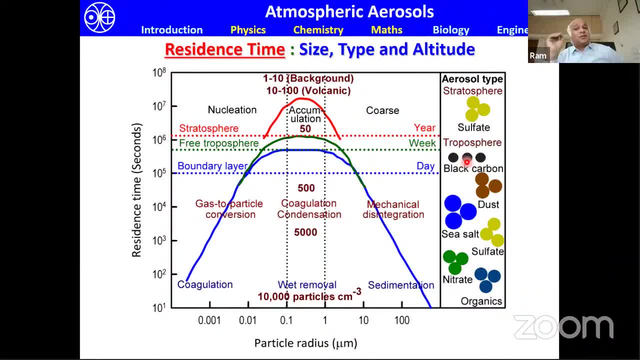 their residence time in the atmosphere also vary as a function of size, shape and altitude. Typically, you will have something like 10,000 particles per centimeter cube in the surface and then as you go up in the atmosphere, it will start decreasing. 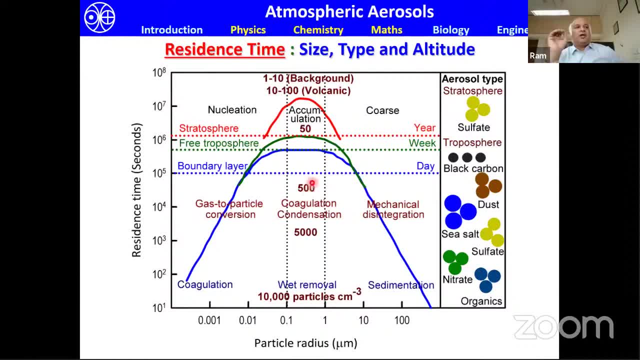 So when you go to the boundary layer, that's roughly about 3 kilometers or so, you can see a large difference or decrease from 10,000 to about 500 particles. and you go up a little further to free troposphere. 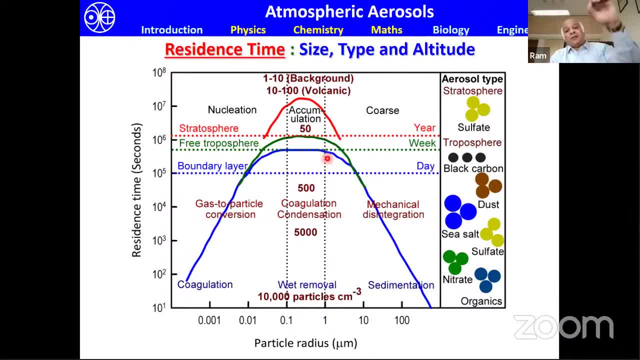 which is about 5 or 7 kilometers. then the number of particles will decrease. and you still go further. Stratosphere, for example, about 70 to 20 kilometers and above. the number of particles will become even smaller. 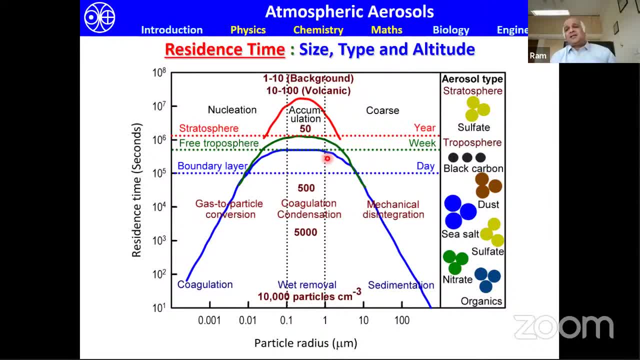 So on the x-axis, here is the radius of the particles. What you can see is that, as a function of altitude, the size of particles that are present also keeps varying because of the processes that are present here, Typically here in this small size range. 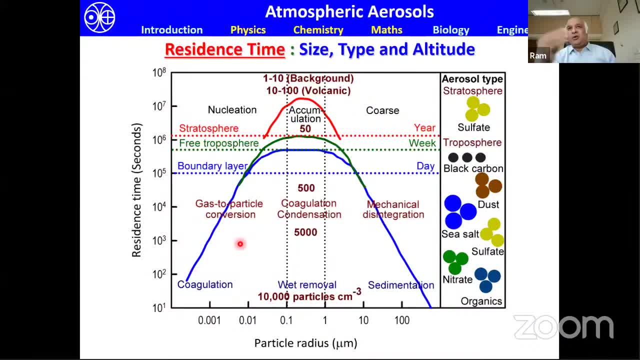 the residence time is on the order of a few hours to a day, and then they convert, through gas-to-particle conversion, into particles that are in the accumulation or condensation size ranges, While the particles that are larger than one micrometer or so. 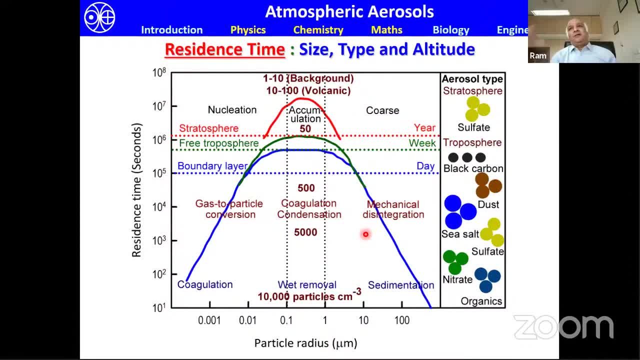 they feel the effect of gravity more effectively than the particles which are of smaller size, as you know, So they also settle out of the atmosphere in a few hours to one day's time. It is the particles within the size range of about 0.01 to one micrometer. 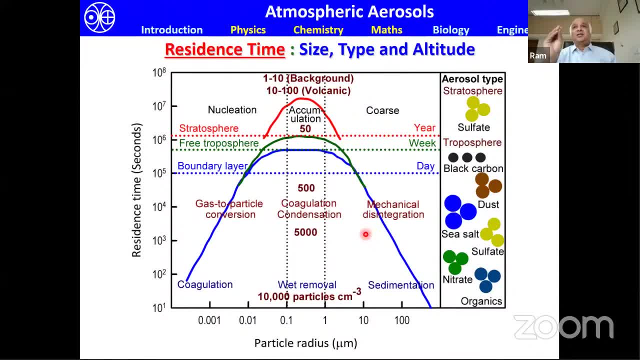 or less than 10 micrometer. They can stay a little longer than the particles that are smaller or bigger than this range, And even these will. the sizes will change as you go up in the Earth's atmosphere. And the other major difference between the aerosols. 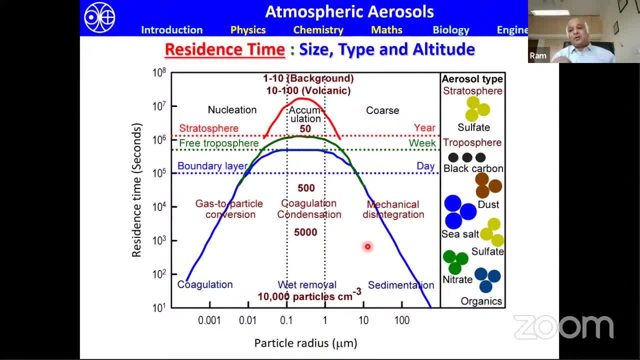 that are present in the troposphere with respect to stratosphere is that in the troposphere you can see all kinds of these particles that we saw before, But in the stratosphere, 99% or more, are only sulfate particles that are present. 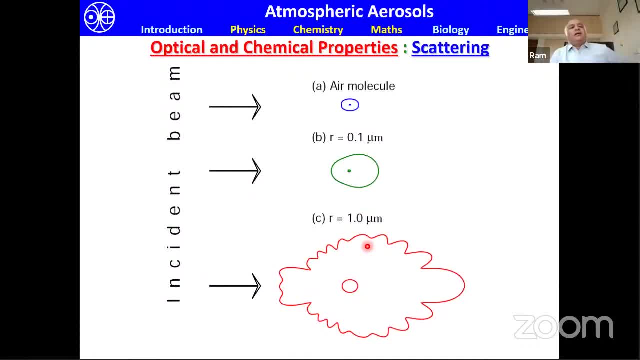 So when the electromagnetic radiation interacts with these particles, for example with an air molecule, we know that the interaction can be simply calculated as due to dipole scattering, where the radiation that is scattered is equally distributed in both forward and backward direction. 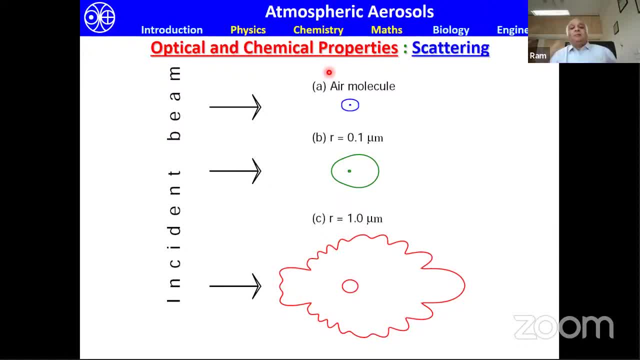 So it's a kind of a symmetry scattering that happens. But in case of an aerosol, for example, when the particle size is of the order of 0.1 micrometer, you will see a large forward scattering when compared to the air molecule. 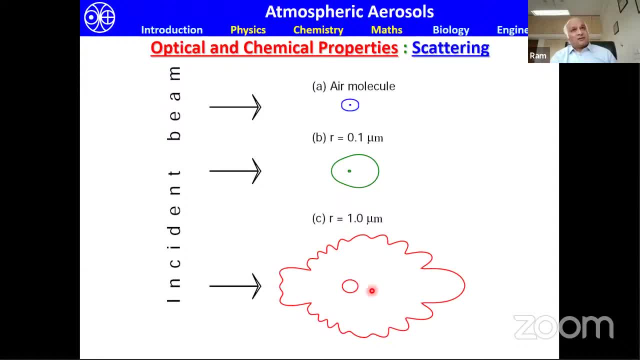 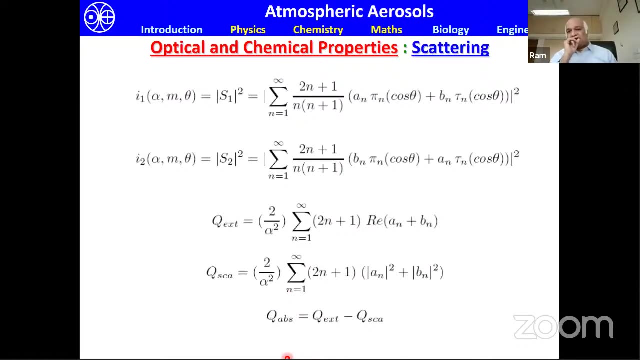 which is symmetric, And when the size increases further, the amount of light that is forward scattered will also be higher. When compared to the air molecule, the intensity that is scattered by aerosols in the perpendicular and parallel directions. they are a little more complicated. 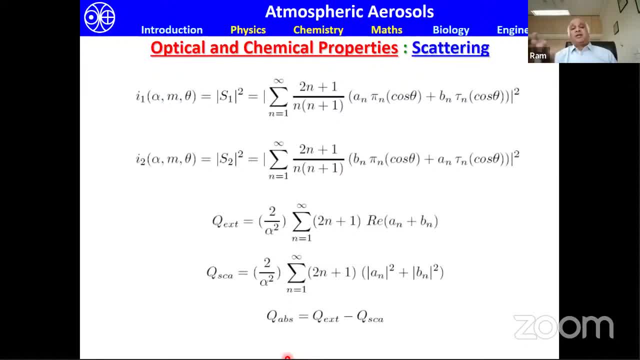 to derive using, for example, we use Legendre polynomials of argument n and order n and argument cos theta, where a, n and b n are the constants. So we calculate the amount of radiation that is scattered as a function of the size. 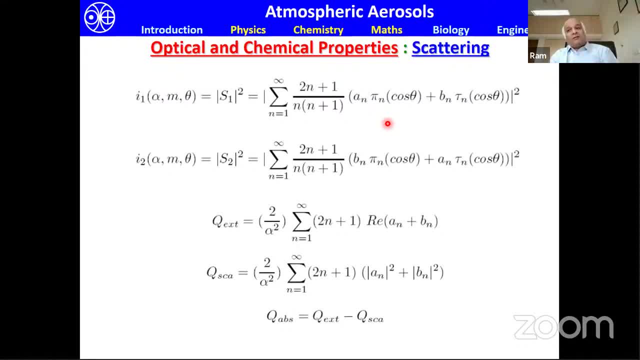 and also as a function of the refractive index. Why refractive index? we'll see in the next slide From that what we get. we calculate the extinction, which is the summation of scattering and absorption, and then calculate the scattering. 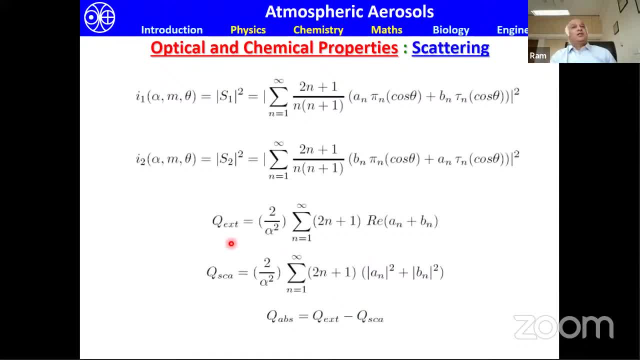 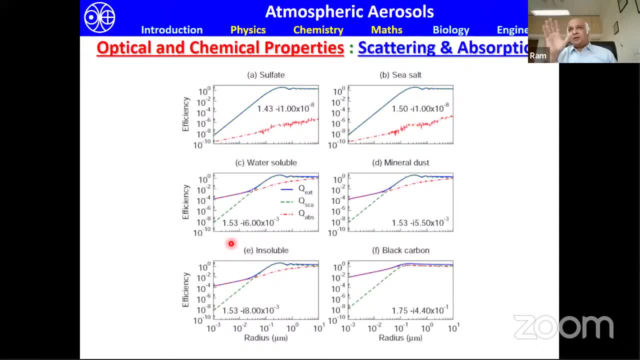 And then the difference between scattering and extinction gives rise to the absorption. So all these particles that are produced by different sources, different types, they can actually scatter and absorb the radiation. So each of the particles that you see in the atmosphere is characterized. 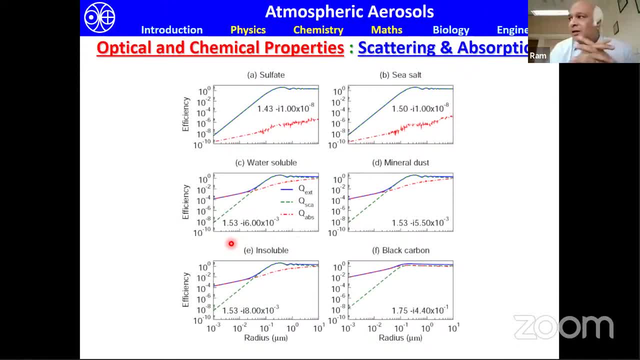 by a refractive index, including the air molecule, and which has a real and an imaginary part, as you are aware. The real part signifies the scattering contribution, while the imaginary part indicates the absorption contribution. The absorption contribution of air molecules is almost nil. 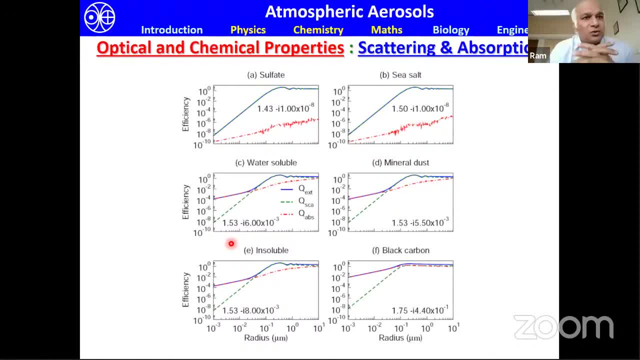 So the refractive index- imaginary refractive index- is small. So what we get is that the absorption of air molecules is small. So here, for example, I have shown the scattering efficiency, the extinction efficiency of particles, scattering and the absorption efficiency. 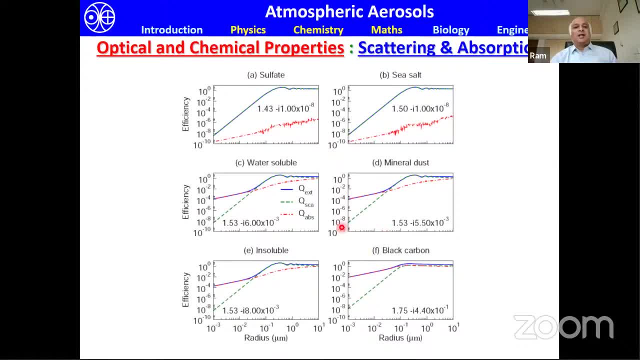 For example, let us focus on sulfate and black carbon. Sulfate, for example, the imaginary part is 1 in 10 to the power of minus 8.. For black carbon, it is 0.44.. You can see that. 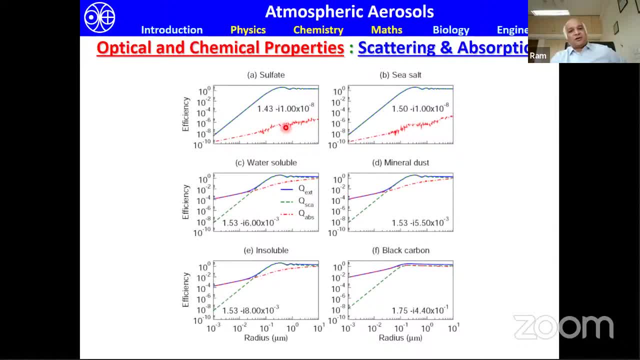 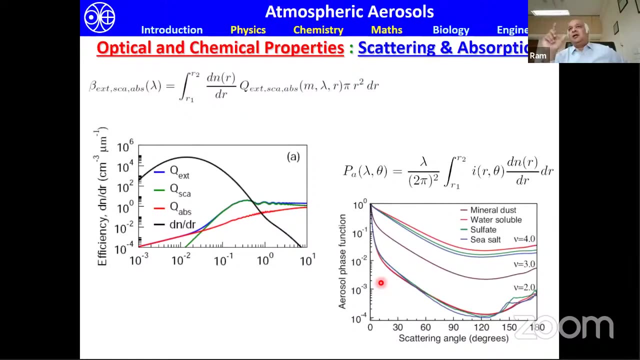 in the case of sulfate, there is no absorption that is contributing to extinction, while in case of black carbon, it is absorption that is contributing to extinction. So once we know how much is getting scattered, how much this particle of this size is absorbing, 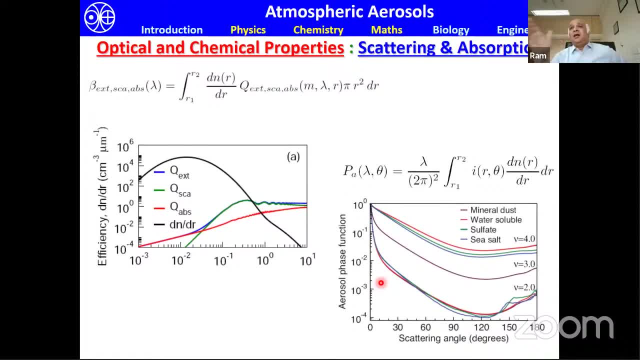 then we can, with the number of particles that is present, that we know, we can fuse the size, distribution and the scattering efficiency of these particles to derive the extinction efficiency or extinction coefficient, And how much of this radiation is getting forward scattered or how much. 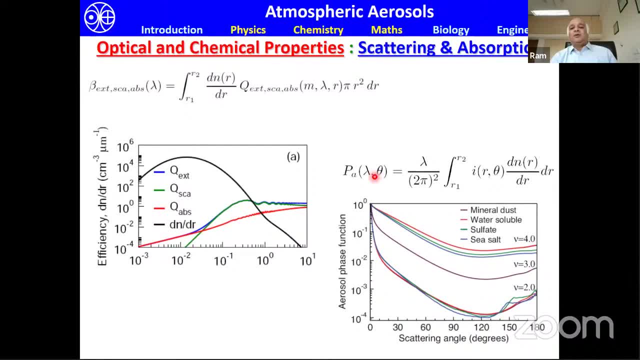 is backward scattered is calculated by using the aerosol phase function. So you can see that there is a large amount of forward scattering. that happens initially in the first few degrees and then it also changes as you go to the back sphere. The aerosols 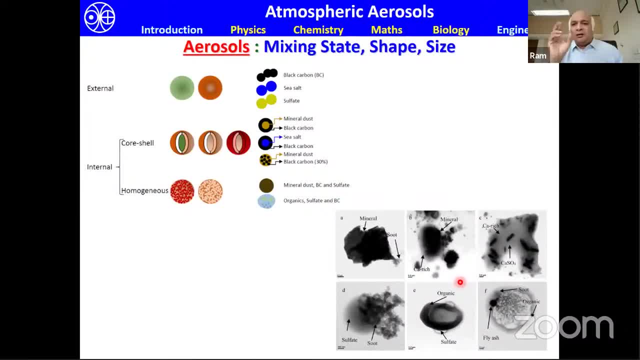 do not necessarily exist as individual components in the Earth's atmosphere, such as sulfate separately versus black carbon separately. They can also be present, mixed in the atmosphere, And one of the scenarios is actually a simple scenario which is external, while the other scenario is a little more complicated. 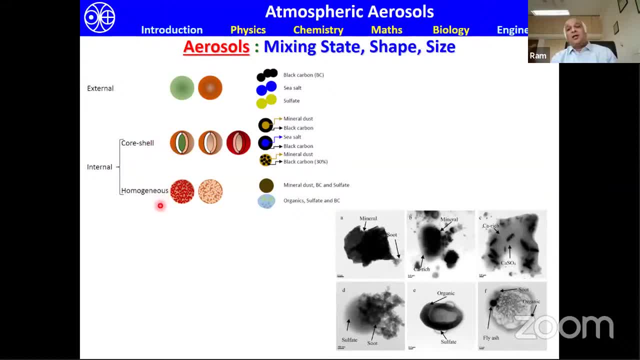 which is either the core shell or the homogeneous internal mixing. In core shell, one species forms the core and the other species acts as a shell, and in the homogeneous internal mixing all the species kind of get mixed together and form a shell And they can be. 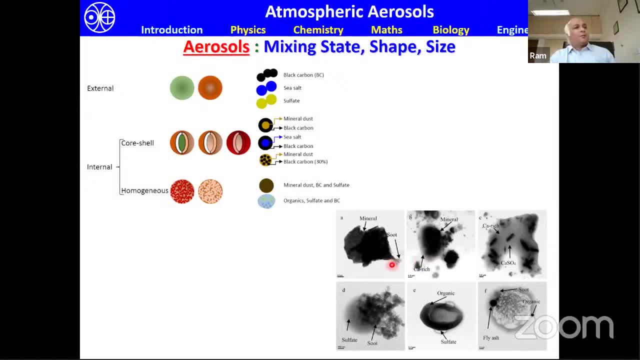 of different shapes also depending on the process that they are produced and the types of particles that are emitted, So and they can be of different sizes, as is also shown here. So this has a direct linkage to the phase function that we derived, depending on. 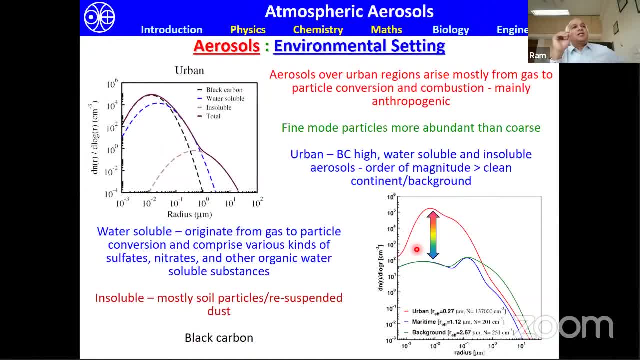 the shape of the particle. the phase function will also keep changing, So we can see different. So we come back to the aerosol distribution, the urban distribution which we saw. We know that aerosols or urban regions are mostly from a gastroparticle. 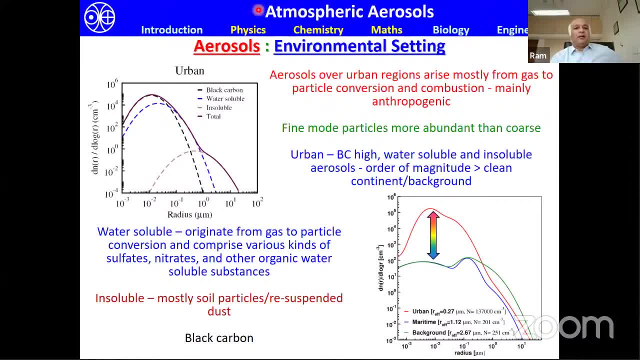 conversion and conversion mainly anthropogenic and typically particles in the fine mode, meaning less than one micrometer, are much, much larger than when with respect to particles that are larger than one micrometer, and particularly the aerosols over the urban regions, especially in the fine mode. 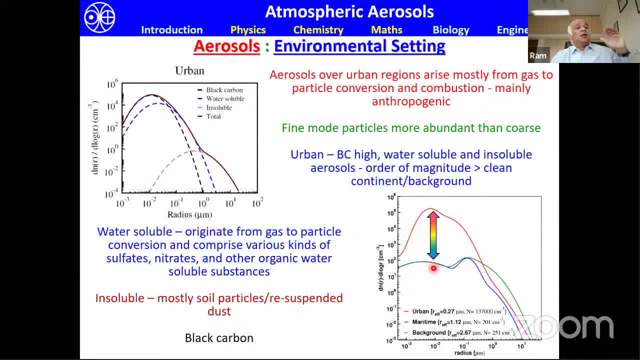 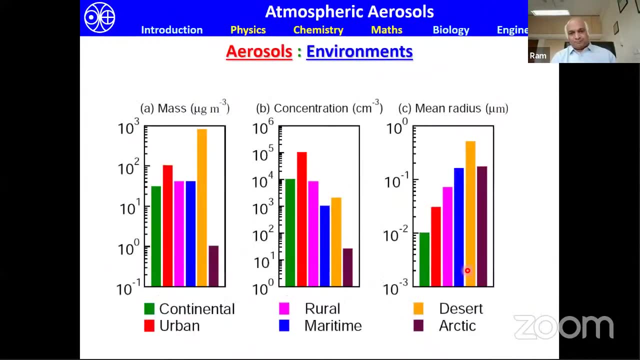 are about more than one knot of magnitude when compared to a clean continental or a background or a marine region. But when you go to marine region, for example, you will see that the particles of bigger sizes, the sea salt particles, are typically larger than the urban. 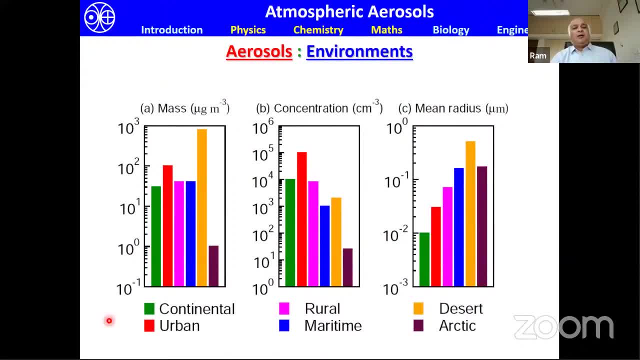 fine mode species. So this is an aspect- that, depending on the environment and the chemical makeup of these particles, the sizes, the numbers and the mass can vary. So if you look at the radius, for example, from the urban to desert, just like fine to coarse mode, 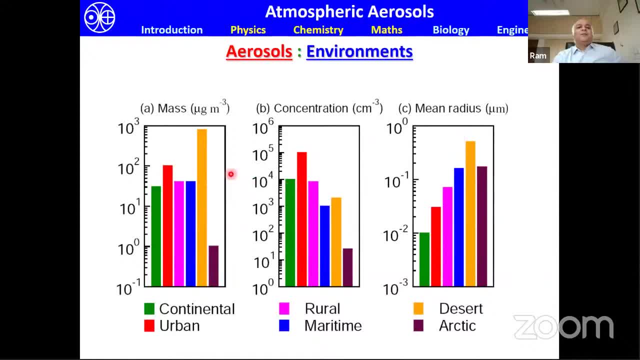 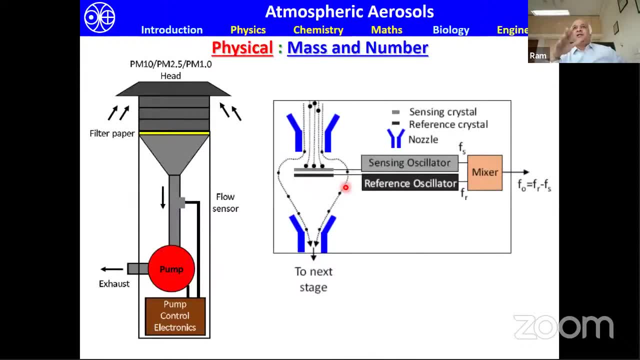 you can see that the radius of the particle increases, Typically, the mass and the numbers also change accordingly. So once we know about the chemistry and the fundamental principles of how these aerosols work, then we resort to developing the instruments, which can be ranging from a 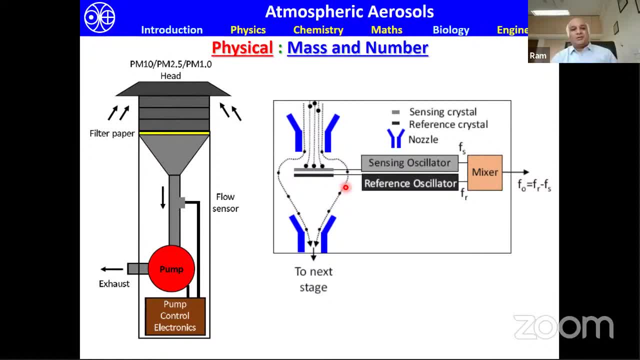 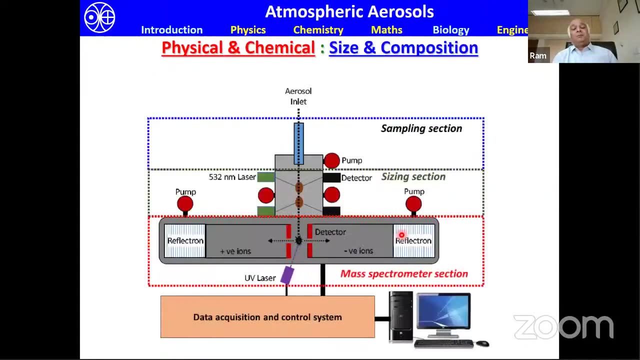 very simple method of just collecting the air on a sample and then trying to analyze using a high volume sampler and then further with chromatography techniques, you can actually derive the size distribution of the particles to a very, very sophisticated mass spectrometer where you can actually derive both. 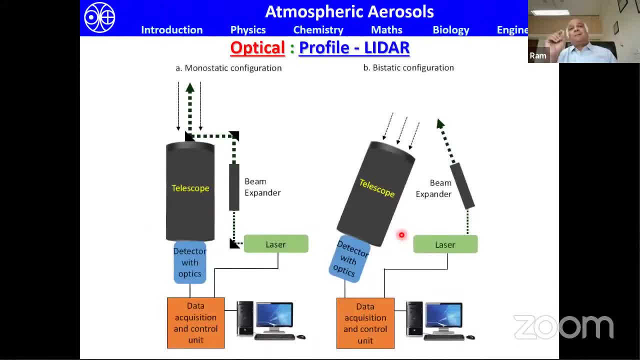 the size and the chemical composition of the particle to obtaining a vertical profile of the aerosol particles. use the laser, which we call as a laser radar, light reduction and ranging similar to the radio reduction and ranging to a very simple, and then you collected the scattered intensity. 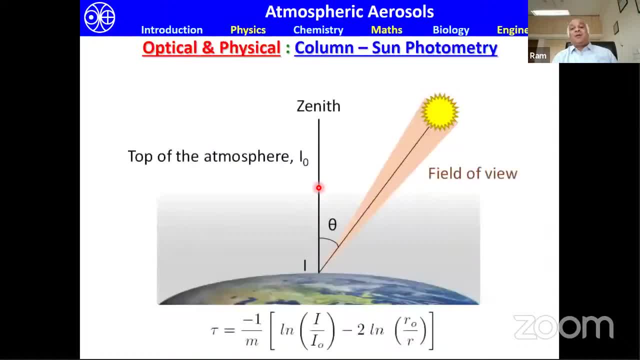 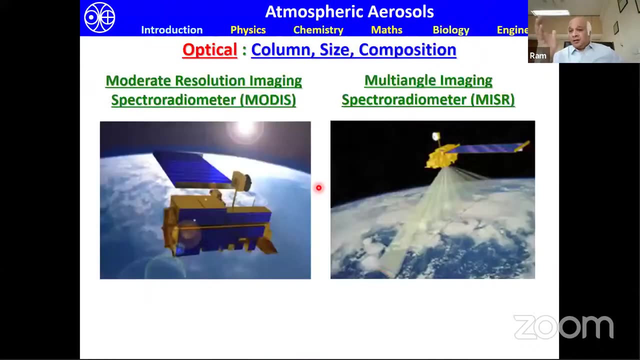 as a function of altitude, where you can actually map the vertical distribution of these aerosol particles, or the most simple technique, which is the sun photometer technique, which measures the column or amount of aerosols present in the atmosphere. currently, for example, there are several of them. 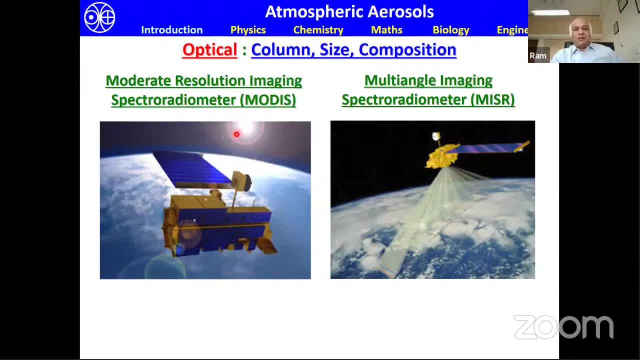 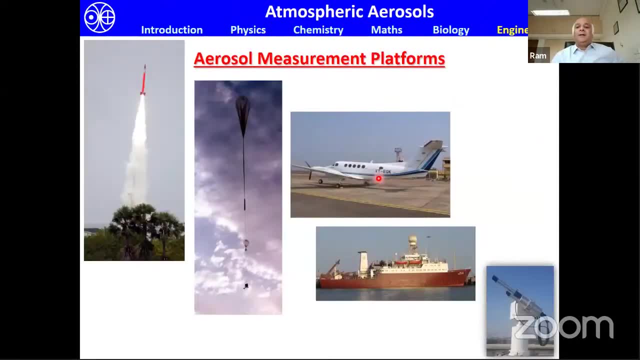 to measure the aerosol column size and composition, which includes the MODIS and MISER- I'm sure you are aware of these satellites and the payloads in it- and then the different platforms that we use, starting from down waste to go on ships, on aircraft, on balloon. 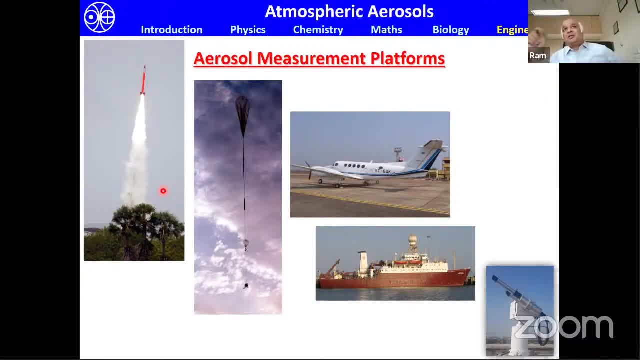 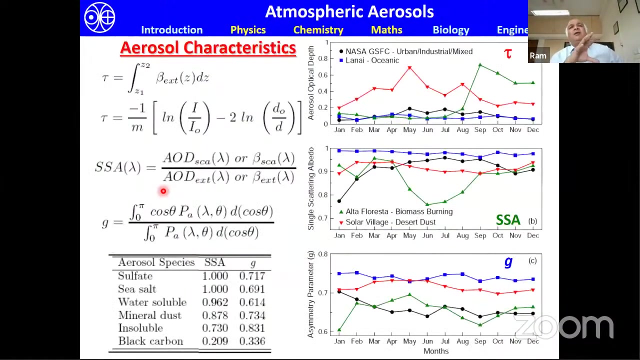 and rocket. we use a variety of them, for which the characteristics that you are interested in studying, for example, whether it is a surface, vertical or the column, they matter. whether as a function of wavelength, altitude, etc. depending on that and the characteristic of interest, the techniques vary. so 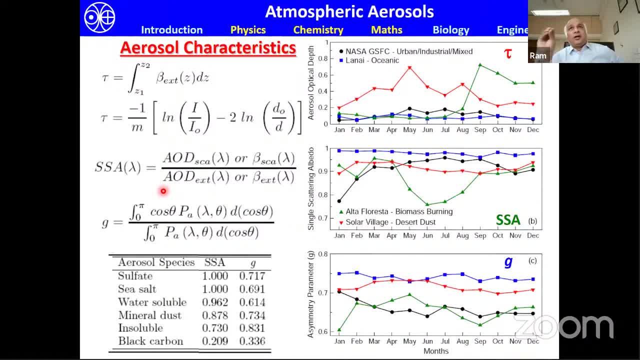 having talked about the aerosols, let us look at some of the features of the aerosol species. one is the. there are three parameters that describe the aerosol in whole, which is the optical depth, the column distribution of the aerosols in the atmosphere, the single scattering. 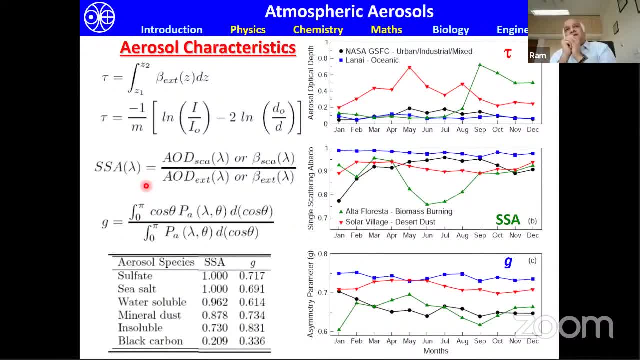 albedo, which is the ratio of scattering which is backward scattered versus how much is backward scattered, etc. so if you look at the values- for example sulfate being a perfect scatter, these, the single scattering albedo of sulfate is actually one, because there is no distinction- is mostly. 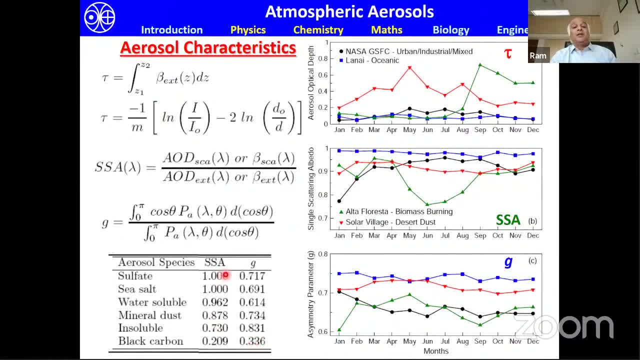 by black absorption to in black carbon. so you can see the single scattering albedo is a perfect one for sulfate and sea salt. while it is black, carbon is the single largest absorber of solar radiation in the earth's atmosphere. in a similar way for particles that are 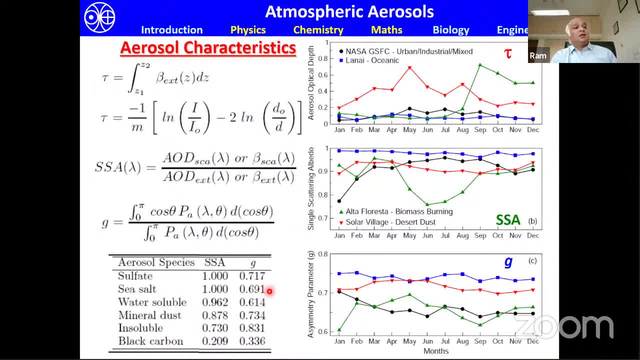 bigger in size, for example mineral dust or sea salt. the g values are higher when compared to the black carbon, which are mostly in the fine mode species or small size particles. so, over different environments, how these optical depths are influenced by desert dust, more number of particles, while 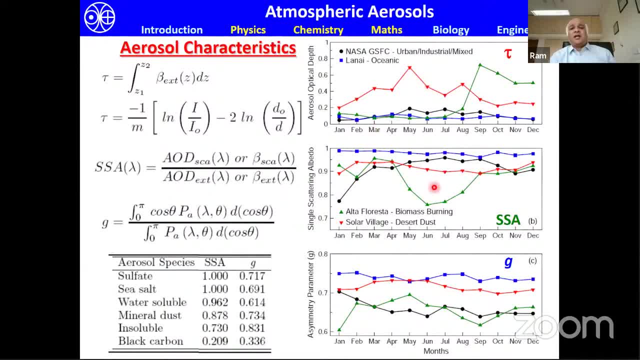 the. if you look at the single scattering albedo, when the region has a mixed influence, such as the oceanic region, you can see that the oceanic region has the biggest, highest g value and compared to what is present over the urban or the biomass burning regions. 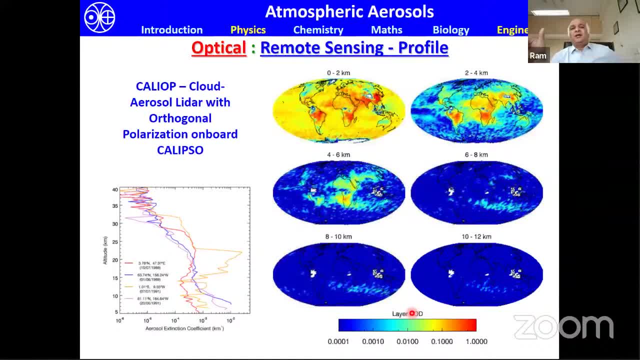 typically the particles are in the fine mode. so the asymmetric parameter also small kind of a slab layer, aod. then you see that most of these are present in the first five kilometers in the earth's atmosphere. but the scenario will change when there is a volcanic eruption. 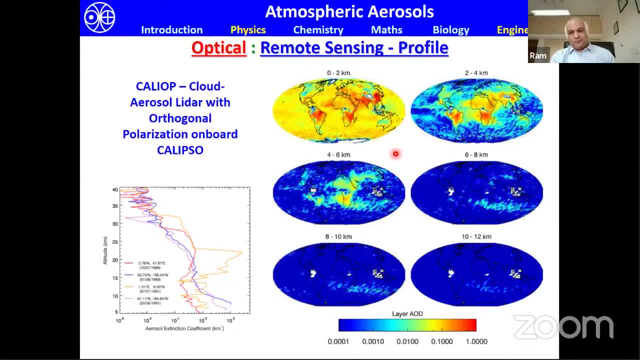 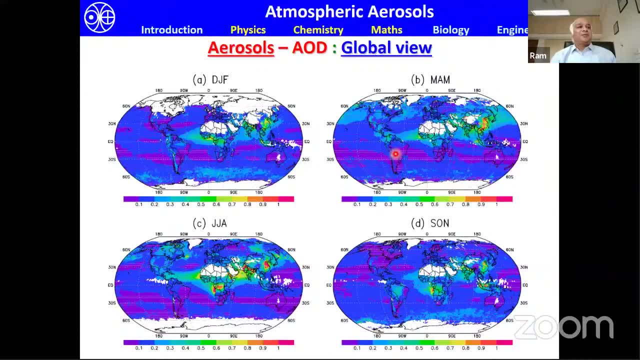 as you will see later. so most or almost 95 percent of these aerosols that are present in this same species, the aerosol optical, look, you can see that it is not uniform across the globe and it also exhibits seasonal and spatial variations. so you also see the 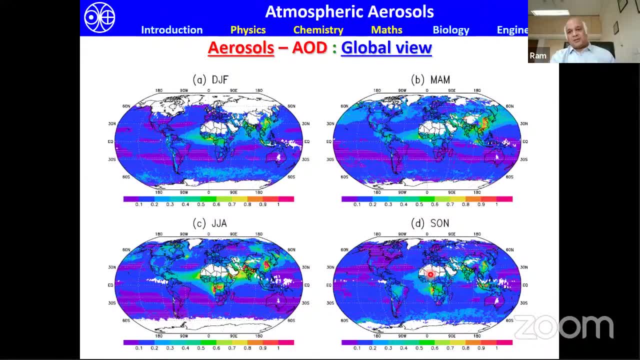 effects of transport over the during the monsoon months, the. the wind speeds. when they are a little higher, which are typically characterized by wind speeds that are greater than 10 to 15 meters per second, they produce a lot of sea salt and hence sea salt aody. 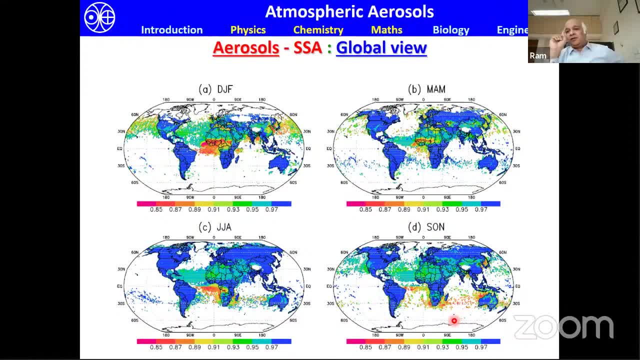 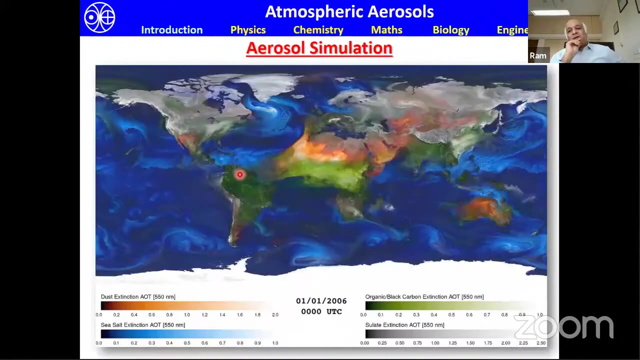 which you can see in this graph. so we can see that, these different regions of the external surface, and from this point, we can see that if we look at the changing during, than compared to the scattering type. and okay now, um, i just wanted to show that as an illustration. 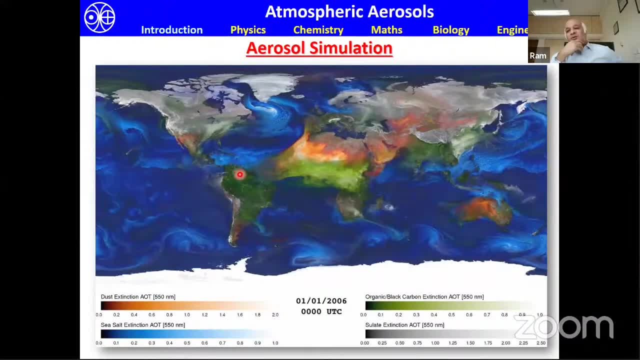 that the the life of an. with aerosols, for example, there is no dull movement at all in life. so here what we will see is a simulation of various aerosol species on a global scale. this will run for about two minutes, but i will keep talking in between, so you have a dusting brown color. 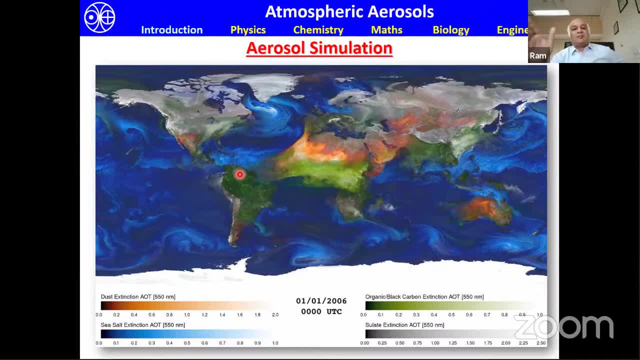 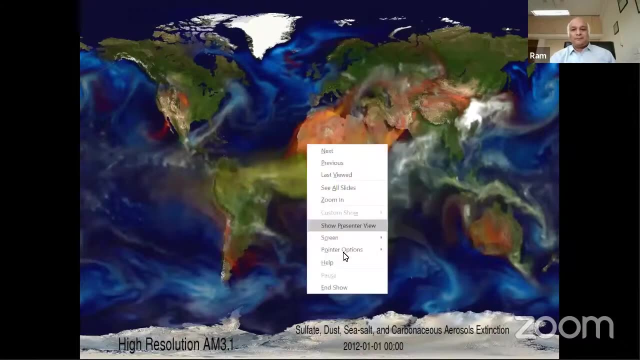 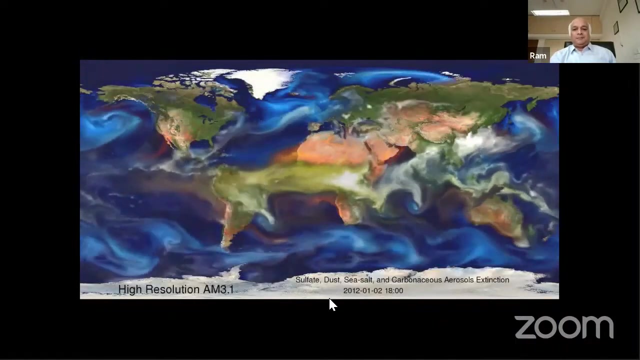 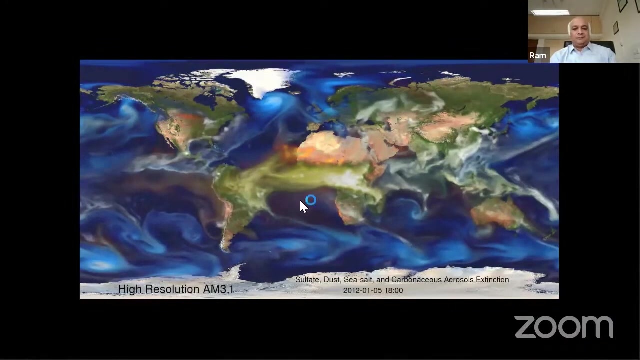 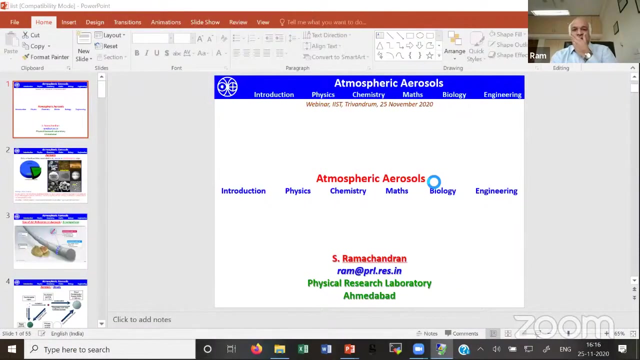 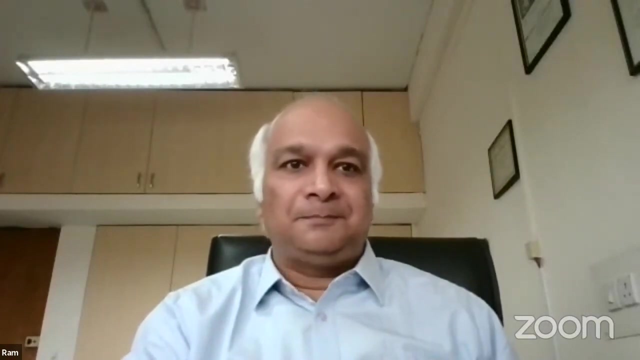 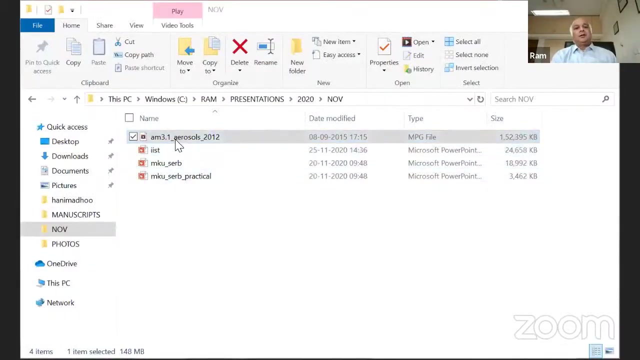 a green, darkish green, is the organic of the black carbon. sea salt is in blue and kind of white to gray is actually the sulfate extinction. now let me, let me play the movie. um, sorry, um, let me go back, sorry, so i'm i'm playing the movie separately, so, um, so what you are seeing here is the. 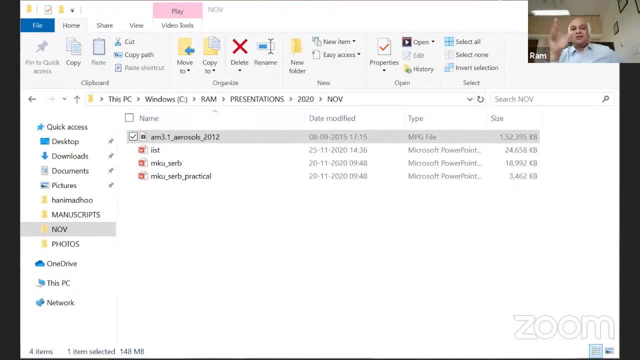 that you can see that all aerosols of all kinds, different kinds, they are spread across the entire globe and they keep changing on the. you can see the variation in time of the aerosols. as you um, as the time is changing, you can see the types of particles are also changing. 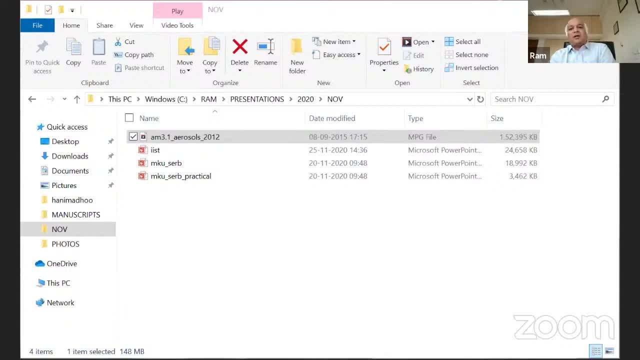 um, for example, let us just concentrate around the indian subcontinent. you can see, yes, really okay, okay, okay, okay, okay, just a minute, just a minute. so so now can you see? so, so, so I'm sharing the screen. are you seeing now? no, sir, what about this? 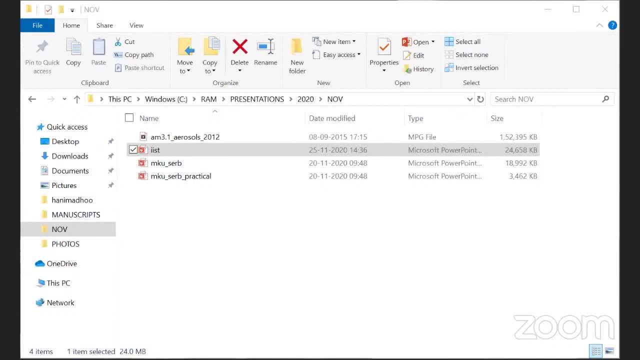 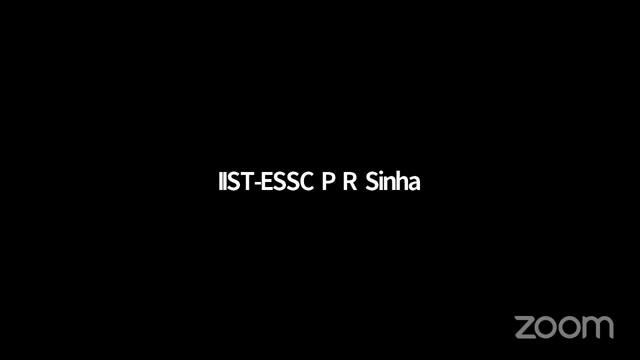 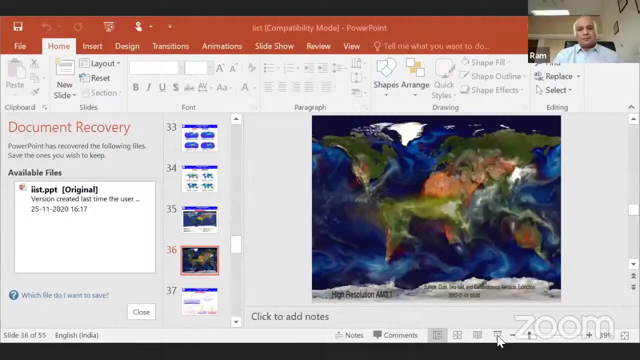 only folder. oh, really, okay, and you have to reshare it, share it, and you have to reshare it, share it, um, share it, share it, let me stop sharing, and i will now let me stop sharing and i will now share, share, yeah, yeah, you can play it. 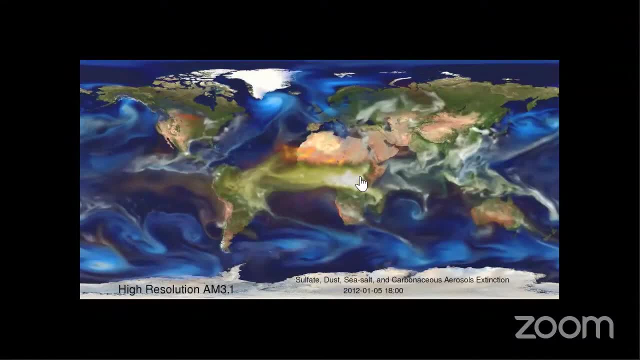 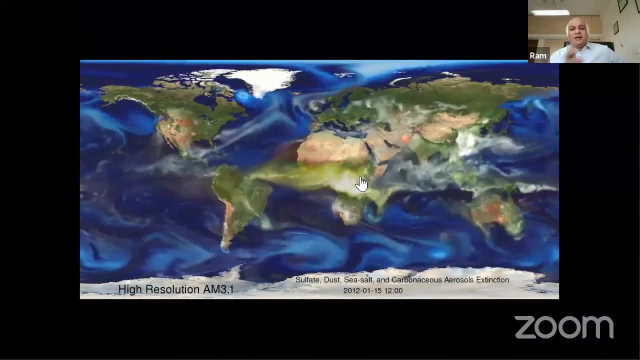 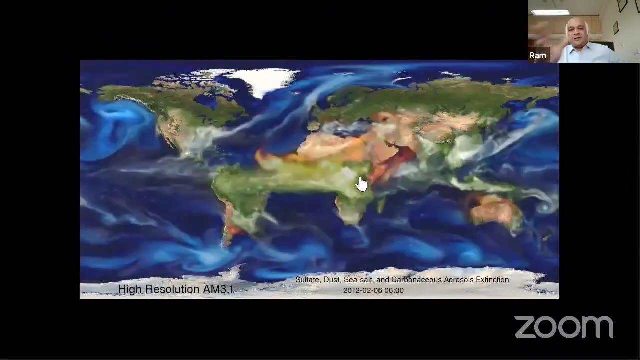 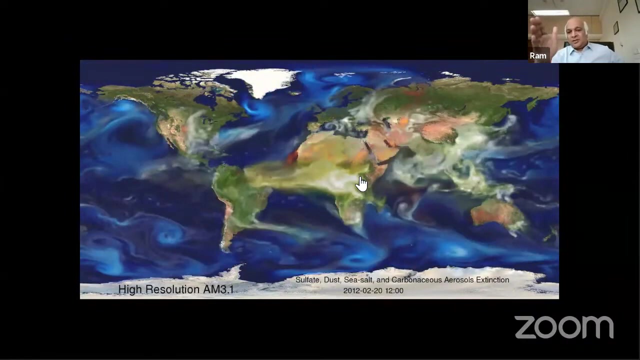 you can play it. yeah, can you see? yeah, can you see? okay, Okay. so what we are seeing is, across the globe, aerosols of different types are produced and they are getting transported across. So, if you concentrate, just looking over the Indian region now, it is approaching to March. 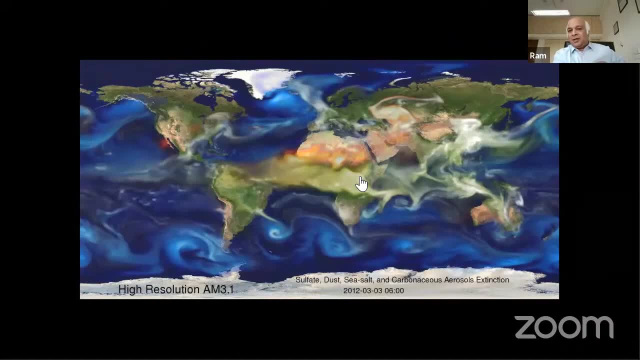 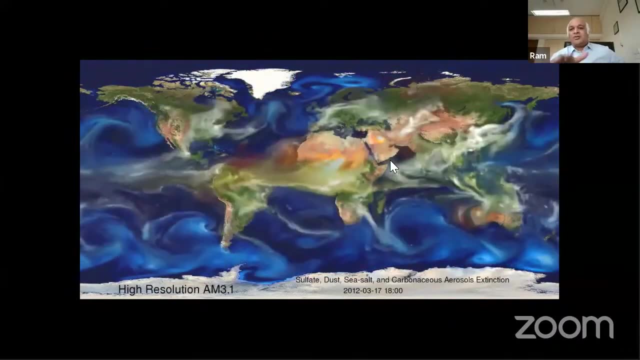 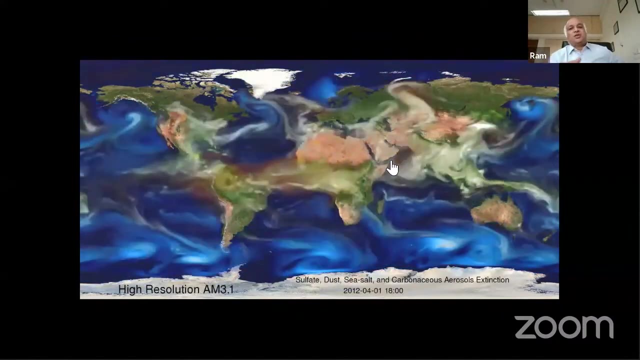 April, May. you can see a large amount of dust particles that is coming from the desert regions, the arid regions that are surrounding, and you can also see the pattern that is changing. during monsoon You will see a lot of sea salt that is sweeping across the Indian subcontinent. 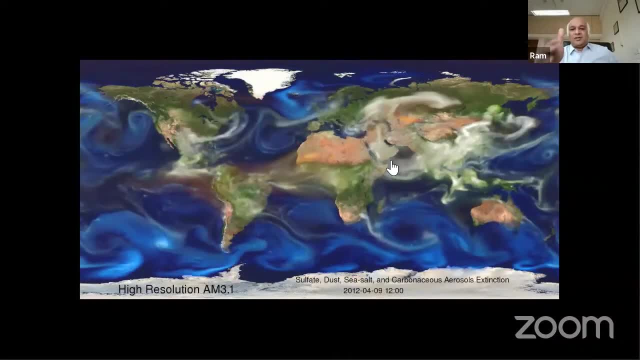 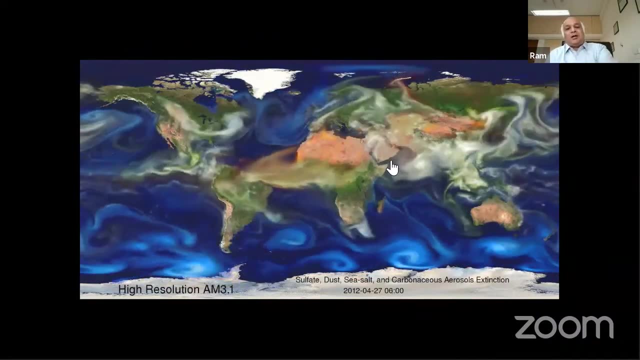 We are still in April, So you can see across the other regions of the globe. you can see the southern hemisphere, for example. it is a large amount of sea salt. through the gusts of wind You can see the sea salt that is being produced. 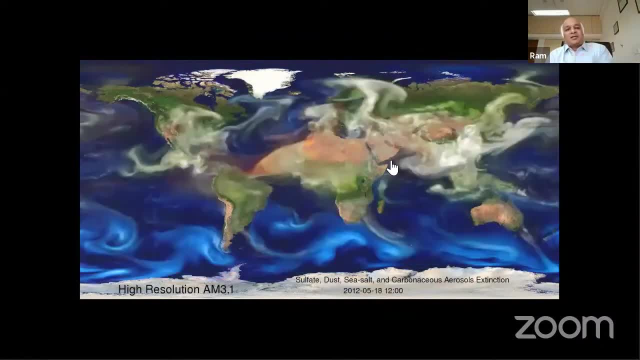 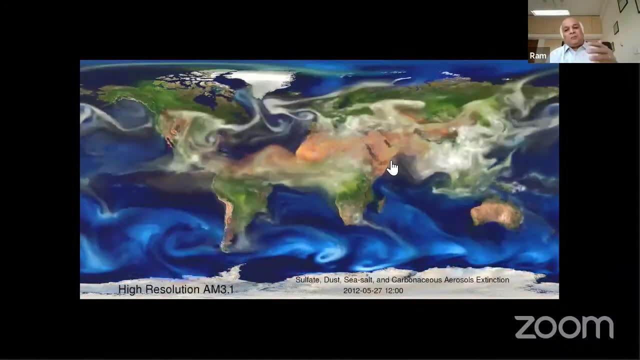 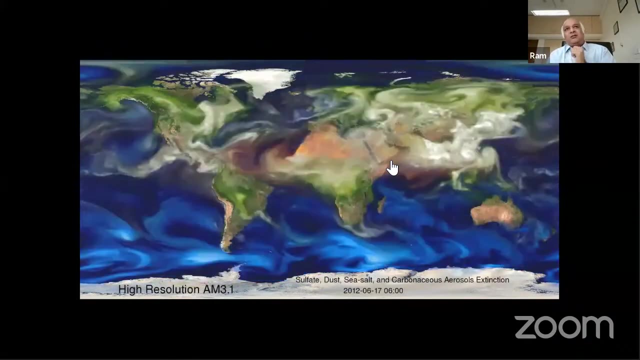 And so it is a very active and a dynamic system of aerosols being produced over a certain location and they getting transported across. So, at any given location, the characteristic of these particles will exhibit a change as a function of time- day, month and season, and also interannual. 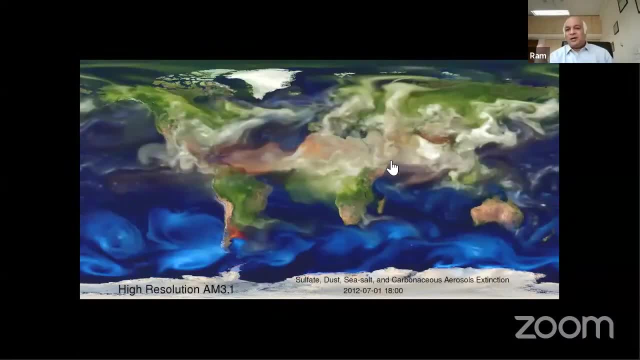 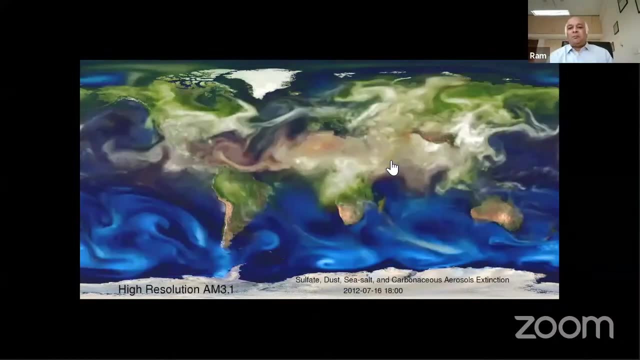 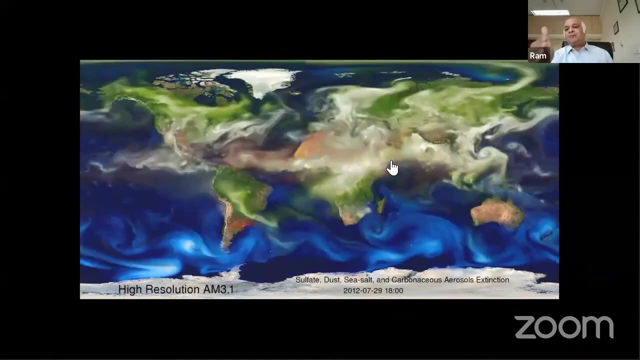 So now we are, the monsoon has started, So you can see that the whole it's a kind of a white to green to blue over the entire Indian subcontinent. A lot of amount of a large amount of sea salt dust, and the local production also contributes. 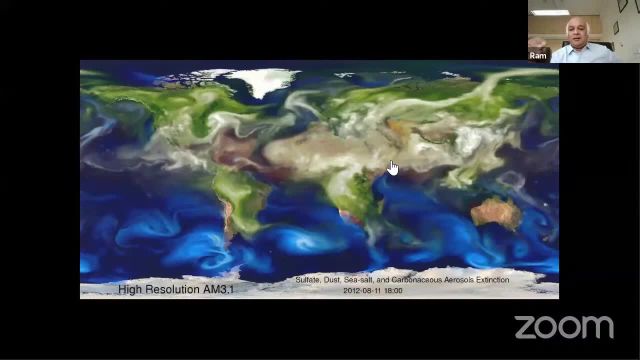 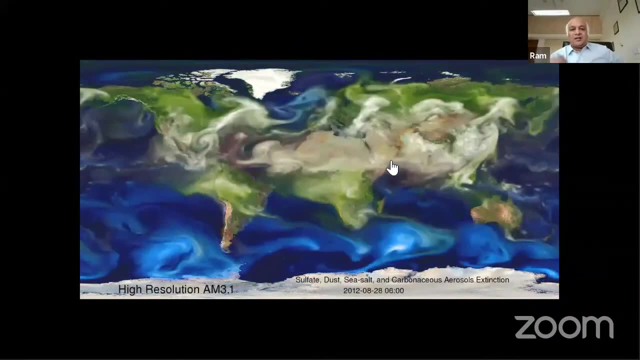 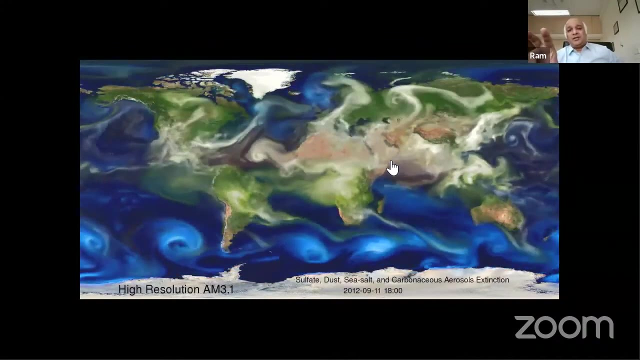 to the extinction here And then in about. so this is still. we are in August. So we are in August, Okay, And you will see a signatures of transport of from the African and the Southern American regions that we saw in the previous figure. 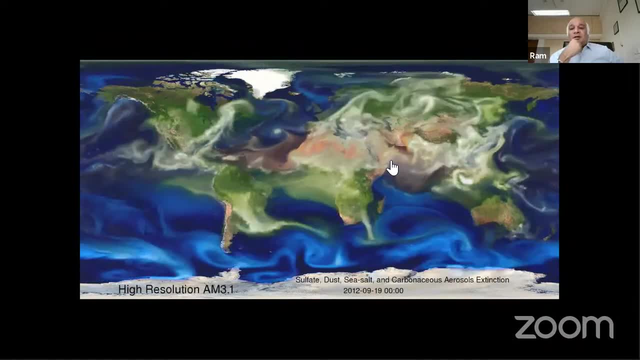 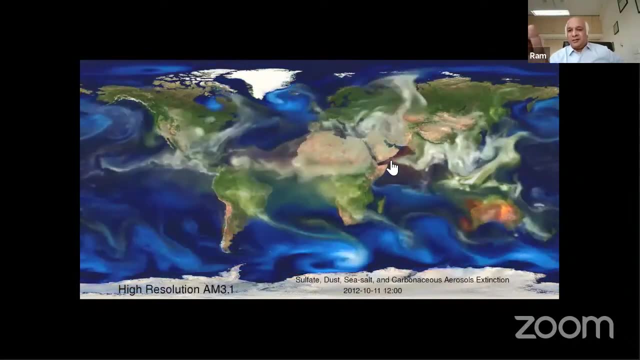 So now we are, we are going to be in post-monsoon. now You can see that actually, suddenly Indian India will become kind of cleaner. You can see the entire map of India that is visible with less aerosols because the monsoonal. 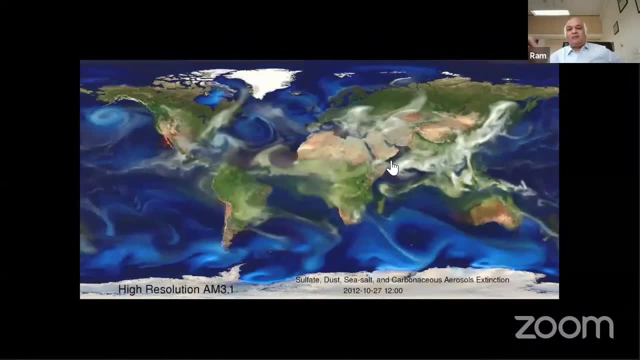 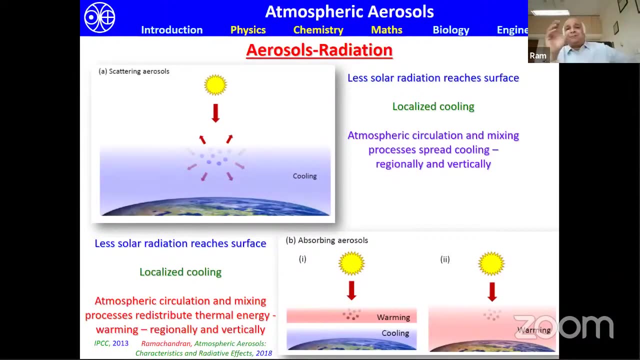 because of precipitation, the aerosols have settled or gone, gone out of the atmosphere. Okay, Now we looked at the physical, chemical, maths, biology, all these species, Why we should study, why are they important in the Earth's atmosphere? 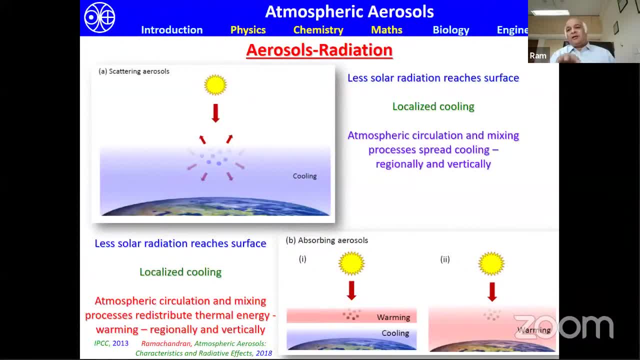 So, depending on whether these particles are scattering or absorbing, The effects on the atmosphere will also vary. So when it is scattering aerosols, for example, in both the cases please note that, both absorbing or scattering aerosols, the amount of radiation that reaches the Earth's surface will only 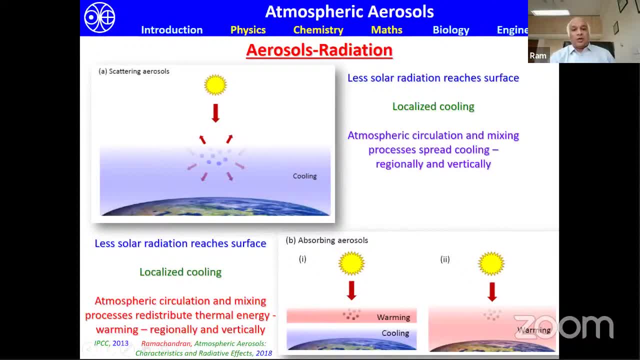 decrease will be lower. Hence both of them will produce actually a cooling, But later the sulfate or the scattering aerosols will actually contribute to localized cooling as as well as a cooling that spreads across the region. Okay, Okay, And as a function of the altitude, while in case of absorbing aerosols, the initially 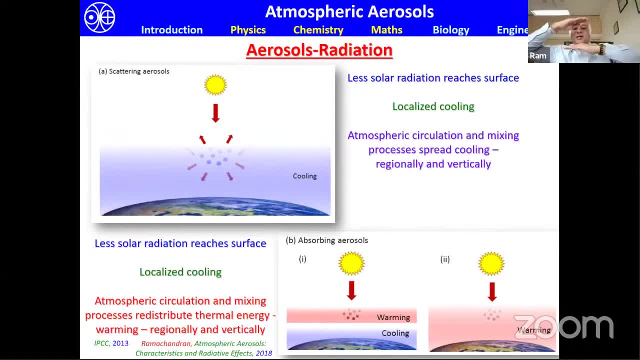 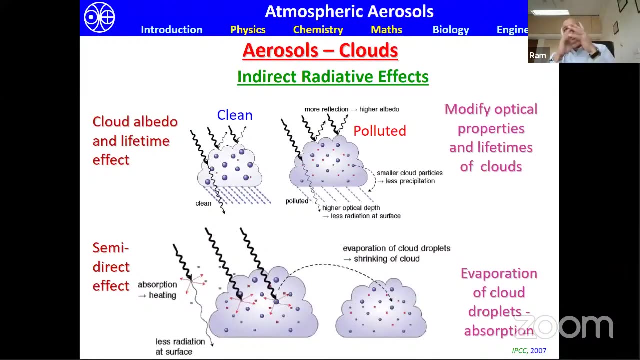 there will be a gradient, because it is cooling at the surface and warming at the higher altitude, But this will homogenize because of mixing, both in terms of vertical and horizontal scale, And then we actually contribute to warm In addition to the direct effects, as we also saw earlier that aerosols contribute to the 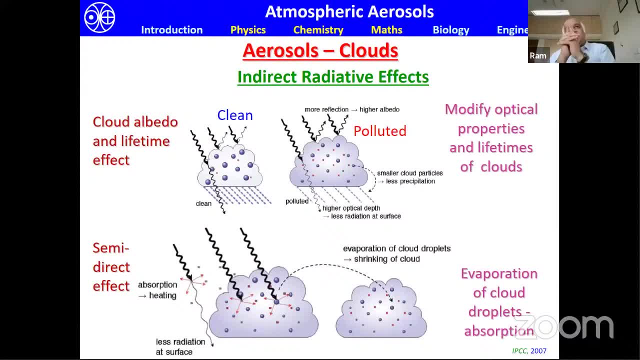 formation of clouds And depending on the nature of these particles that is present. when I say nature, it is the chemical nature of the particle and also the number that can be present between a cleaner and a polluted environment. The dust, the cloud, characteristics of the properties in the lifetimes also will change. 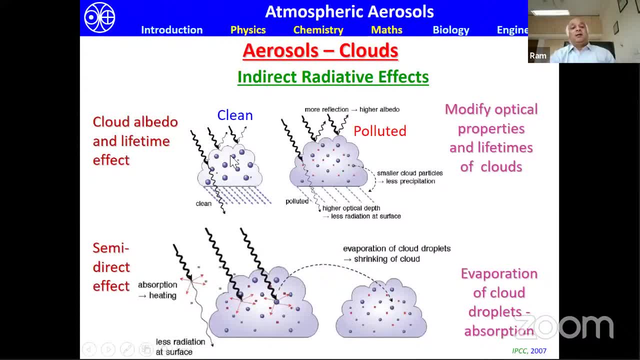 So, between a cleaner environment and a polluted environment, the size of the cloud droplets you can see, which is shown in blue circles, they actually reduce And you can also see more Red drops, which are the aerosols. This can modify the optical properties and lifetimes of clouds. 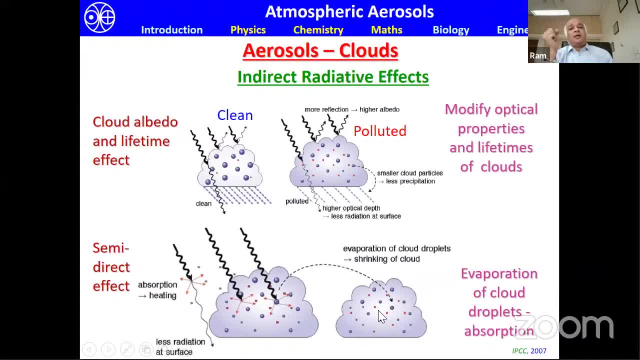 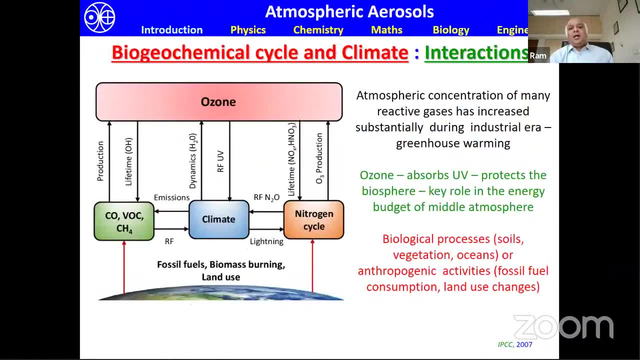 And if these aerosols are the absorbing nature, then it can actually burn off the clouds and then hence the evaporation can reduce. In addition, these aerosols form an important part of the global biogeochemical cycle. So when we say biogeochemical, 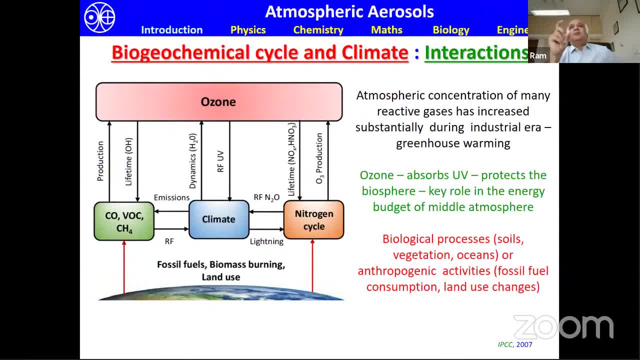 Any chemical. Any chemical, Anything that is a component of the Earth's atmosphere contributing to changes in terms of the biological, the chemical and the geological contribution, or changes in the system that contributes to biogeochemical cycle. So here, for example, the life cycles of most of these aerosol species present, namely be: 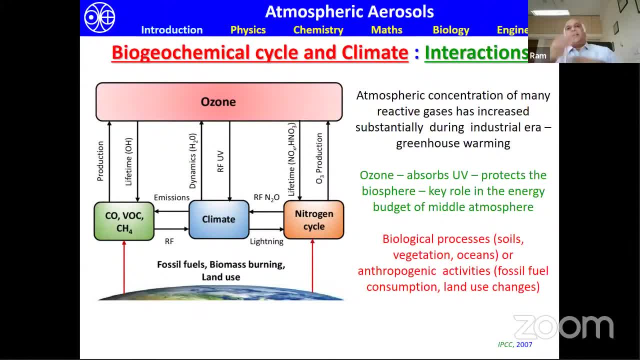 it carbon or sulfate or nitrate, et cetera. they all contribute to the geochemical cycle. So this is the biogeochemical cycle. This is the biogeochemical cycle. So we know that the atmospheric concentration of the gases have been increasing substantially. 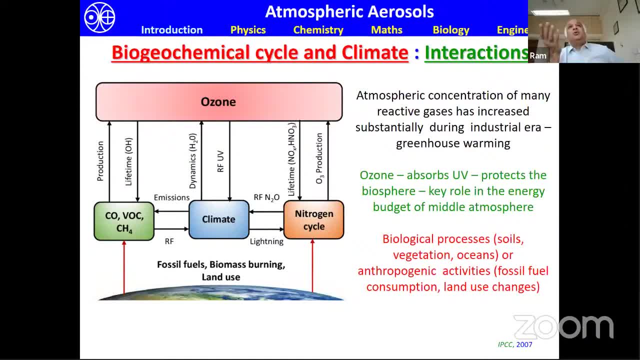 during the industrial era, which we call as a global warming. Ozone, as you are aware, absorbs the ultraviolet radiation. It plays a key role in the biosphere and also in the material atmosphere. It protects the harmful ultraviolet radiation. 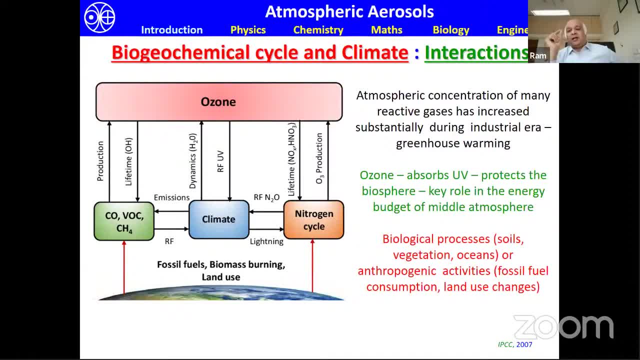 And then the biological process, Wherein the biogeochemical cycle comes. the changes in the soil, vegetation, oceans or anthropogenic activities, the emissions coming from this, namely the fossil fuel, the fossil fuel and biomass consumption, changes in the land use, et cetera, they all contribute to 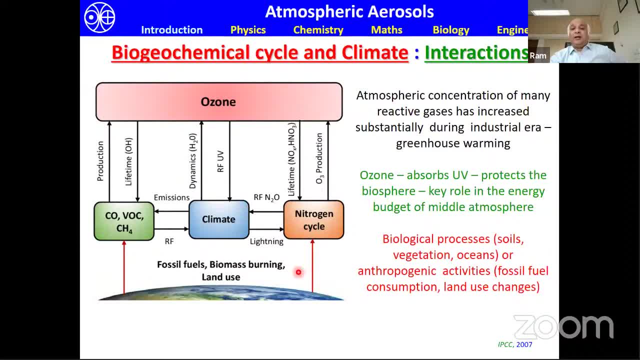 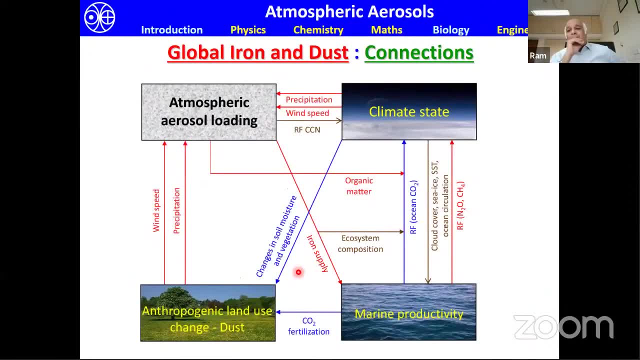 changes in the climate. So, directly and indirectly. So we know that, Directly and indirectly, aerosols form a part of this biogeochemical cycle. The next connection comes from the amount of dust that gets transported to the ocean. The dust is an important source of iron in the ocean. 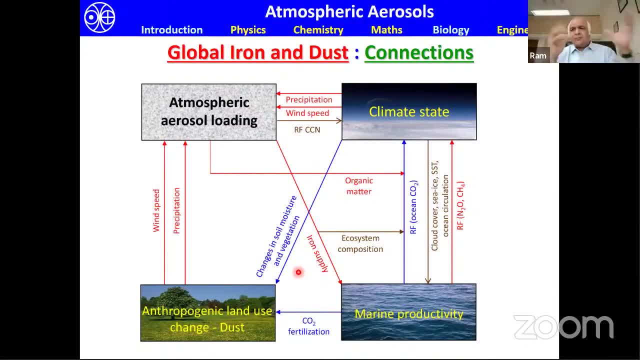 Now this one depends on the kind of scale of parameters that are involved, which includes the atmospheric aerosol loading, the state of climate, The changes in the land use And the dust that comes out of it, And the marine productivity. All of them are closely coupled. 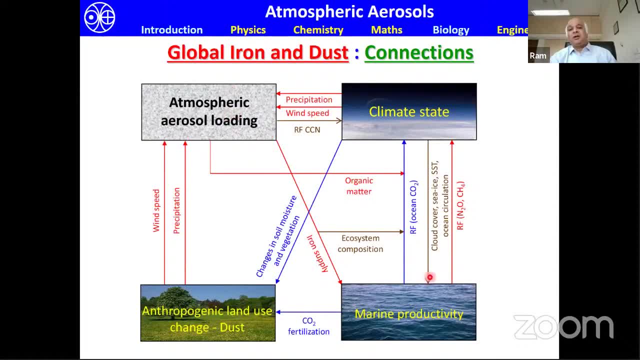 So you can see that the aerosol forms an important link in the entire biogeochemical cycle. Alteration or changes in any of these, to the climate or to marine productivity or land use, can influence the other aspect, other module, and then can contribute to the biogeochemical 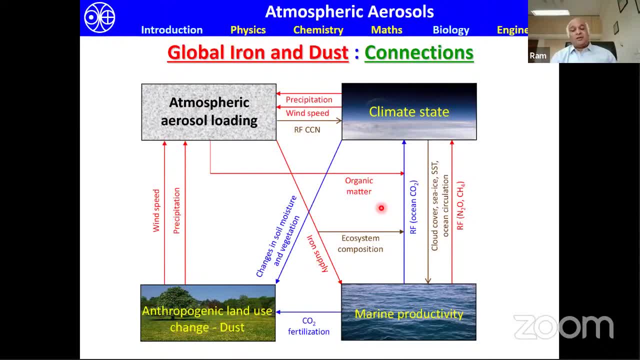 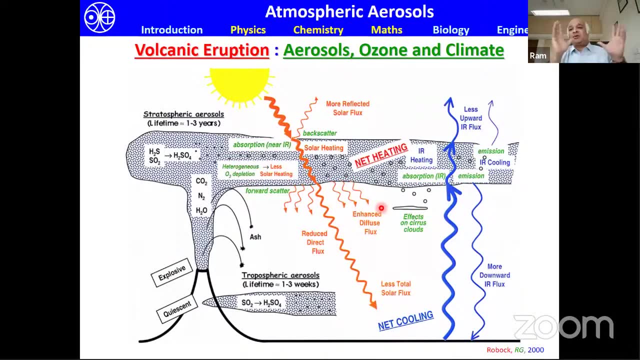 cycle And then can contribute to climate and the climate change. So one of the last aspects regarding aerosols is the aerosols that are emitted from the volcano. Volcanic eruptions usually inject tens of megatons of sulfur dioxide into the stratosphere. 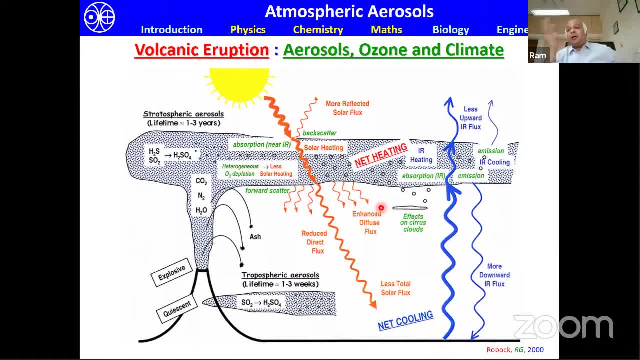 altitudes that are above 15 to 17 kilometer, depending on the magnitude of the eruption. It also injects carbon dioxide water into the stratosphere, And it also injects carbon dioxide water vapor, etc. But these are very small quantities with respect to the amount that is already available in. 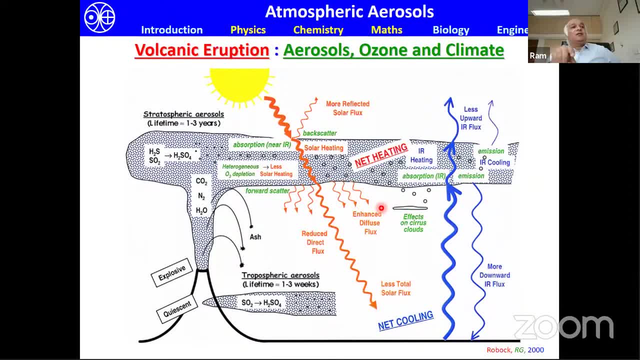 the Earth's atmosphere, But the sulfur dioxide gas that is ejected, which later forms into sulfate aerosols. they are a huge amount of contribution, addition to the already existing aerosols present in the Earth's atmosphere. Now these aerosols, once they are produced, the sulfate aerosols which are projected like 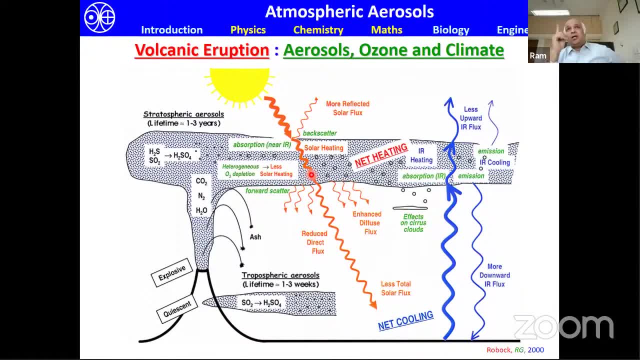 a fountain effect When they go to stratospheric altitudes, because these we have seen, they can scatter the incoming shortwave radiation, They block the radiation that is coming in. hence they will produce a cooling at the Earth's surface, But in terms of the long 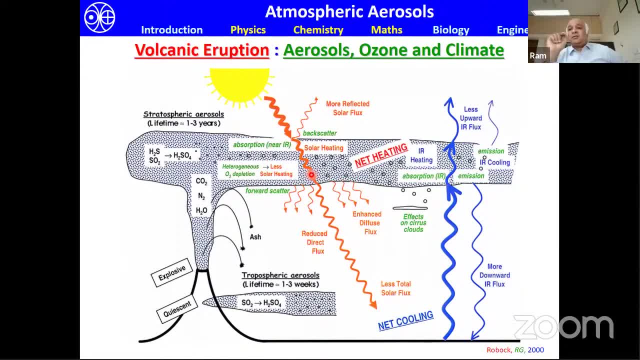 wave wavelengths above 4 micrometer. these very aerosols can absorb the Earth-emitted long wave radiation, And hence they produce contrasting results in the troposphere and in the stratosphere In addition, which is one of net cooling at the surface and one 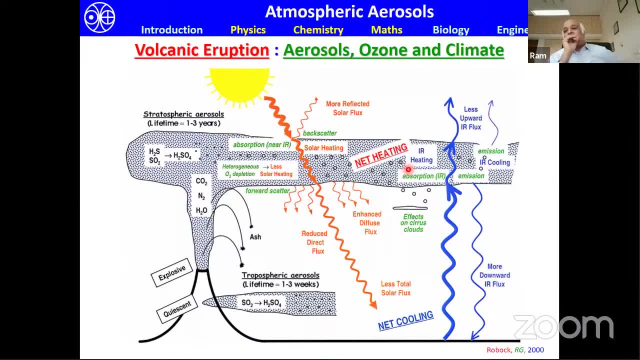 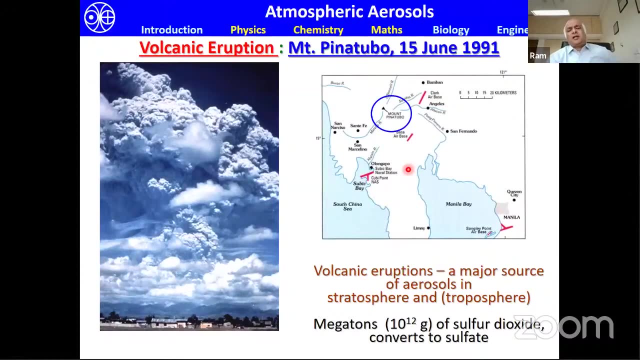 of net heating at the stratosphere. They also contribute to other changes. Major change occurs in terms of the depletion of ozone, which you will see in the next few slides. So we take as a pointer the largest eruption of the 20th century, which occurred on 15. 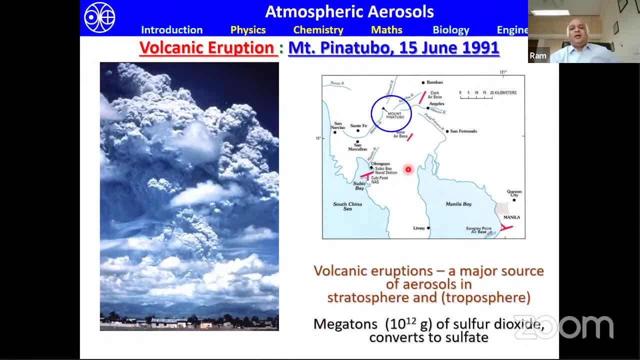 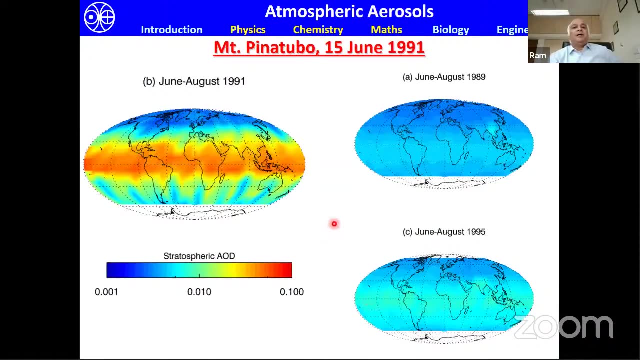 June 1991.. This eruption occurred in the late 19th century, namely Mount Pinatubo in the Luzon island of Manila, Philippines, 15 degree north and 120 degree east. It injected about 30 megatons of sulfur dioxide into the atmosphere. Now the optical depth, familiar optical depth. 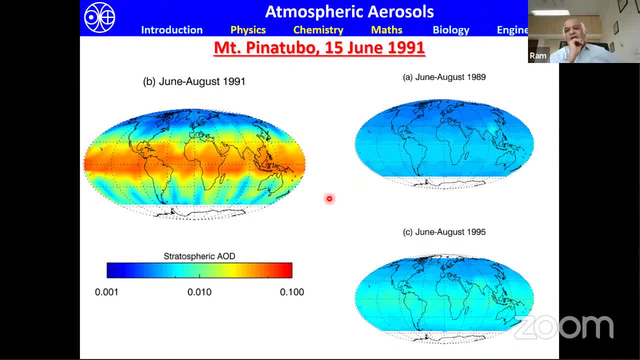 picture that we saw. this is only the stratosphere, which means 17 to 30 kilometers. This is the normal condition of optical depth in the stratosphere when there is no volcanic eruption. You can see that this is roughly 1.5 kilometers. This is the normal condition of optical depth in. 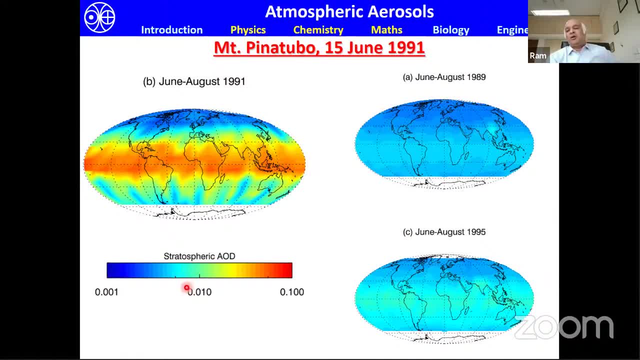 the stratosphere when there is no volcanic eruption. You can see that this is roughly about 0.01 to 0.01 during the normal conditions. But look at this when the eruption occurred in June 1991.. You can see that the subsequent three months you can see the optical depth. 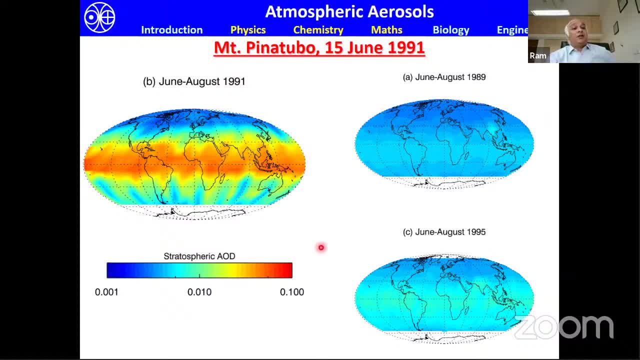 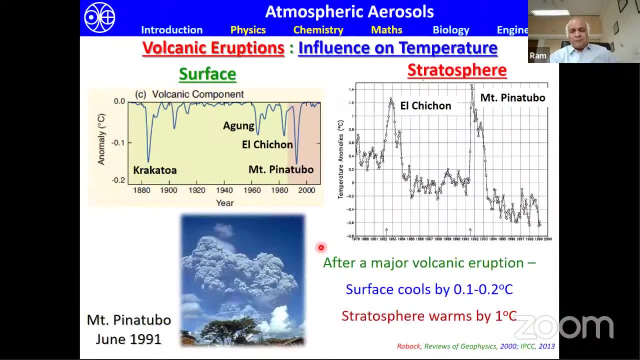 increased by about at least two orders of magnitude and the effect is global. Please note this point when we will revisit this in a few slides from now. So, as I mentioned earlier that the eruption occurred in the late 19th century, The eruption occurred in. 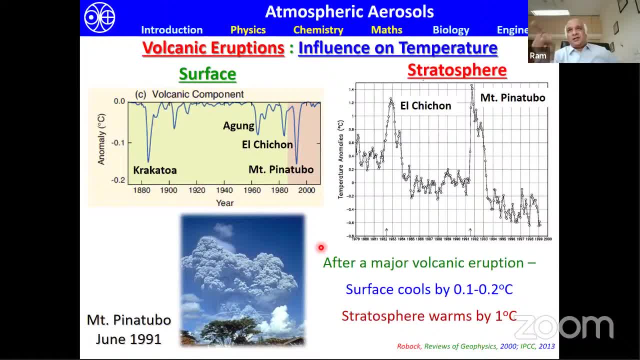 the late 19th century and the surface�other, and acknowledge it was formed in 1916.. And trends in the surface, as seen in the image below. here is one that is ropes for Francisco. the mount sea level crab to a sudden rise, in this case 10 to 20,000 kilometers, with 我們 youtuber. 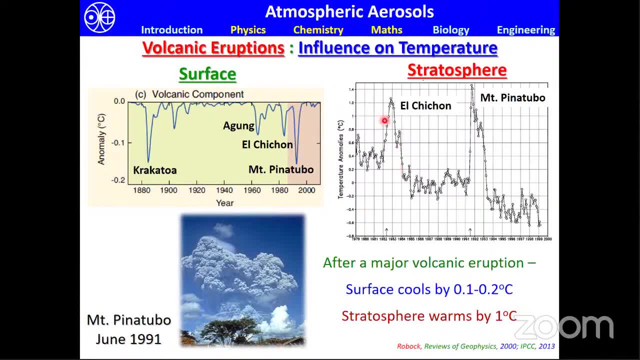 from Planet Pi Because of the reduction in the surface reaching shortwave radiation and absorption in the stratospheric long wave radiation at this stratosphere. it will produce that the sulfate aerosols or volcanic aerosols to produce a cooling of that surface. We can see that the 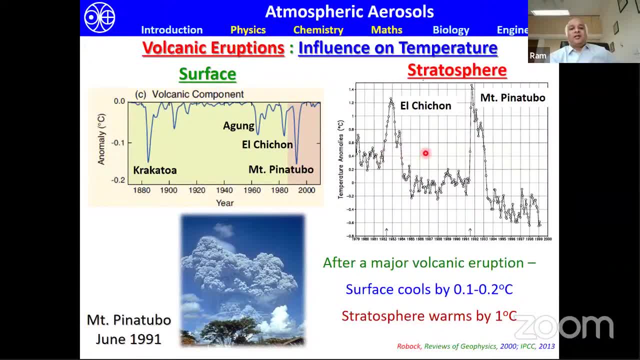 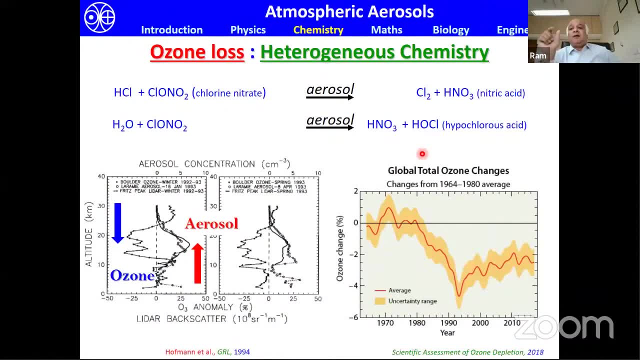 surface could after every volcanic eruption in history and the stratosphere gets warm by about after the eruption. Also note that these effects are transient, meaning going up to one or two years after the volcanic eruption. So when I was discussing the other process, I also mentioned 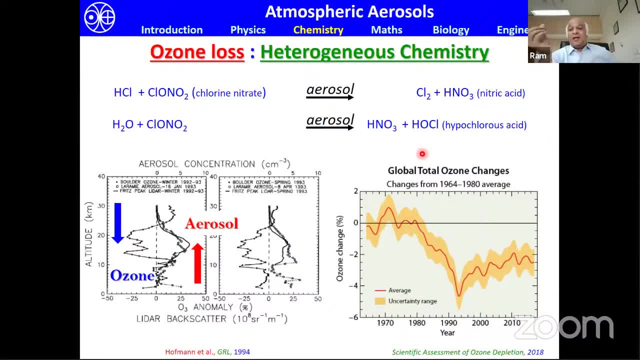 about these aerosols playing a role in ozone depletion. This again connects to the biogeochemical cycle distribution when aerosols contribute to the other aspects. As you are aware, the ozone depletion reactions take place on particles that provide surface areas for the reactions to occur. 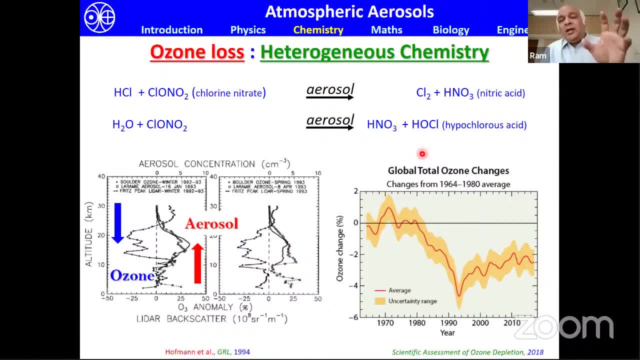 which are typically heterogeneous, meaning a solid or liquid particle is an aerosol and the gases that are present. So these are in different phases And because of this heterogeneous chemical reaction ozone can destroy, can decrease, So it will produce ozone depleting substances. 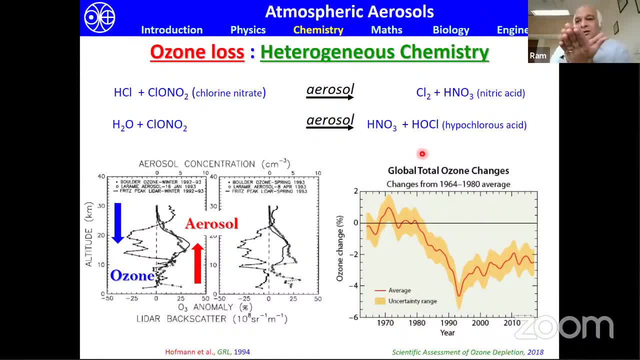 from the chlorofluorocarbons And these reactions. they occur on the aerosol surfaces. So in the background scenario versus a volcanically perturbed scenario, the major difference comes because of the following: There will be an increase in the number of particles in the stratosphere. And the second thing will be 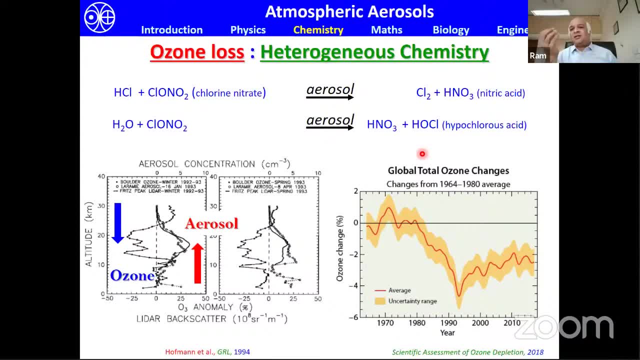 the increase in the size of the particle. So when the radius increases, as you know that the area increases by r squared, So these heterogeneous chemical reactions can occur at much faster rate when the number of these particles increases. So this is a very important. 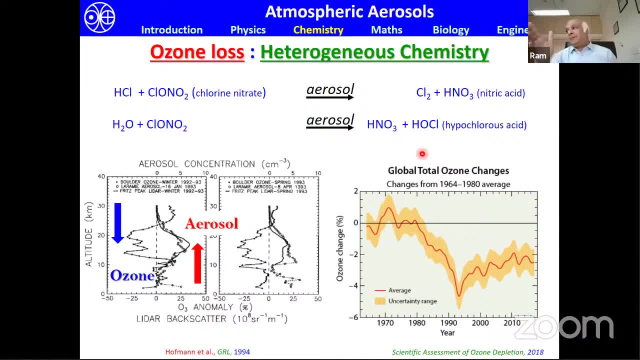 issue here because after the surface air growth is an aerosol, the size of these particles and the size of the particles increase, which happens after every volcanic eruption in the stratosphere. So you can see the close correspondence: where there is an aerosol increase, This is. 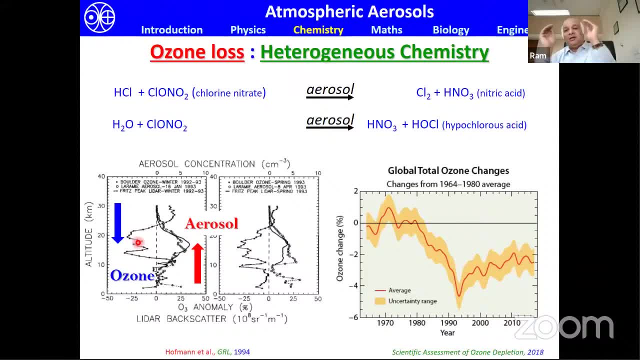 in the order of about 12 to 25 kilometers. There is a subsequent ozone decrease. So there is a close correspondence between the increase in aerosol with respect to a decrease in the ozone. You can see this effect in the global total ozone change. See that the large dip. 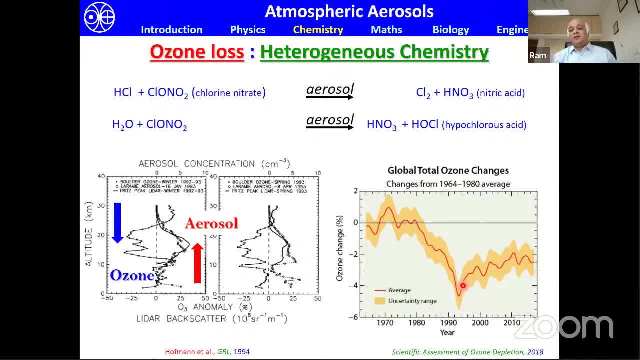 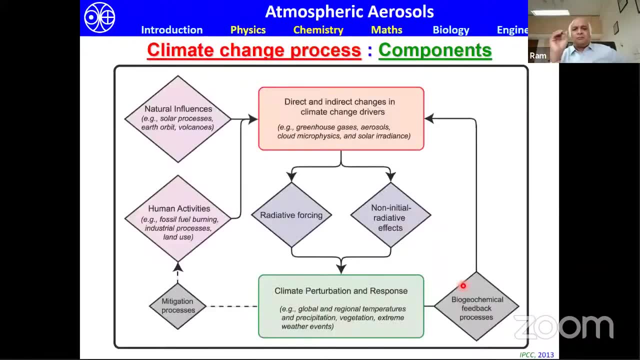 that occurred on the surface of the stratosphere was close enough in terms of total ozone change immediately after the Mount Pinatubo eruption, and this slowly started coming back to trying to come back to the position that we know. So when we say climate change process or the components that make out of it, these include 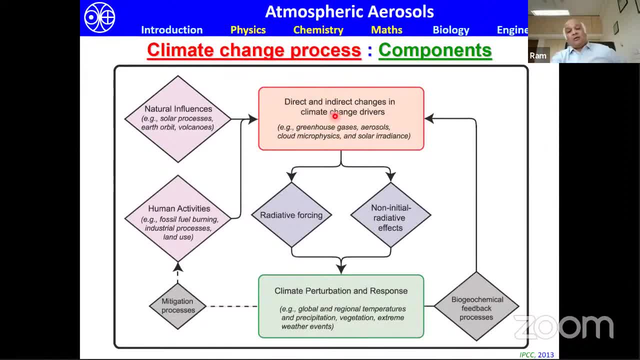 direct and indirect changes in the climate change drivers, which include the well-known greenhouse gases, aerosols, clouds, solar radiance, which contribute to radiative forcing and then through which can perturb the climate and the response, and through the human activities and also the natural influences and the variation, the biogeochemical, the chemistry, the feedback. 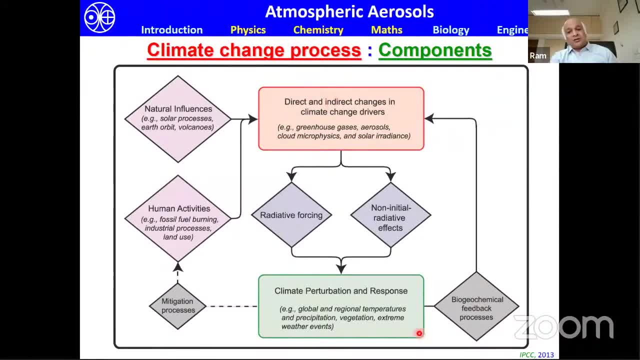 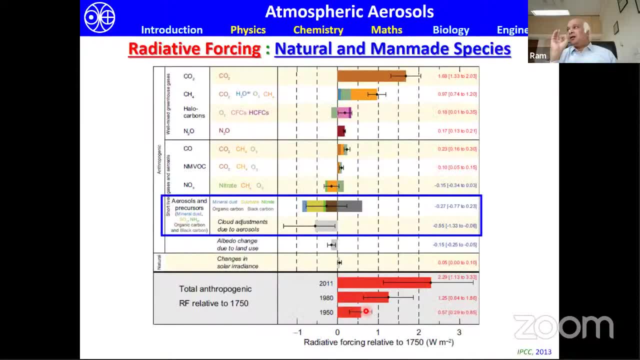 process can actually change these drivers and also can change the climate perturbation and the response. So the global climate is influenced by the agents- the following agents that are present in the Earth's atmosphere, Namely- both are natural and the human-made- the long-lived greenhouse gases versus the 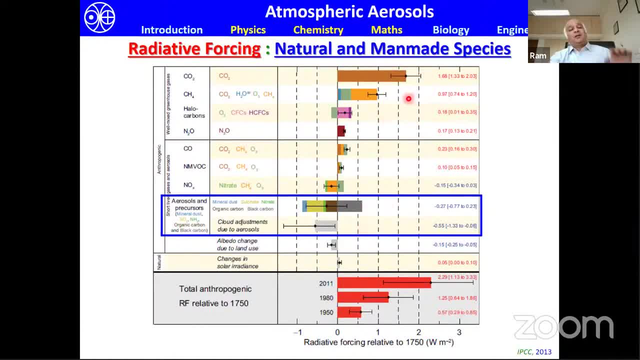 aerosols. We know that the greenhouse gas warming is a major one which is contributing to the increase in the Earth's temperature, while aerosols, which are of different kinds, as we know, can either warm the atmosphere or the surface, or cool the Earth's surface. 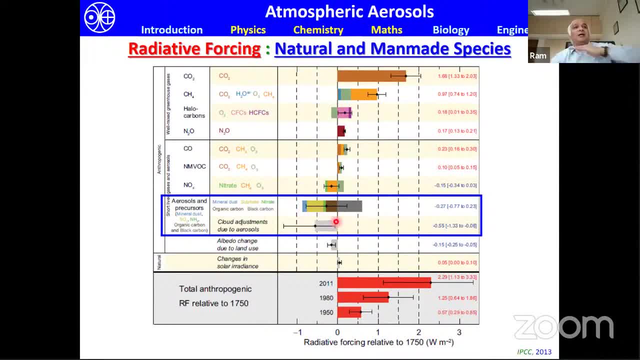 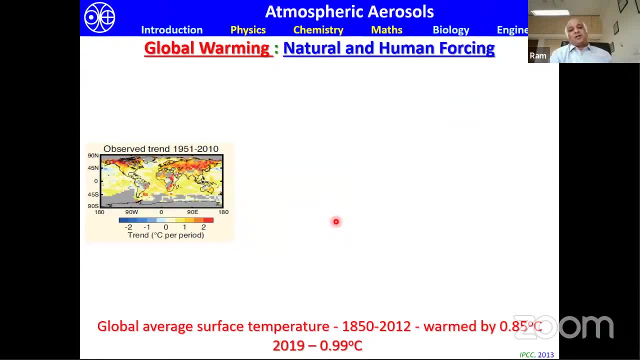 And you also see there is a large amount of error or uncertainty as far as the climate changes are concerned. So if you look at the global average surface temperature, look at the trend. for example, we are very well aware that the Earth has warmed by about in the last 100 years or 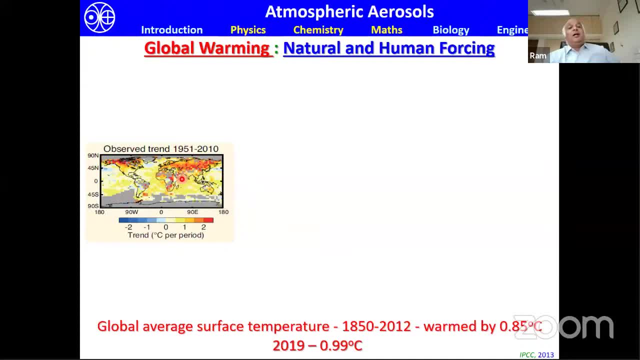 so Here we are looking at the trend per decade during the period In the last 60 years. you see everywhere an yellow or a red spot. that is So what we do is let us put the known causes of this contributing to the global climate. 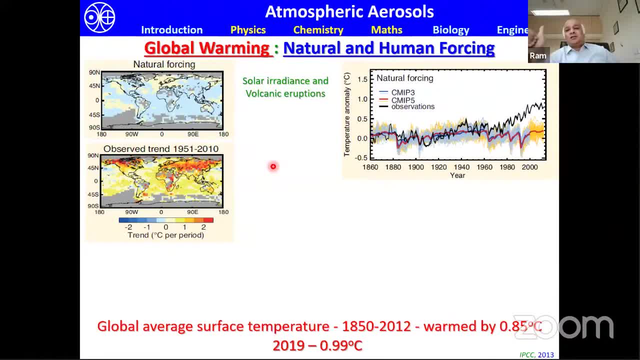 contributing to global warming or increase in temperature. So let us put the natural causes, which is, the changes in the solar irradiance and the volcanic eruption. So we know already, we have seen, that after volcanic eruption there will be the surface temperature will actually decrease with the regular time frame. 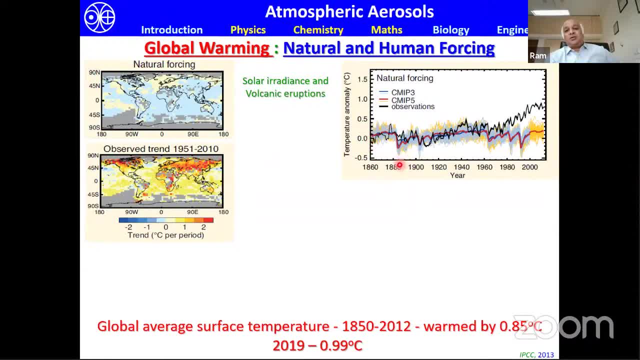 So you can see that in the last 160 years or so, after every volcanic eruption, the temperatures have decreased While the global warming is increasing. So you can see that in the last 160 years or so, after every volcanic eruption, the 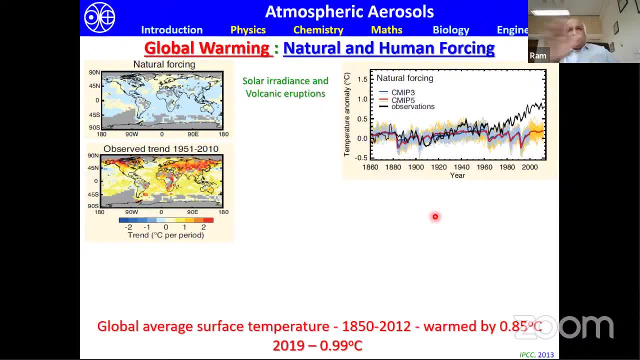 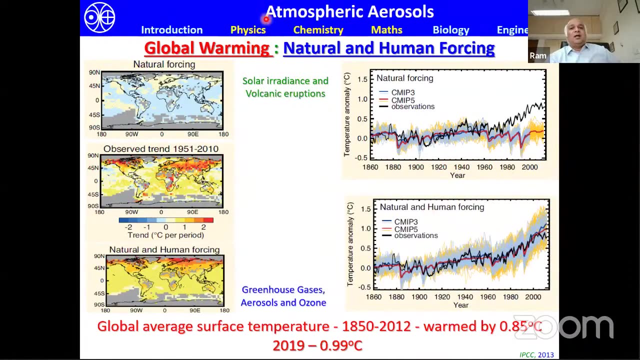 changes in the solar irradiance, which is minimal, in the last 150 years or so did not contribute to any change in the observed temperature. Then the immediate question is: come on: how is this happening Now? in addition to this, let us add the greenhouse gases, aerosols and ozone, the increases that 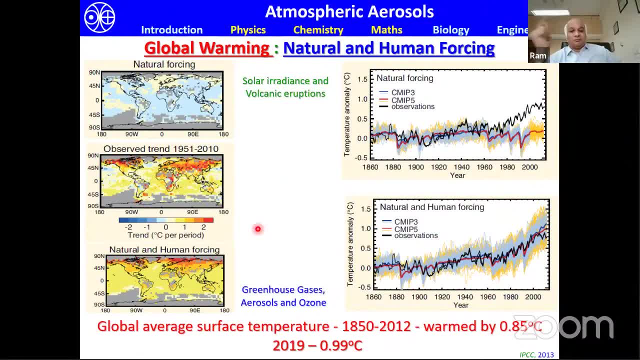 have occurred in the last 150 years. you see, bingo it happens. The model simulation. So this problem is Fermi. So it is not a point analysis because we have to think of it in detail Again. the very basic question is: can these changes in the water temperature look like? 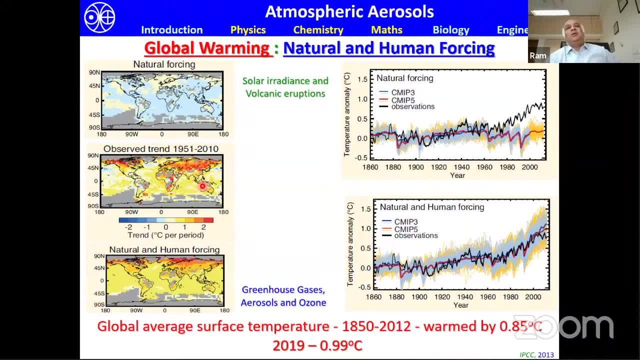 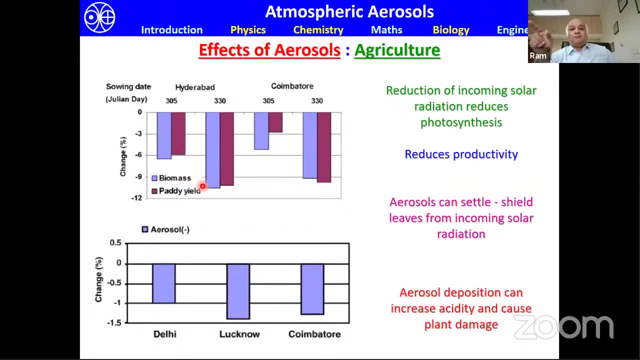 a real thing? Maybe not, honestly, I'm not sure if it's a political question. What you see here is the wind. What you see, You see trouble. You see smoke reduce the incoming solar radiation by these particles settling on the leaf. we we saw that. 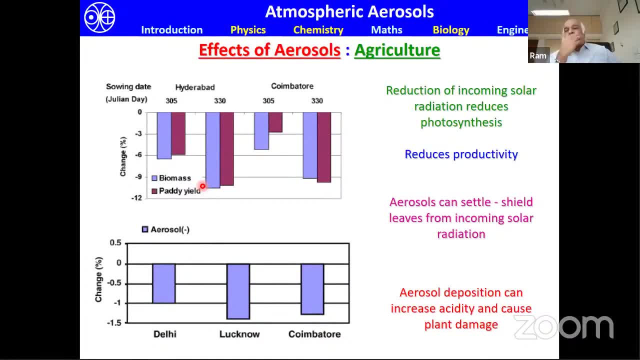 be it scattering or absorbing. they can absorb or scatter, hence any radiation that would have come in the absence of this. they get reduced, and so it can reduce the photosynthesis, can reduce the productivity so, and they can also increase acidity and cause plant damage. so modern simulations do. 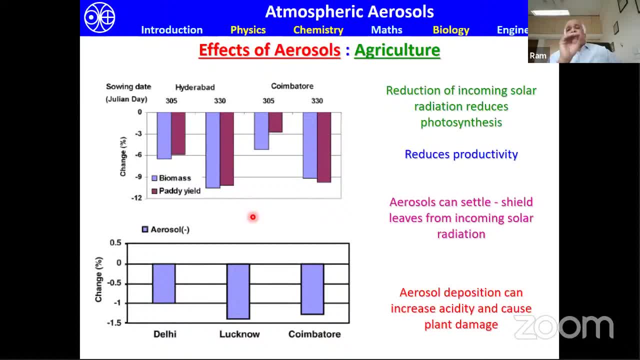 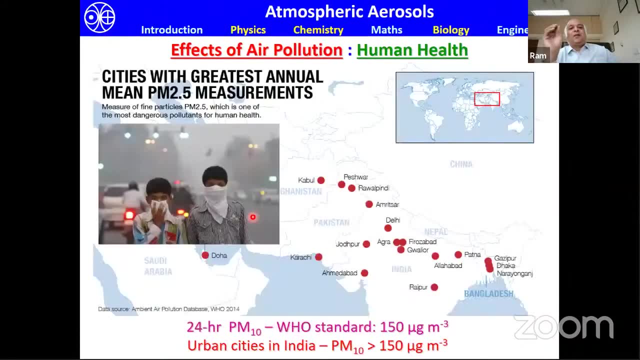 indicate that there will be a decline in the yields that will occur in the due to the presence of aerosols in the earth's atmosphere. then the other very close effect that that almost troubles everybody is the the impact on the human health. we know that typically in the polluted, when we 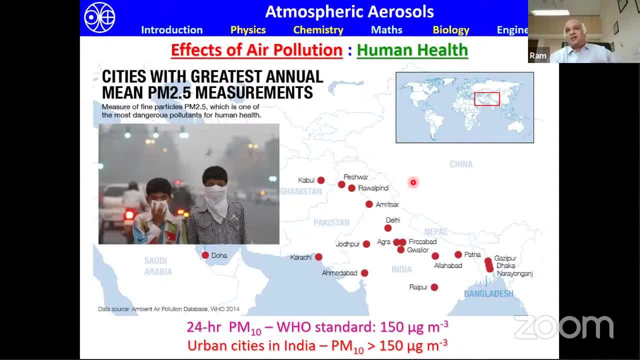 say polluted conditions, that the the sky is easy, etc. the you can see the smell, the air, as we call. so all, almost all the major metropolitan cities do have the aerosol concentration that is larger than the allowed, higher than the allowed limits because of the various activities that are there, that is present over the region, and also due to the transport of. 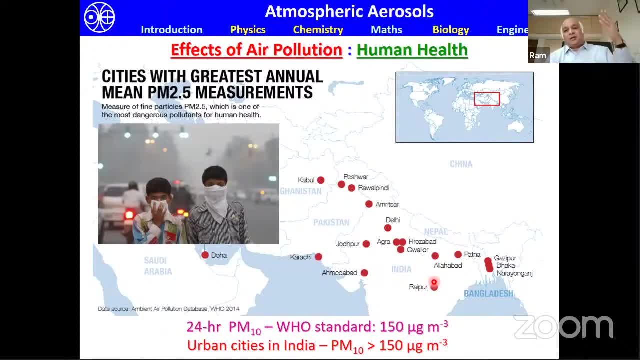 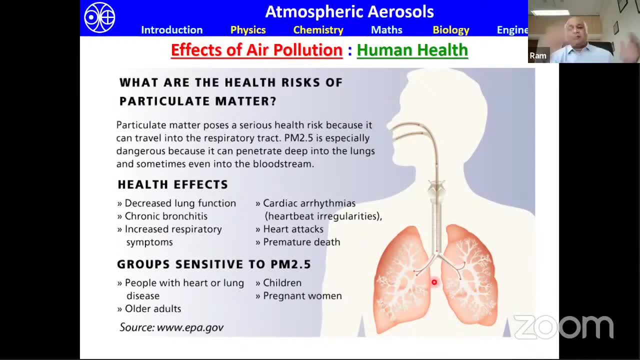 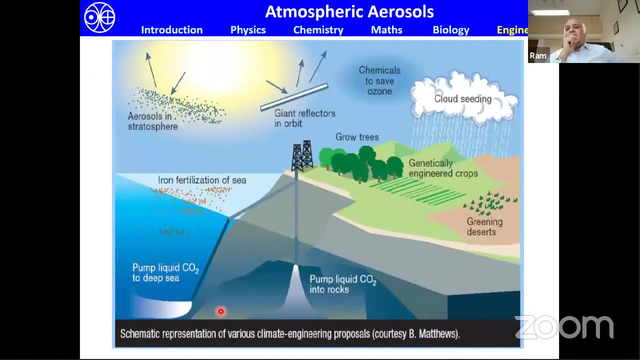 the species, depending on the dynamics, atmospheric winds, etc. so who is, what are the? what can? what? all can happen. health effects can range from, you know, decreased lung function to heart attacks, premature death, and almost everybody um under the sun will get affected because of the pollution. now, when, uh, when you 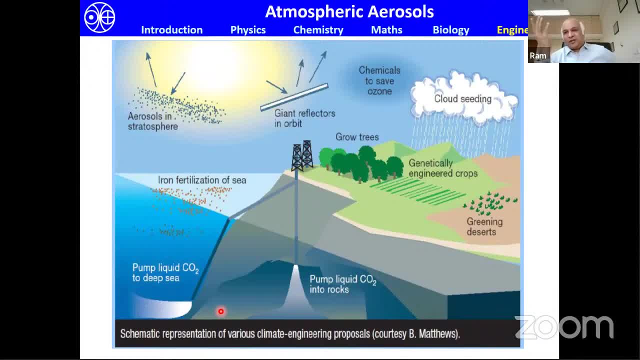 are. when we are discussing that the volcanic aerosols or stratospheric sulfate aerosols actually produce a cooling, then i am sure, uh, one of them would have thought. one of the members in the audience would have thought that, well, man, you got a solution for the global warming. what you do is 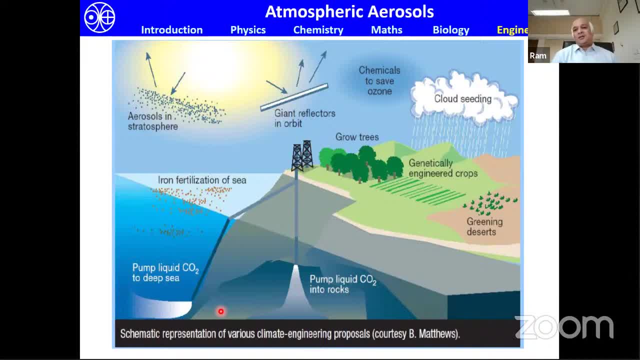 increase the input- the stratospheric sulfate aerosols or sulfate aerosols in the stratosphere- or reduce the amount of carbon dioxide in the atmosphere. so how the surface temperature will cool or the global warming will come down is because when the amount of radiation that is 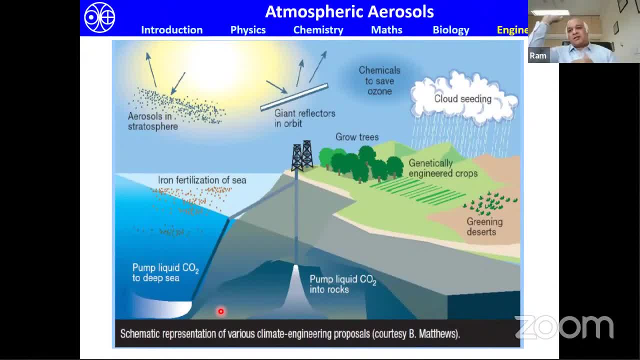 coming from the sun gets reduced because it gets reduced, because it gets reduced because it gets reflected. so it will cause the cooling or it will decrease the temperature or the amount of radiation that is absorbed with the long wave it um, it reduces, then also it will produce the cooling. 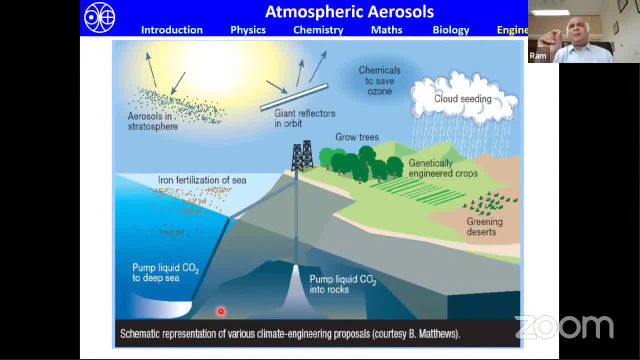 so the common uh methods or the technology where wherein we actually do what is called as the reverse engineering, is also called literally geoengineering, meaning climate intervention. you engineer the climate to, using the geological, the geography, everything, so you change the, the geo structure of the of the earth through engineering that is called as the geoengineering. 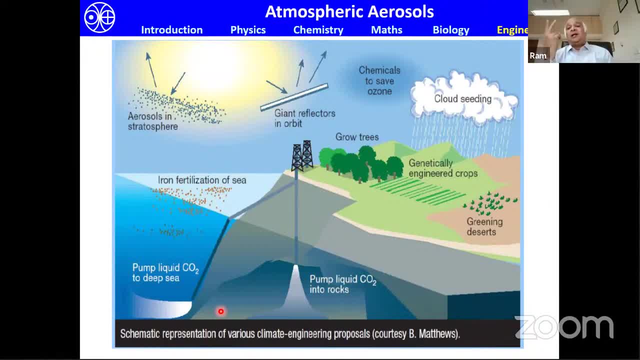 or also called climate intervention. so there are two methods with which you can achieve this. one one is the carbon dioxide reduction or removal, or the other one is through the solar radiation management. so, using space in terms of dust radiation reduction, you decrease the amount of radiation, that is. 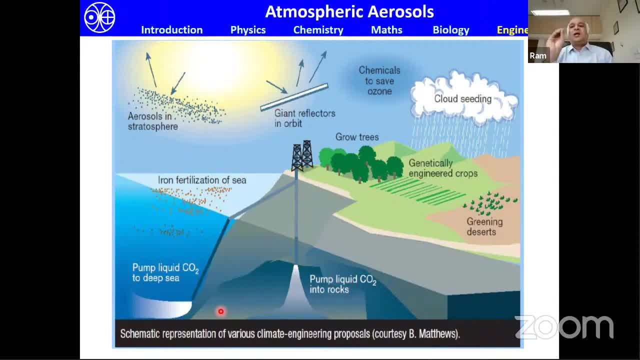 coming receiving at the earth's surface, then we know that it will produce a cooling. so let us concentrate on that by um as a topic of interest today, with aerosols in the stratosphere, uh, being input into the earth's atmosphere at regular intervals, then it will produce cooling and the 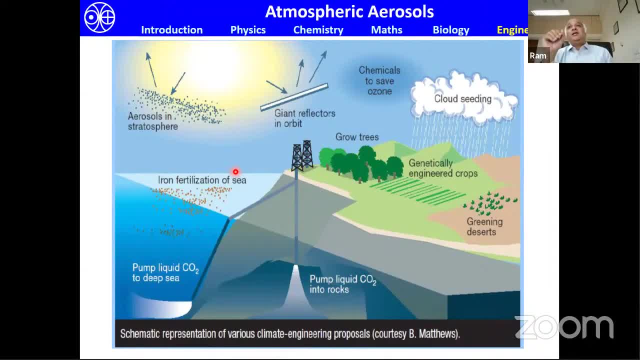 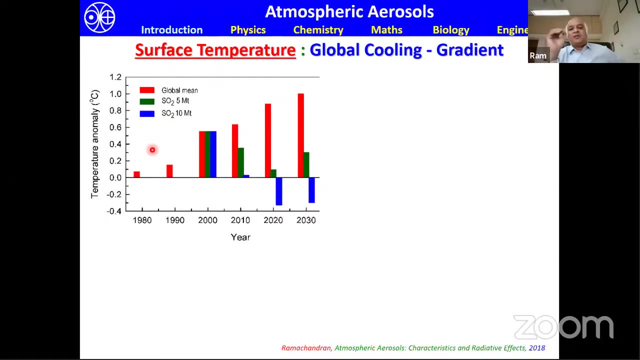 other um issues, uh issues, removal or storage. it is a long drawn process and also there are other effects and challenges. so for the time being, let us focus on the putting the sulfate aerosols into the stratosphere. so here we are looking at the temperature anomaly and then now we in the last 50 years or so, 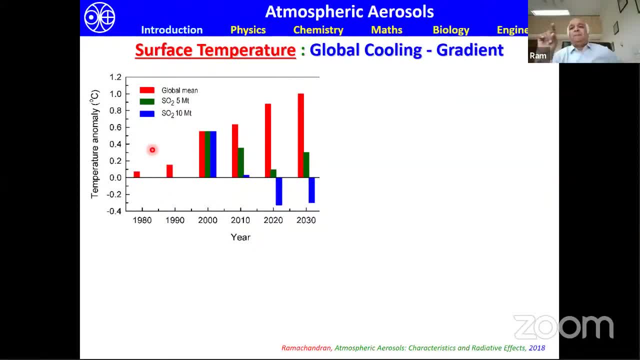 and then let us put, inject an amount of sulfur dioxide and then varied amount of sulfur dioxide. so, as you remember, i mentioned that mount pinotubo injected about an estimated 30 megatons of sulfur dioxide. so what we do is we split the amount of so2 that needs to be injected, typically at 20. 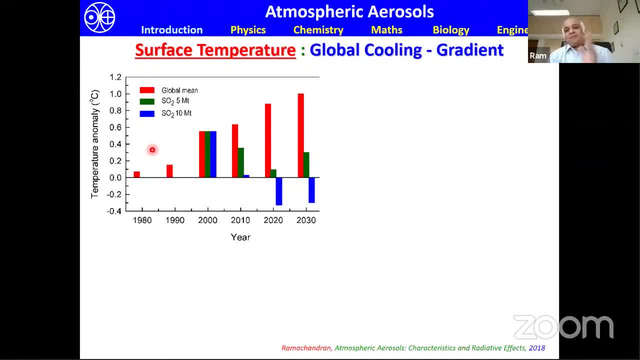 kilometer altitude, in terms of five megatons every six months versus 10 megatons of sulfur dioxide every six months or so, and then look at the possible temperature change that will occur. these are from the model simulation and the experiments. model experiments- those were. 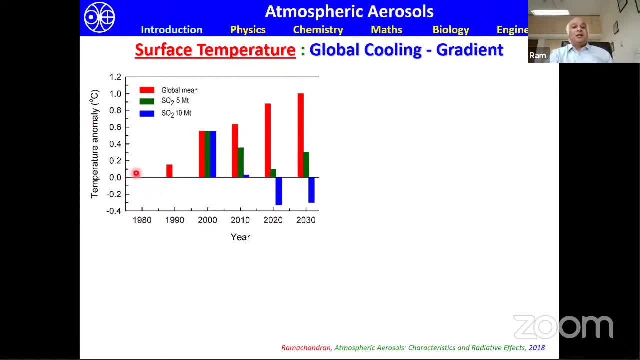 conducted. so you can see in the last: what is in red is the global mean temperature anomaly, which is steadily increasing, as we know. so we have touched almost on one degree, as i pointed out, so in 2020, for example. so now what we do is we begin this experiment in 2000. 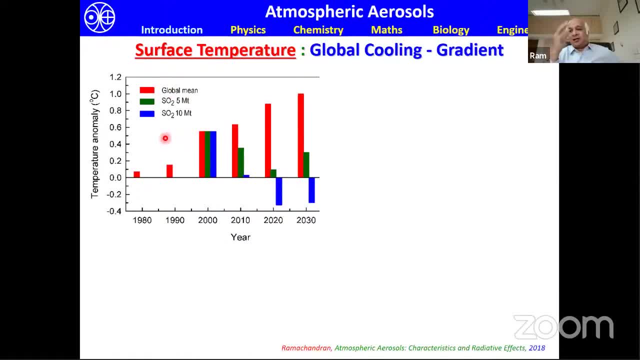 when the the we have injected five megatons of sulfur dioxide and 10 megatons of sulfur dioxide into the stratosphere, but you don't see much of a change in the initial time frame and then 10 years later. so you have to keep this injecting regularly at every six months for about five years and then. 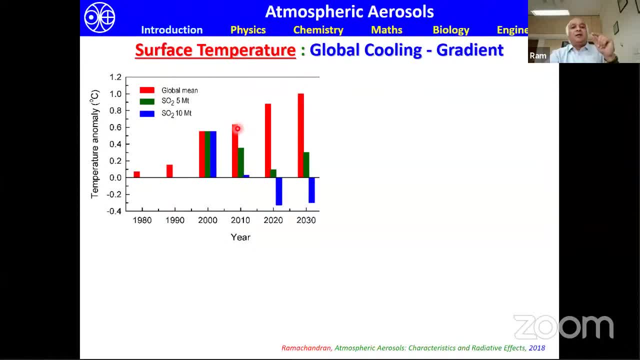 see the effect on the temperature. so you can see that when the five megatons is injected, you look at the temperature change. after about 10 years the earth's surface has cooled by about 0.5 degree centigrade and with 10 megatons it is actually almost touched to zero, meaning offsetting the 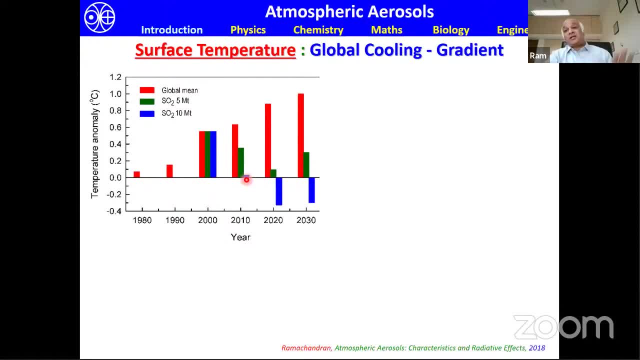 entire global warming, uh, caused by the greenhouse gases and the aerosols and ozone present in the earth's atmosphere. we still go a little further, meaning 2020 this year, for example. so with five megatons of sulfur dioxide, the temperature decreases, but with 10 megatons actually, we are even going going lower than what we are experiencing now. 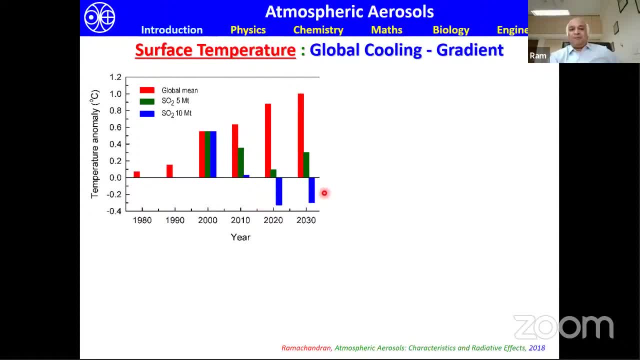 okay, and then 2030. you can see the effect that is happening. um and now let us try to see what happens if i extend this for another 10 years or so, but with the caution that i stop injecting the five megatons of sulfur dioxide and 10 megatons of sulfur dioxide into the earth's atmosphere. 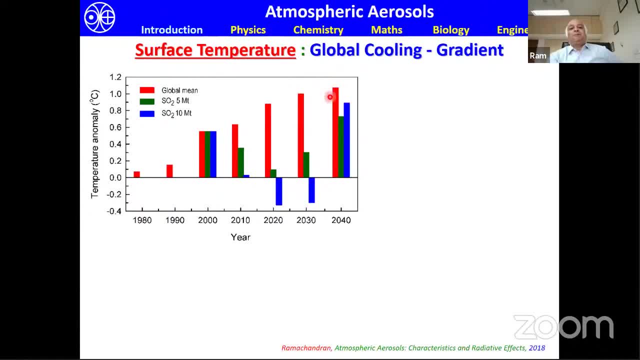 okay, i stopped from here to here. so what we see is that the- uh, the green bar also has gone up and the blue bar has gone up, which is uh, which, which is uh, which was negative in the last 10 years. you can see the gradient that is happening. so, in the last 60 years, you can see the gradient. 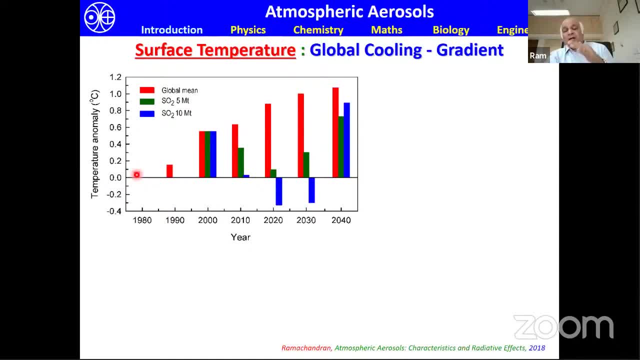 of the warming is kind of uniform and can be scaled. but Look at the. because of the geoengineering or the climate intervention that we did, putting the sulfide aerosols which can cool the Earth's surface, you can see the gradient is much faster. 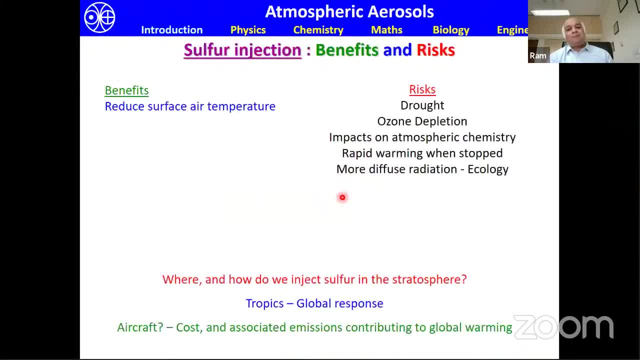 Now this has serious consequences. What are they? So the only benefit that happens is that it reduces the surface air temperature. But look at the risks, for example, Ozone depletion. we saw that it will deplete the ozone, which is equally important for the survival of the human health. 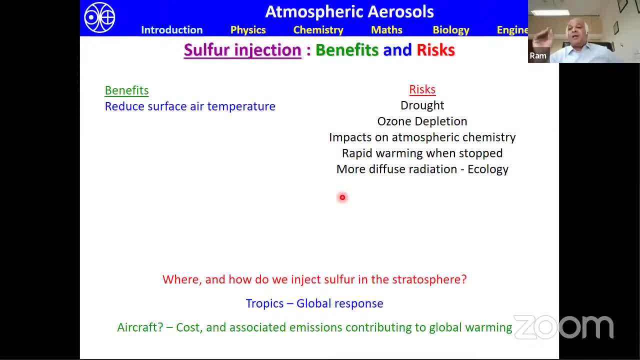 for aquatic and terrestrial ecosystems. These sulfide aerosols also will cause a drying of the atmosphere and will result in the drought condition. It will also change the composition of the Earth's atmosphere, so it will have an impact on the atmospheric chemistry, So it will warm rapidly, as we saw. 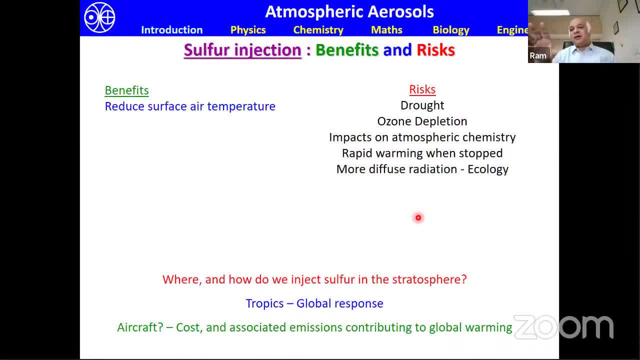 when the emissions of sulfur dioxide is stopped, And so, with more and more of these particles, more scattered or diffused radiation will increase in the Earth's atmosphere, and this will have an effect on the ecological, on the ecology. For example, we know that more diffused radiation on the leaf 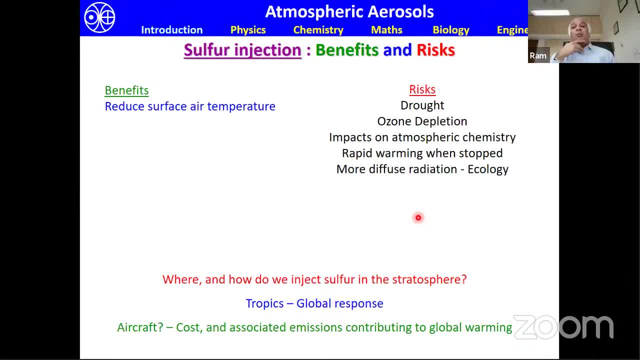 of the plant will reduce the photosynthesis. Now more logistical questions, such as- which also has economic implications and societal implications, which is where and how do we do this? How do we inject this sulfur in the stratosphere Now, for in order for the global response, global change to occur? 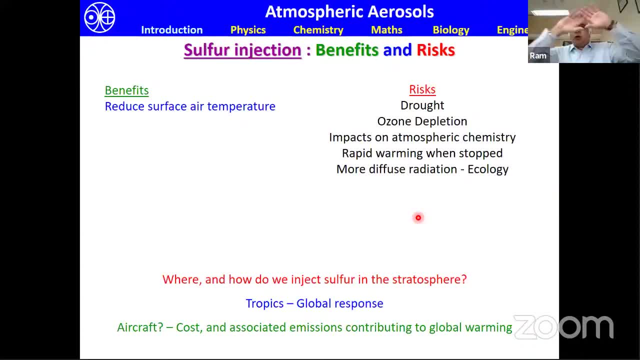 these aerosols need to be injected in the tropical belt, Then only the effects will be global, because they will diffuse across the latitude and the longitude, while injecting them at higher latitudes, namely higher latitudes, will not yield result in a global response. 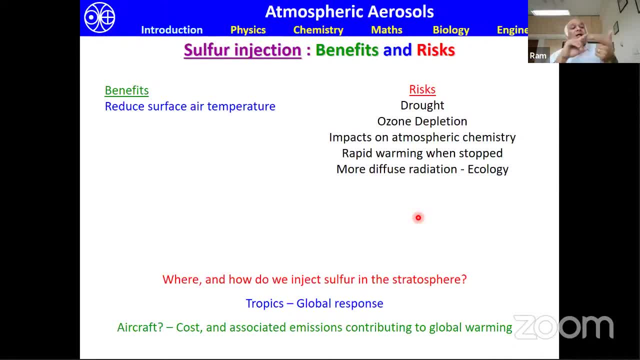 Point number one. Second thing: how do you do it? Let us say that you can use a balloon aircraft, etc. Aircraft means it has to go all the way up to 17 to 20 kilometers and then we'll inject this sulfur dioxide. 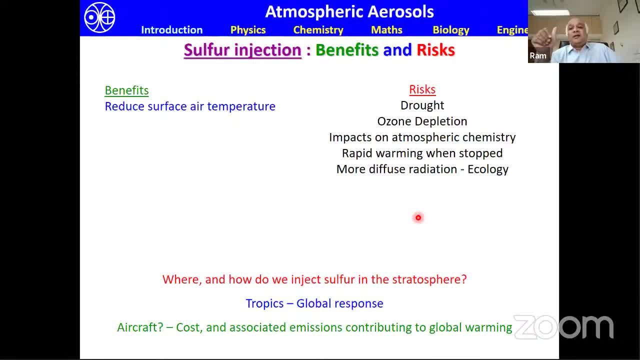 and you should do it regularly, as I said. So the question is the cost: who will bear? who will do that? And not only that: on the one hand, you are trying to control the global warming, but these emissions that are associated. 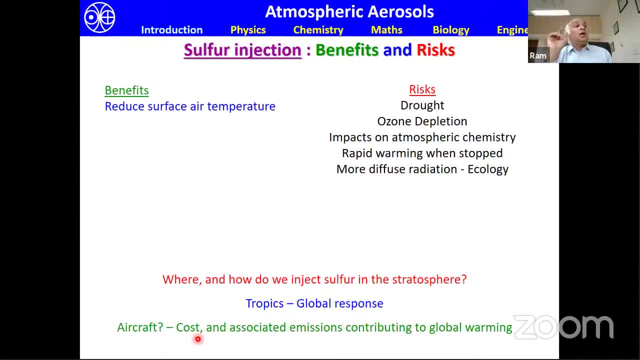 with the aircraft flying all the way up to 20 kilometers or so and transporting not one or two- 30 megatons to 5 megatons of sulfur dioxide and then going and spraying there in the tropical belt. So you are kind of intervening with the climate. 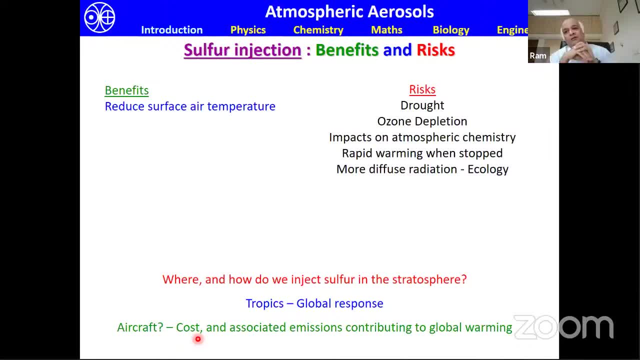 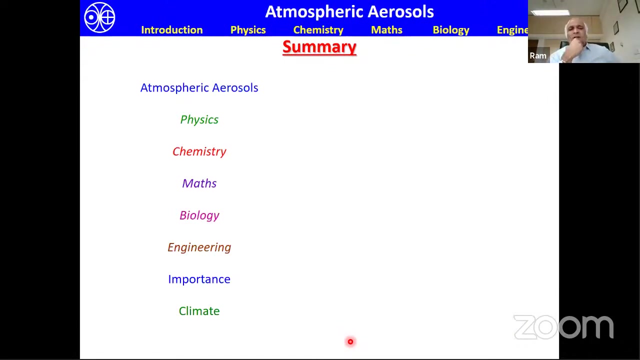 create the same scenario as a volcanic eruption would have produced or created, which means that will contribute to emissions that are already increasing. So there are more risks when compared to the benefits of this geoengineering. So I think I am finishing up with the summary. 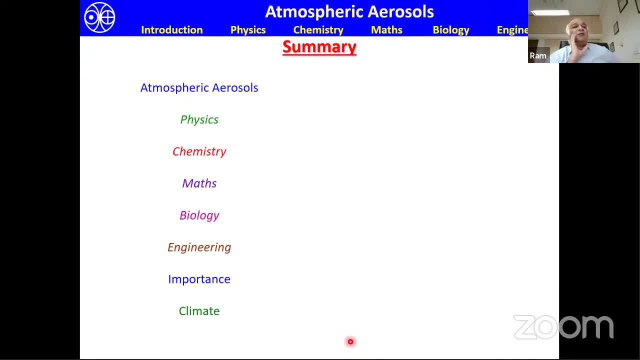 So we looked at, for example, starting from water, aerosols, the physics, chemistry, max biology and the engineering aspects of it. How do we do it? What is it we do? What is it we study? Why they are important. 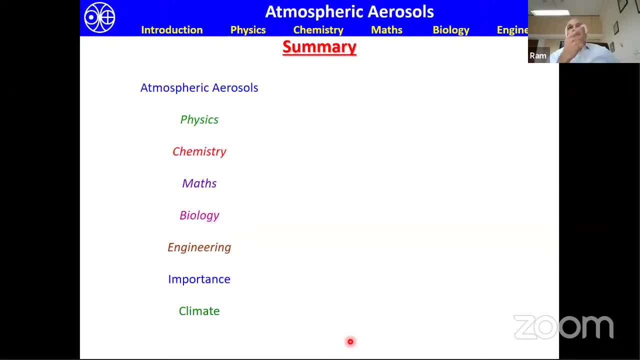 and the role they play in climate and in what way. doing anything by changing the concentration of these particles, of sulfate, sulfate particles, it will affect the Earth's temperature or, in general, the Earth radiation budget, etc. So thank you very much. 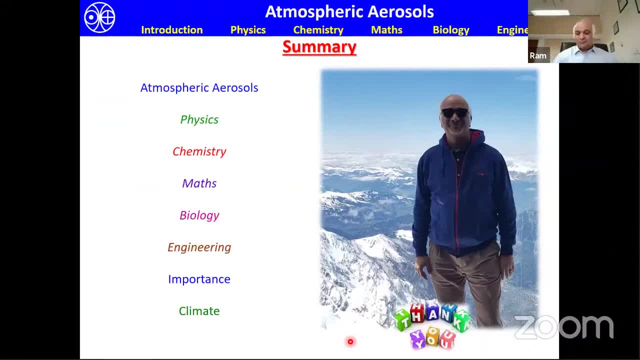 I am happy to answer the questions. Thank you very much, sir, for such a comprehensive presentation. I think you have not left anything with. you know talked about aerosols, So thank you very much, sir, for such a wonderful talk. 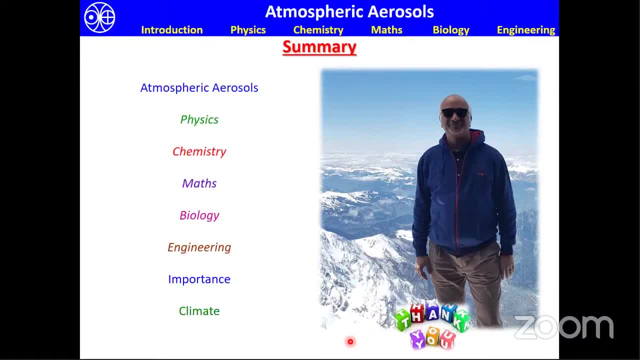 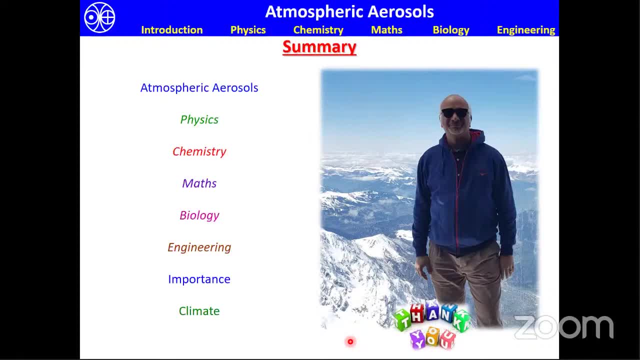 the temperature in the stratosphere increases. Why is that? Because the sulfate aerosols will absorb the outgoing longwave radiation And so, if you remember, the signal scattering albedo of any species is also a function of the wavelength In the infrared region. 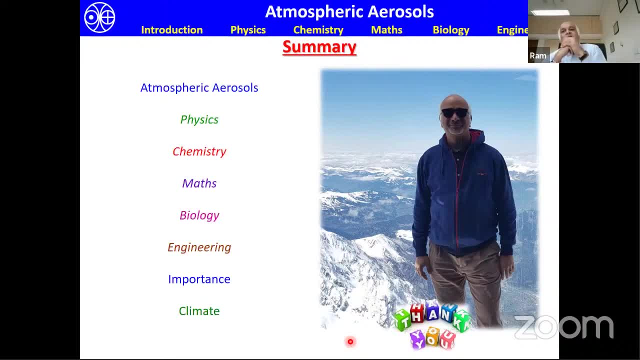 the signal scattering albedo of sulfate aerosols is lower than 0.5 or so, So they can actually absorb the radiation. So when they absorb the radiation they contribute to warming there. Sir, can they warm up even in troposphere then? 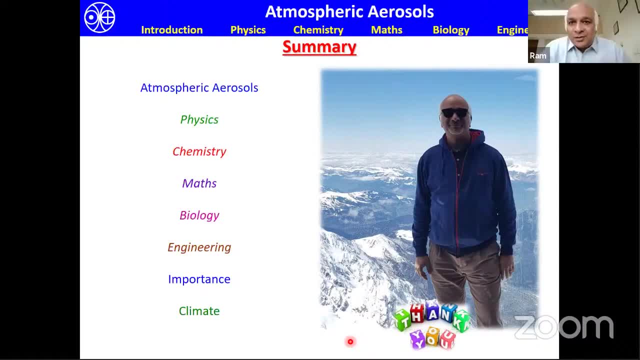 Why is it only in stratosphere? Troposphere? no Troposphere. see, as you are aware, the Earth atmosphere system is driven by the solar system. It is driven by the solar energy or the solar radiation that we receive at the Earth's surface. 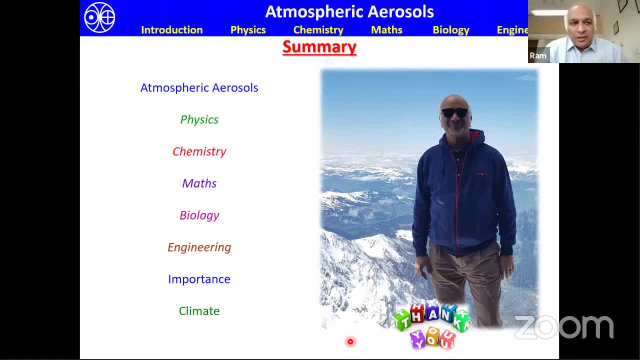 So in the Earth's surface, in the shortwave regime, sulfate aerosols are one which is of scattering kind. The signal scattering albedo is close to 1. So they can only scatter the radiation, So they will send the radiation that is received back to space. 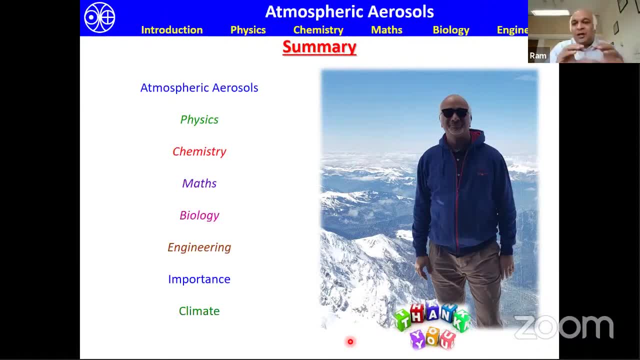 and hence they will produce a cooling at the Earth's surface. And when you increase the number of sulfate aerosols in the Earth's atmosphere, as it happens after a volcanic eruption, you are increasing the cooling. So that is why, after a volcanic eruption, 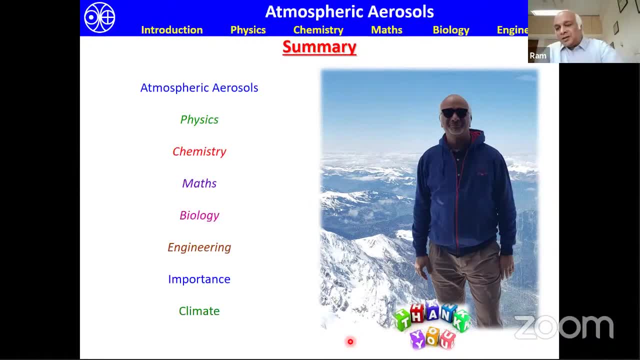 in the surface or in the troposphere. the Earth's temperature decreases about 0.2 degree centigrade on a global annual mean scale, But at the same time the stratosphere warms up by 1 degree. This cooling in the troposphere 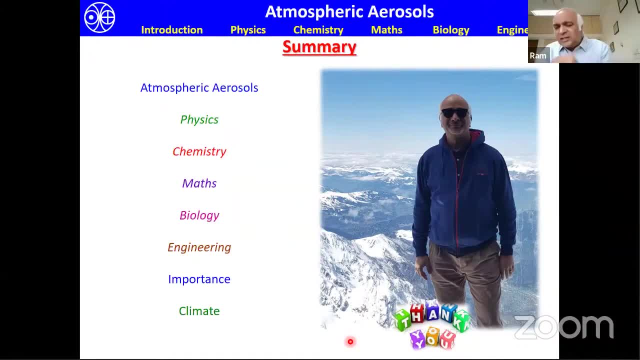 actually can vary as a function of region, latitude, longitude. Typically in the tropics the cooling is higher than about half a degree, going up to 1 degree centigrade. So if you were there, I am sure you are a 21st century kid. 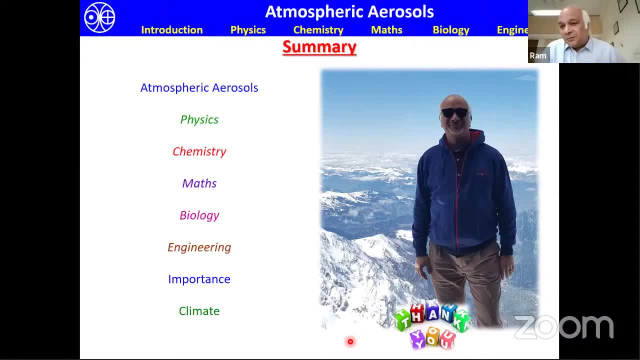 So just after, for example, the Pinatubo eruption, the winters after Mount Pinatubo, which occurred in June 1991, was a little more colder because of the decrease in the surface temperature of about half a degree over the equatorial belt. 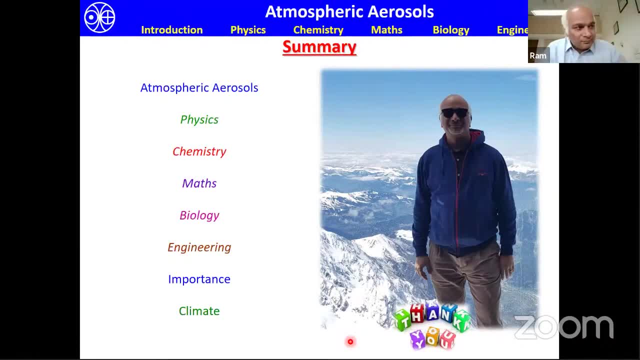 including tropics, etc. Thank you, sir, You are welcome. Sir. I have a general question. sir, Compared to the present narrative of air pollution, particularly this relating to PM 2.5, and often using that as a parameter, 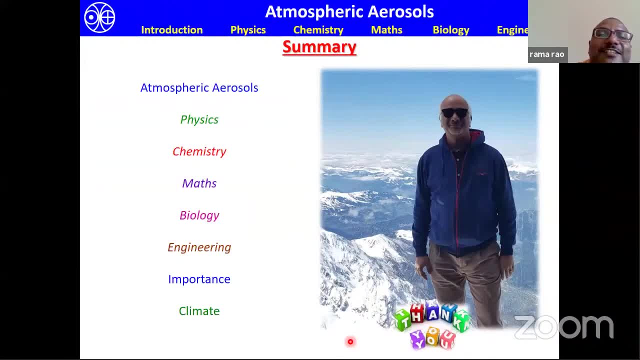 and say that that is caused by transient events such as deep valley crackers. So when we know that these aerosols are really a systematic process and also a lot of sources which are independent of an activity which happens, for example, once in a year, 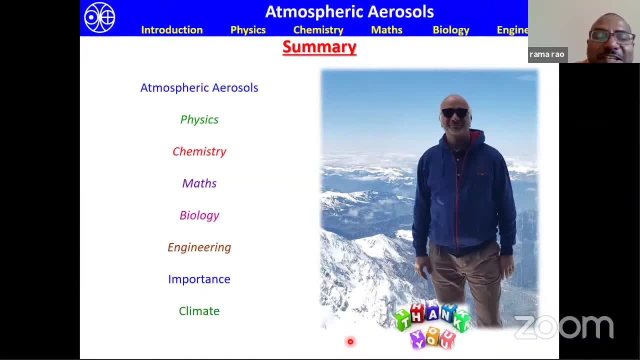 So is that really an effect, sir, compared to the many vehicular and other industrial emissions which actually do a lot of these things? Okay, Okay, Okay, See. first is, for example, over an urban region, the amount of PM 2.5 particles? 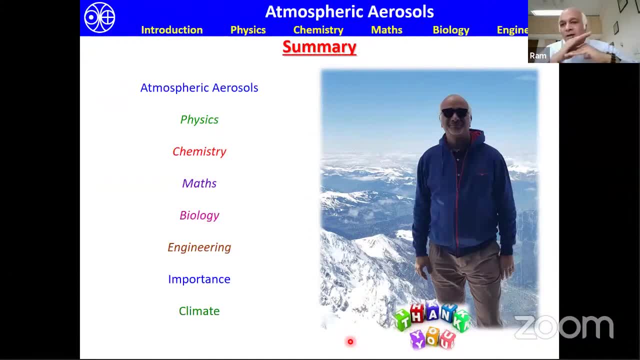 that are present due to the normal sources of vehicular and industrial emissions is already existing. Yes, Now, this level itself, if you take the annual average, this level itself is actually higher than the national prescribed standards. Yes, sir, Now during the Diwali or any other festival. 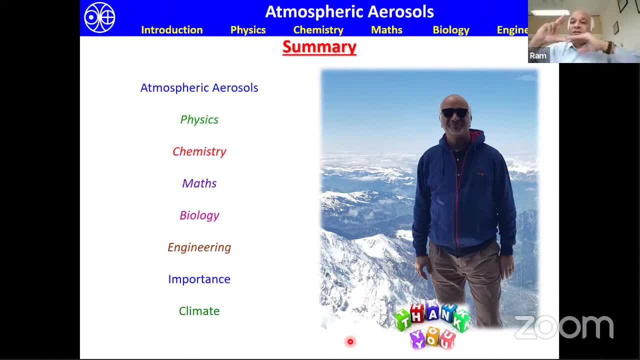 what happens is you are increasing this significantly further to the already available threshold. That is the reason. So, and since the conditions, for example, as it is happening in Delhi, for example, right now, the temperatures are so low, In fact, even in Ahmedabad. 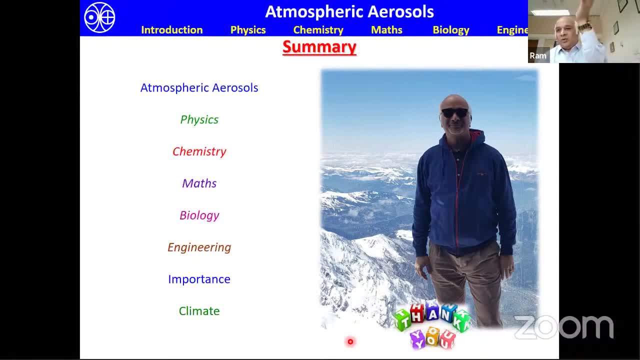 the sky is now hazy, cloudy. There is no sun at all. This is because the temperatures have become lower and these pollutants that are emitted, actually they are not ventilated out because of the lower temperature and boundary effects, So these are contained in this atmosphere. 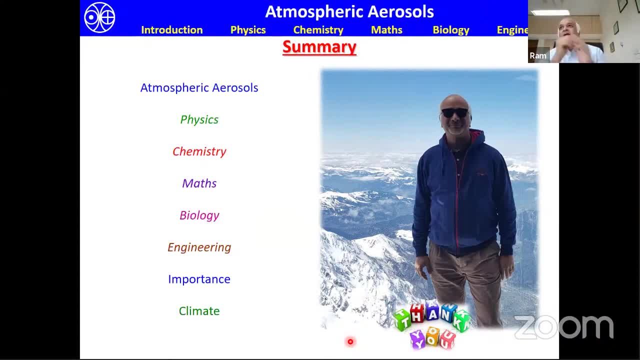 And the winds, also the wind speeds, for example. I don't see any leaves now shaking here, moving here, So the aerosols produced over this particular city or region stays in that region. So compare this with, for example: 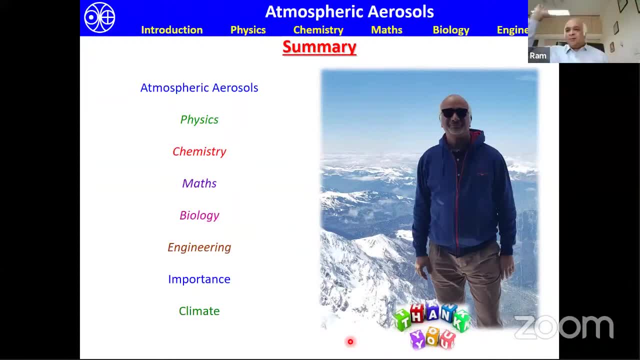 during monsoon. You may be producing it, but the winds will sweep it away, So there is a mechanism to handle them. But in this timeframe, like in winter and in post-monsoon, the prevalent atmospheric conditions actually add up to the increase. 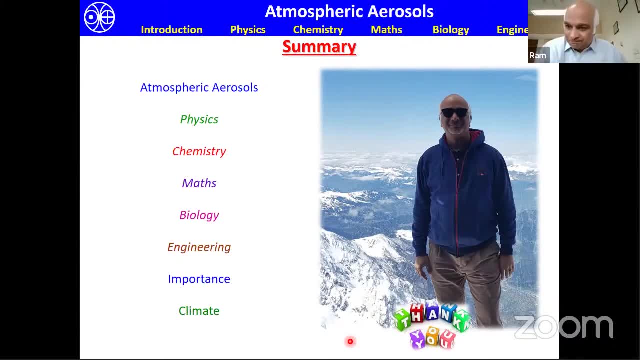 that we are contributing because of these activities. Thank you, sir. May I have another question, sir Sure go ahead- Related to retail of these AOT and kind of parameters. there are these most optical satellites and as well as this, LiDAR-based technique. 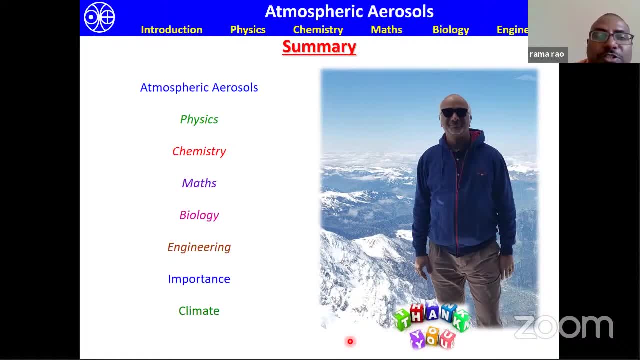 And also these days a lot of these ground-based networks, of these AOT stations, other things are there And a lot of wireless sensor networking also. So, compared to the LiDAR, is that optical technique is inferior in the way that they offer the quality. 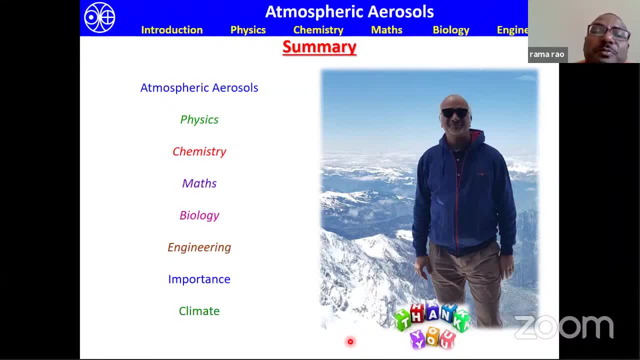 or are they better in terms of their coverage, other than Okay? First thing we should understand is that LiDAR is used to derive the vertical profile, Yes, sir, While the other ones will give you the columnar concentration. Yeah, We have, I think. 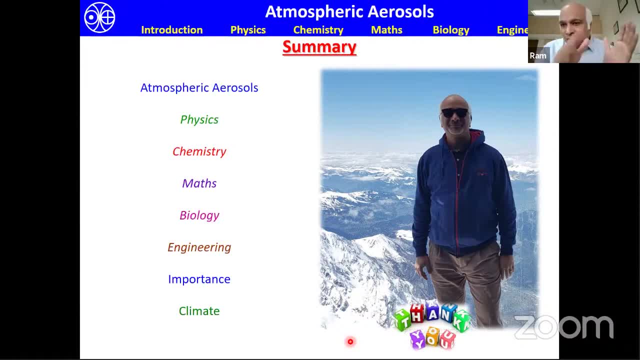 the extinction that is derived, etc. from Calypso, which is the LiDAR in space, is quite good. That is being used to study and address several research problems, Even at the ground level, when you have a LiDAR that is fixed to the ground. 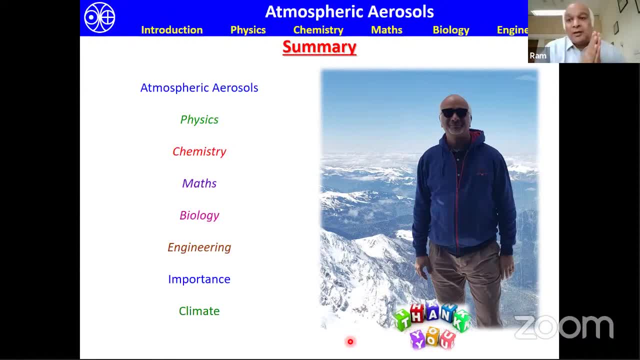 I mean the techniques, the errors, or uncertainty is actually very, very less. The one form of uncertainty creeps in when you try to derive the aerosol extinction from the total extinction, Because you need to now assume that above 40 kilometers, 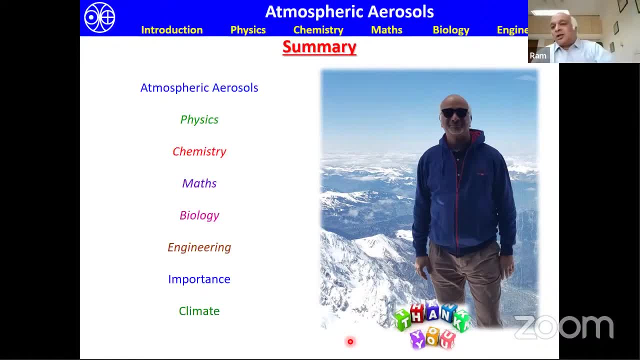 there were no aerosols or something, And then you try to derive the contribution of aerosols in the signal that you have seen. So this, for which you need what is called as a LiDAR ratio- Assumption of this actually contributes. 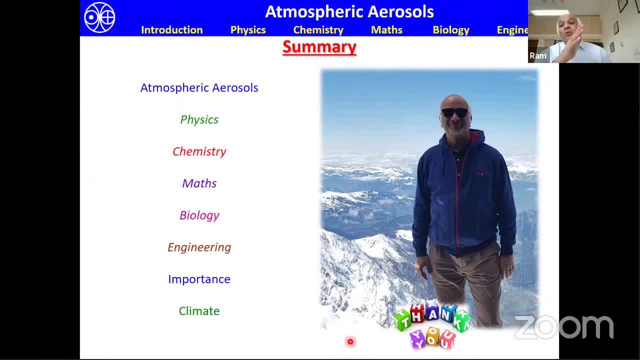 to this uncertainty in the LiDAR extinction. So what is typically done is: you can. in order to reduce this, you need to have a multi-wavelength LiDAR, So you can derive a size-dependent ratio- LiDAR ratio. 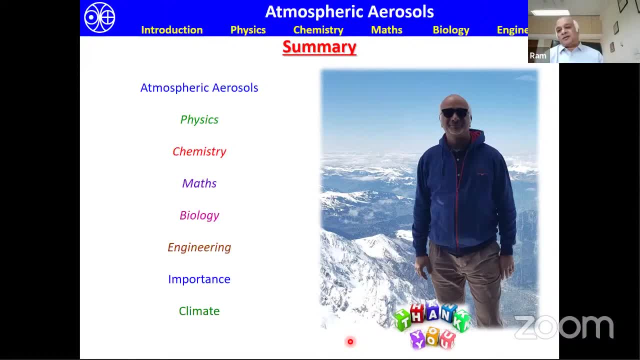 and use it for retrieval, So wherein you can reduce uncertainty. Yeah, So is that, because multiple LiDAR-based satellites are now, I think, going to come up. Is it a better progress, sir? Yeah, Of course. 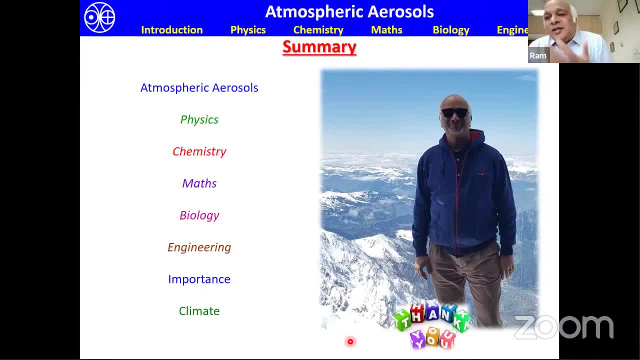 Yes, Yes, See, when you, the moment you say size distribution, say trying to identify fine versus squares, you need to have data at several wavelengths in order to derive. say this one. Thank you, sir, You're welcome. 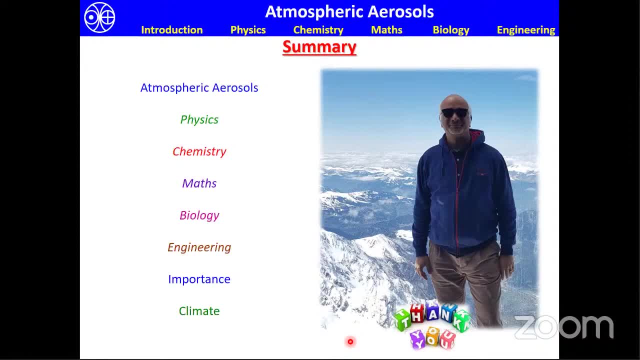 Any other question. So if you have any questions you can post to me. I can pass to Ramachandran, sir, and I think I'm sure that he will be able to give his reply to your question. So if you have any later on also, 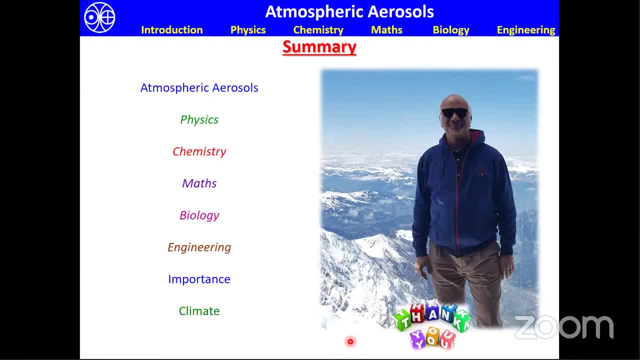 Yeah, sure, So if there is no further question, then let us thanks Professor Ramachandran for his wonderful and informative talk And thank you, sir, once again for bringing our request. Thank you for the invitation, Thank you. 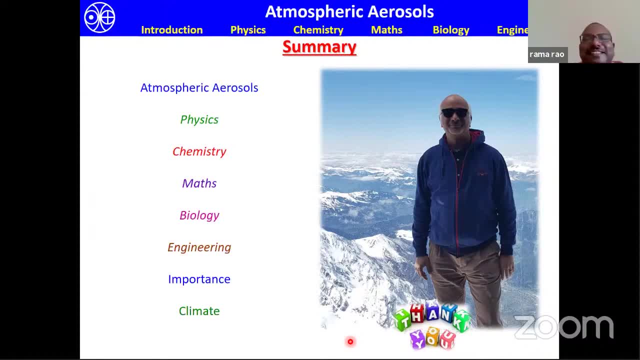